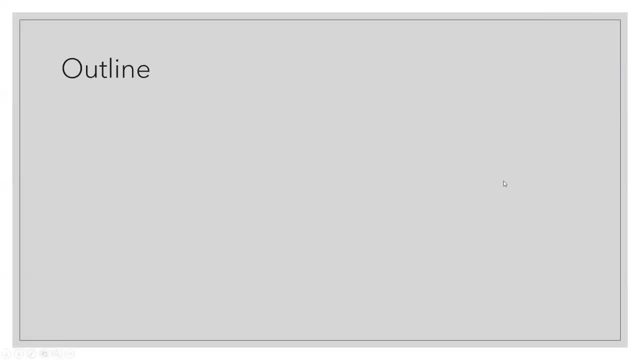 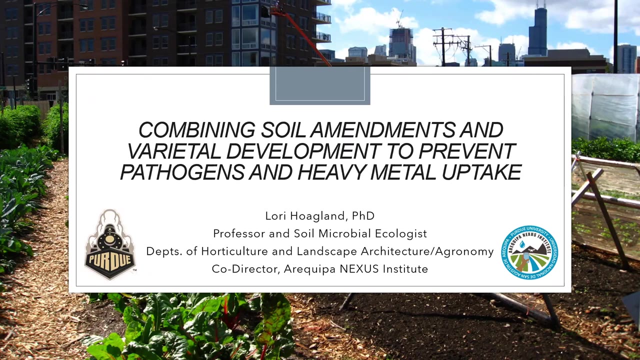 on the screen. you should be able to advance the slides. Okay, great, Okay, wonderful, All right. well, thank you, Alice, for the the opportunity for myself and my colleagues to put on this webinar series, and it's great to be a part of the webinar series. Thank you. 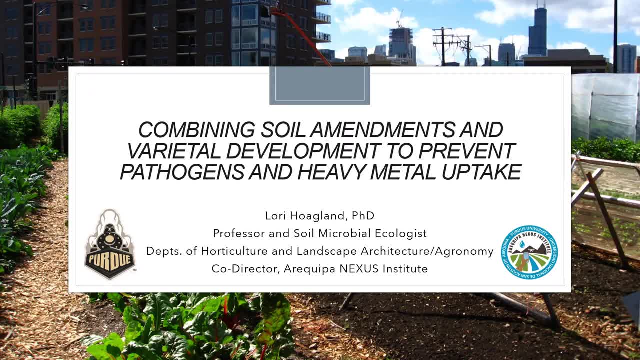 So I'd like to introduce you to some of the speakers that you're going to be talking to today. So I'm going to talk a little bit about a lot of things. So this is two aspects of my research program where, on one side, we're looking at ways to mitigate issues around heavy metal uptake and 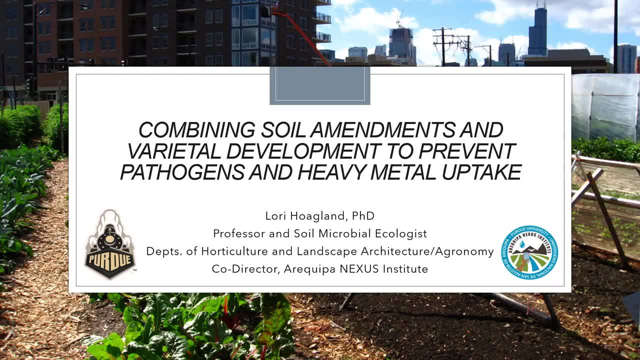 on the other side, we're working on ways to enhance biological control of pathogens, And so it's a lot to put together, and I realized that in putting this together, maybe I was a bit ambitious, but hopefully I'm going to be able to get you all involved in this. So I'm going to start with you. 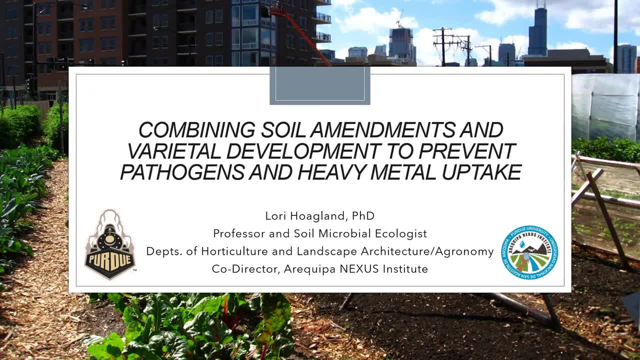 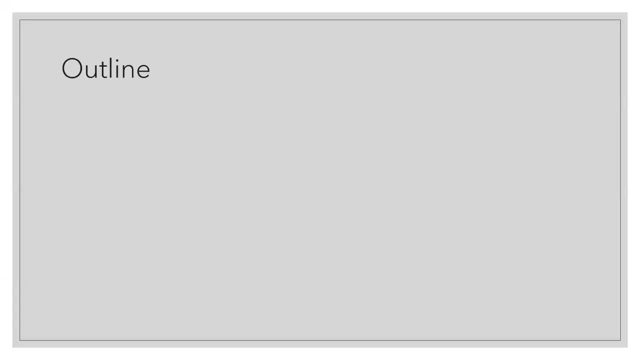 The heavy metal aspects will build on some of what you might have been hearing if you've been attending the past three webinars, and then we'll take it a little bit in a different direction with the pathogen work that we're doing. So in the talk today I'm going to start out just really giving a broad overview of some of the benefits and challenges of urban agriculture. 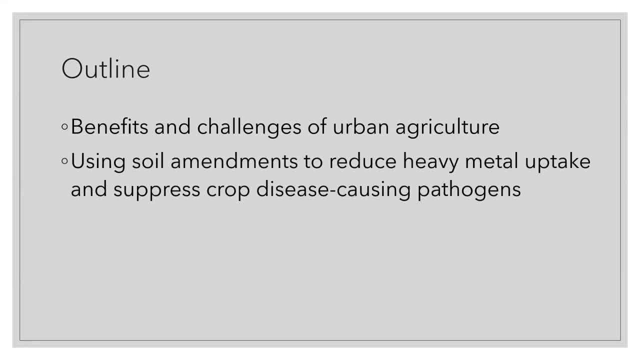 Then moving into some of the work we've been doing on investigating ways to use soil amendments both to reduce heavy metal uptake and suppress crop disease-causing pathogens. Next, we'll just briefly talk a little bit about some of the work I've been doing with the TOMI project and the CIOA project around developing and identifying varieties that can utilize multiple ways to manage crop disease. 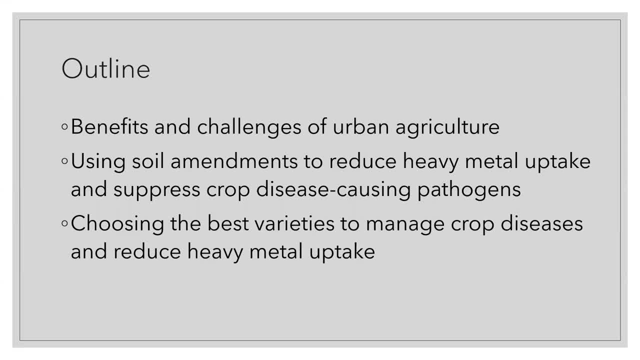 Next we'll just briefly talk a little bit about some of the work I've been doing with the TOMI project and the CIOA project around developing and identifying varieties that can utilize multiple ways to manage crop disease but also, potentially, to reduce heavy metal uptake. 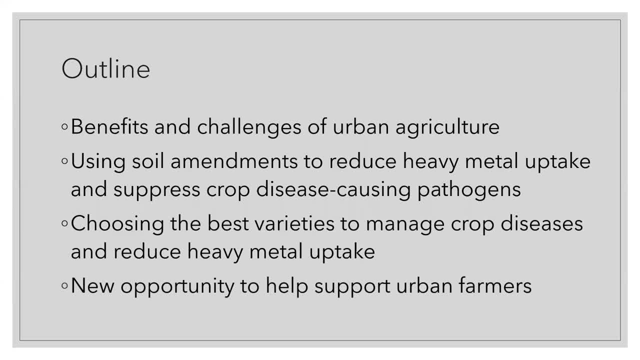 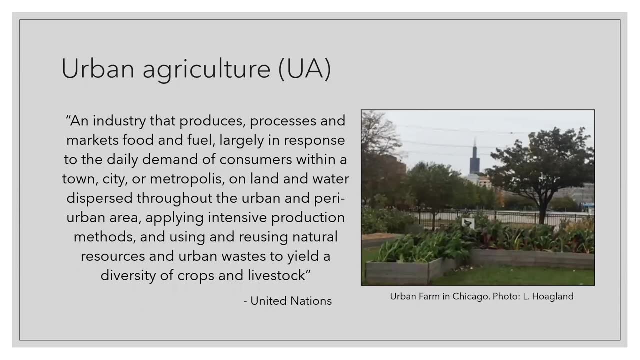 And then, lastly, I want to share with you all an opportunity that's recently arose here at Purdue University to further support urban farmers, and so I'm hoping you'll all help me get the word out about this opportunity. So first, just to start, I know we've been talking about urban ag- This is the fourth in the series now- but in case you're just joining us and you're not familiar with 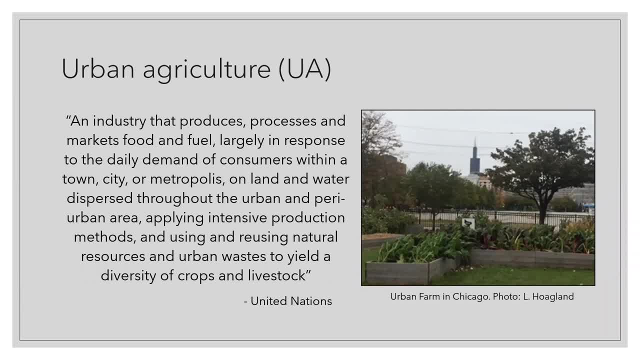 What urban agriculture is? there's lots of ways to define it, but I like this particular definition from the United Nations that just describes urban ag as this: an industry that produces, markets, Food and fuel, largely in response to daily demands of consumers within cities or around cities, generally applying very intensive production methods and using and reusing natural resources and urban waste. 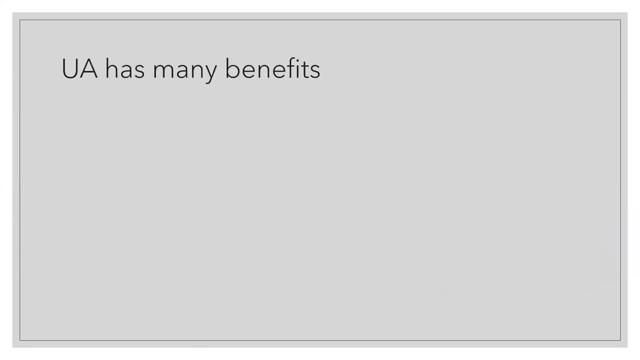 To To help the yield crops and livestock. So there's many different benefits of urban agriculture and I'm not going to talk about all of them, but just some of the ones that come to mind that I like to talk about in my class. 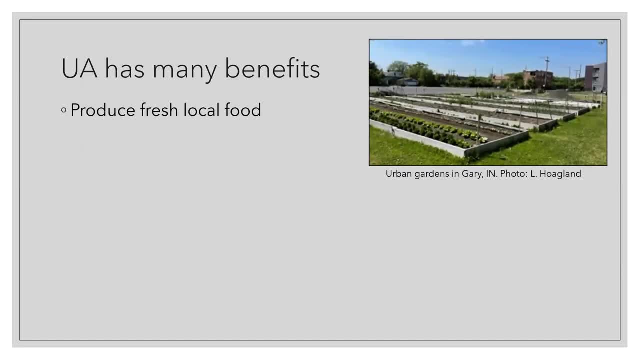 First of all, just the capacity to produce fresh local foods, like this wonderful garden up at Gary and Deanna Sojourner's Truth House that does a great job In creating produce for their local Neighborhood. It can help to improve human nutrition. We know that when there's greater availability of fresh produce, people tend to eat more of that produce and so therefore improving human health. 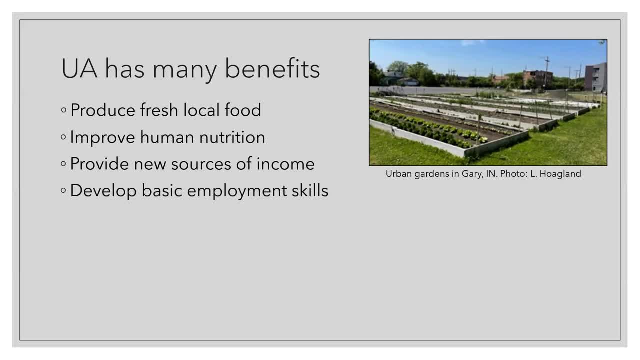 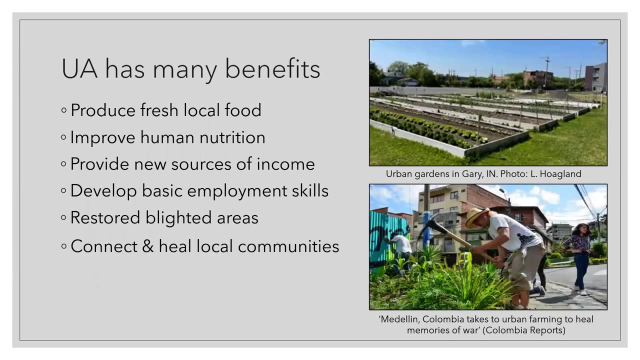 can provide new sources of income for local communities, help to develop basic employment skills and also restore blighted areas within a local neighborhood. There's also plenty of social benefits, Things like bringing communities together to connect and heal after turbulent periods like here. I love this article about Medellin: how they're using urban AG to heal memories of war there. 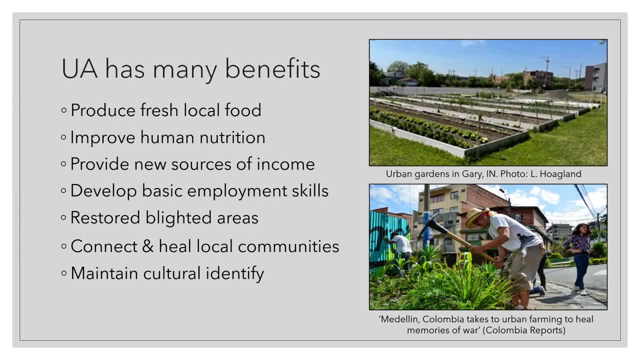 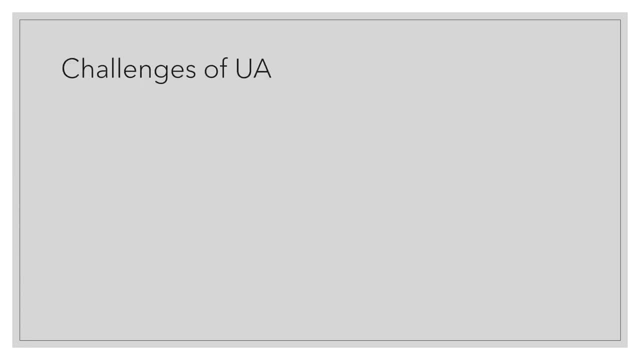 And it can help to maintain cultural identity. as people move into new cities, they can grow crops that they're familiar with. So, unfortunately, there's also several challenges associated with urban agriculture. So, unfortunately, there's also several challenges associated with urban agriculture. So, unfortunately, there's also several challenges associated with urban agriculture, And the one that we've been talking about a lot within this series is that soils, unfortunately in many urban areas can be very highly degraded and, in some cases, contaminated with toxic heavy metals and metalloids- mostly things like lead, cadmium and arsenic. And the one that we've been talking about a lot within this series, is that soils, unfortunately, in many urban areas can be very highly degraded and, in some cases, contaminated with toxic heavy metals and metalloids, mostly things like lead, cadmium and arsenic. And the one that we've been talking about a lot within this series, is that soils, unfortunately, in many urban areas can be very highly degraded and, in some cases, contaminated with toxic heavy metals and metalloids, mostly things like lead, cadmium and arsenic. And the one that we've been talking about a lot within this series, is that soils, unfortunately, in many urban areas can be very highly degraded and, in some cases, contaminated with toxic heavy metals and metalloids, mostly things like lead, cadmium and arsenic. And the one that we've been talking about a lot within this series, is that soils, unfortunately, in many urban areas can be very highly degraded and, in some cases, contaminated with toxic heavy metals and metalloids, mostly things like lead, cadmium and arsenic. And the one that we've been talking about a lot within this series, is that soils, unfortunately, in many urban areas can be very highly degraded and, in some cases, contaminated with toxic heavy metals and metalloids, mostly things like lead, cadmium and arsenic. 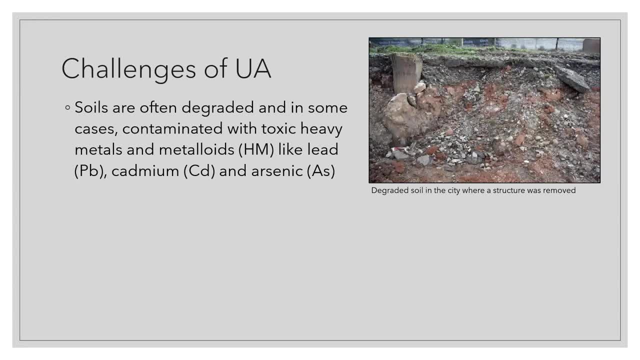 And the one that we've been talking about a lot within this series, is that soils, unfortunately, in many urban areas can be very highly degraded and, in some cases, contaminated with toxic heavy metals and metalloids, mostly things like lead, cadmium and arsenic. 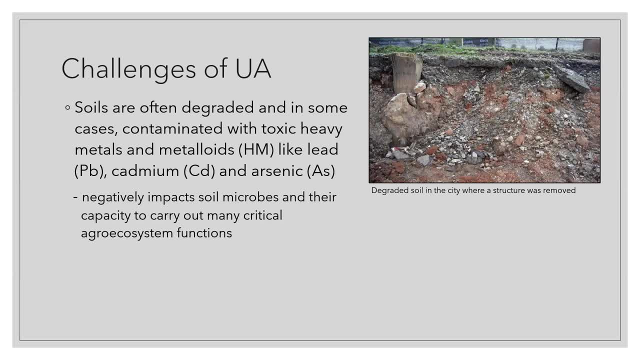 So this contamination- and both this degradation- negatively impacts the capacity for soil microbes to carry out many critical agro ecosystem functions like nutrient cycling or carbon sequestration. This can also alter plant metabolism and potentially make plants more susceptible to biotic stress, like pathogens, as well as abiotic stress, things like heat and water. 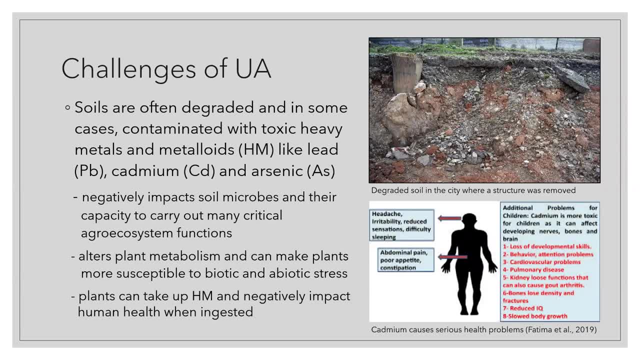 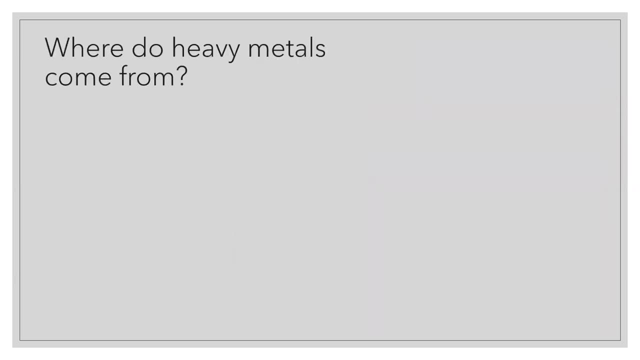 And then, worst of all, if there is contamination presence, plants can take up some of these heavy metals and this can negatively impact human health, especially young children, when this produce- contaminated produce- is ingested. So where do heavy metals come from? There's a variety of sources. 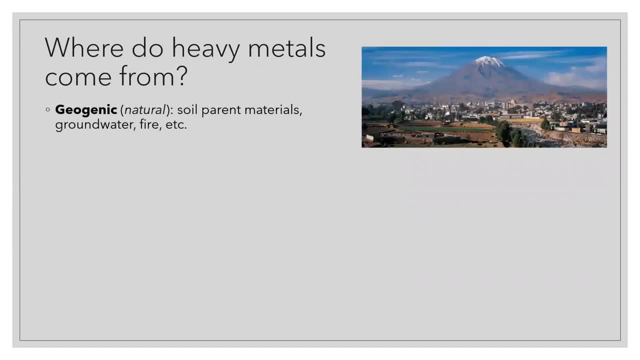 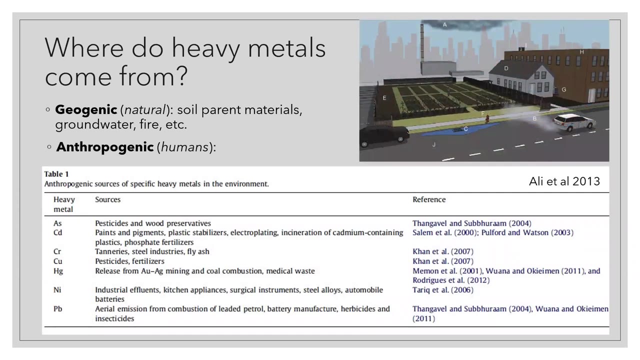 This can be geogenic. natural soil, parent materials and volcanic regions, for example, may have greater deposits of heavy metals. There can be things like groundwater fire that contribute it, But mostly here in our northern cities a lot of the contamination could be due to more anthropogenic factors. 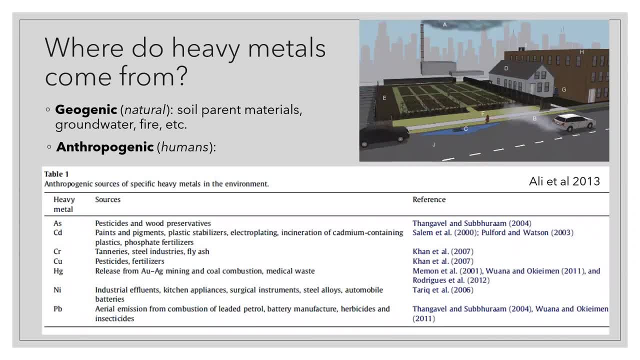 such as things like wind. we use leaded gasoline for years in our cities- and leaded paints. There are also pesticides and fertilizers that can contribute to heavy metals, And so this can potentially be problematic in some areas of urban urban areas. So another challenge is just there's a lot of pests. 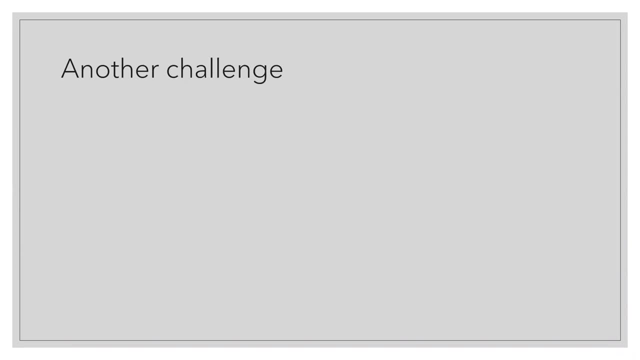 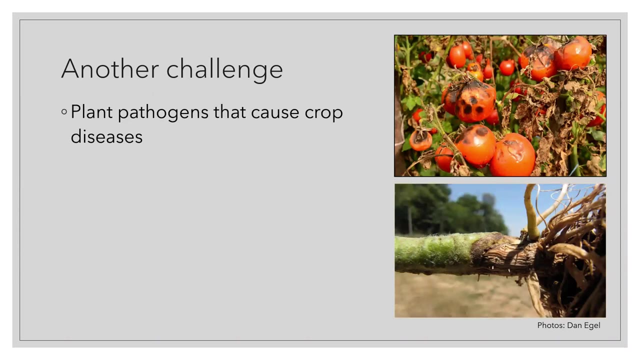 So if you work in agriculture you know you hear about these things all the time. but they're also a problem in cities And in my lab the pests that we find we focus on a lot because our surveys have indicated are very problematic. 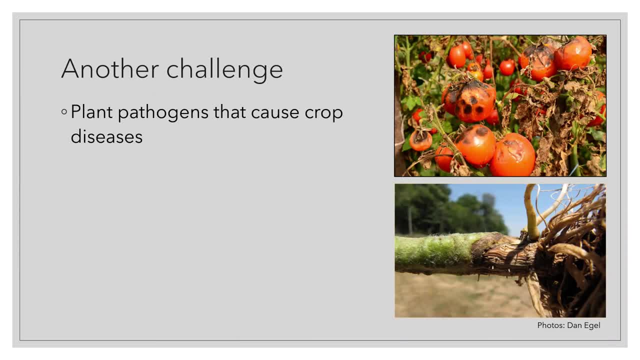 Our plant pathogens like these that can cause crop diseases. So out here in the Midwest, where I'm at, there's a lot of these pathogens can be favored and very warm, wet and humid climates like we have, We know these can pretty dramatically lower the yield and quality of produce, as well as increased production costs when you have to be replanting. 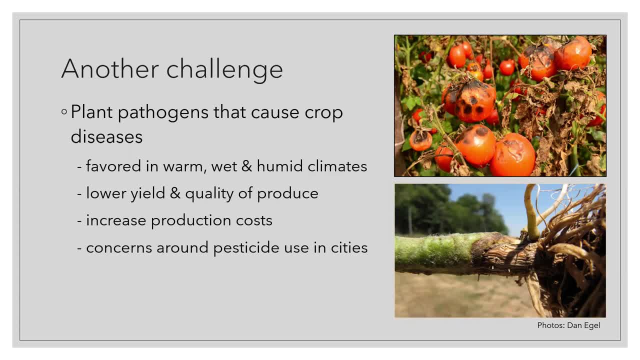 lowering your yield And, while you know, controlling pests is a problem and pathogens anywhere, it can be particularly problematic in cities because using pesticides, there are issues around that with spread and legal things like that- People might not have the training to use them. 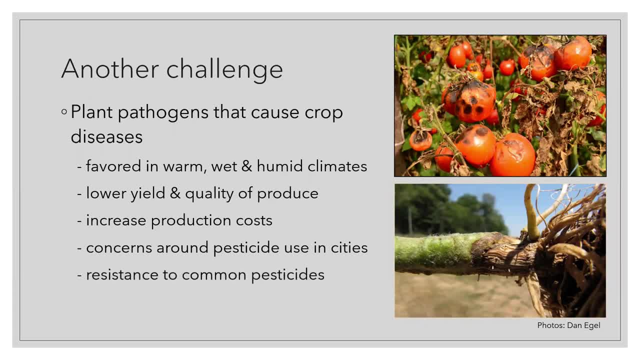 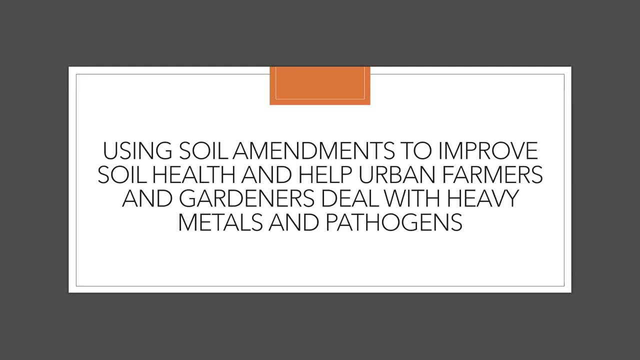 And then we know many of the pesticides out there, even copper products- that are used, often in organic systems. a lot of pathogens are developing results, So there's a lot of resistance to those. So we need alternatives. So now I'm going to move into some of the work that we've been doing over the past many years. 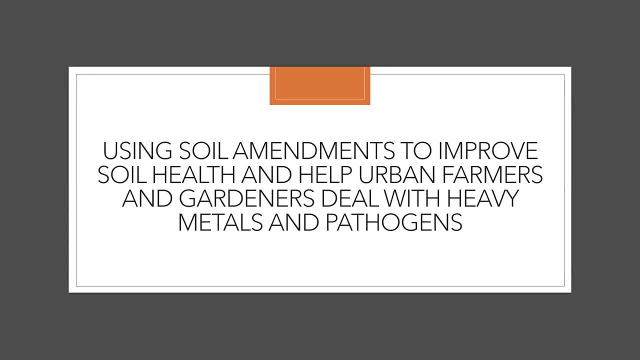 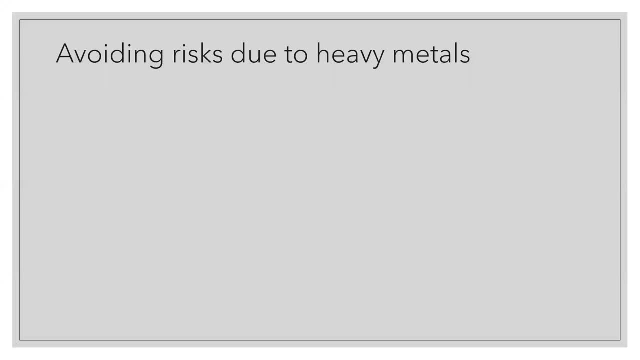 using soil, amendments to improve soil health and potentially help urban and peri-urban farmers and gardeners deal with these two challenges that can be related in many cases. So first of all, before we get into soils, I just want to recap. I suspect this has been said in the other seminars. 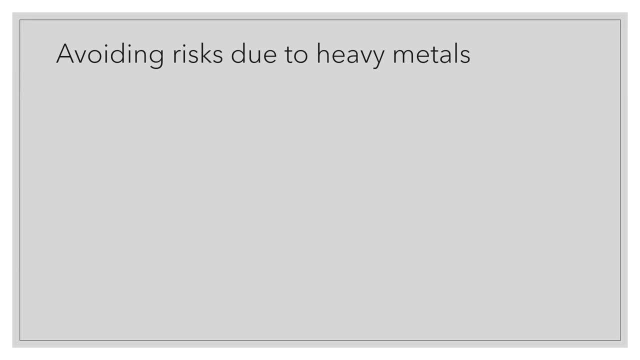 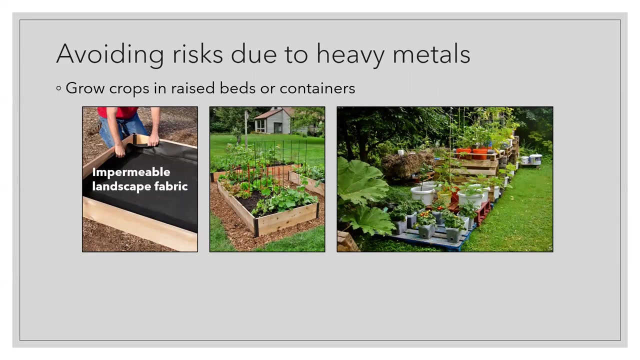 but it's just good to focus on things that we know we can do to really reduce risks around heavy metals, especially if you're in an area that has pretty high concentrations in your soils And so one you know pretty easy thing to do is just to grow crops in raised beds or containers to physically remove them and keep them separated from contaminated soils. 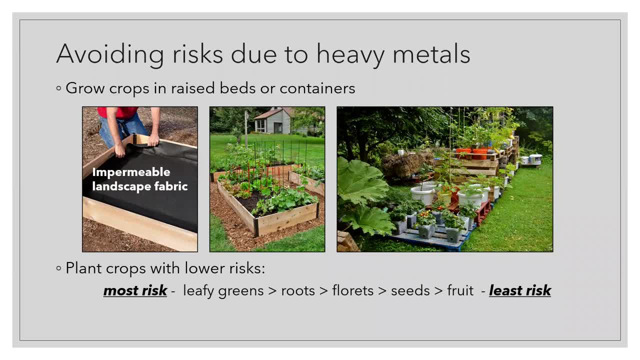 You can also plant crops with lower risks. So this is just kind of a standard you know thing of what we see in terms of risk associated with heavy metal uptake. Leafy greens tend to be the most problematic, Some root crops and then generally fruit. 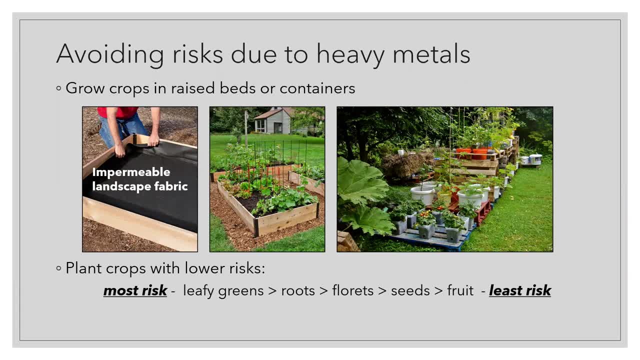 fruiting crops are a little bit safer because they tend to accumulate less heavy metals in fruiting tissues. And lastly, regardless of how you're producing food, you should always look at thoroughly washing all of your crops to remove soils and peeling root crops. 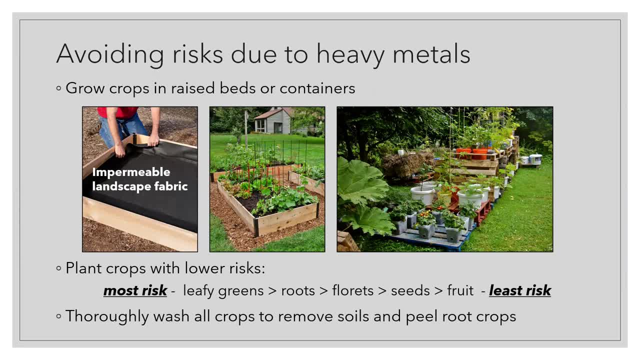 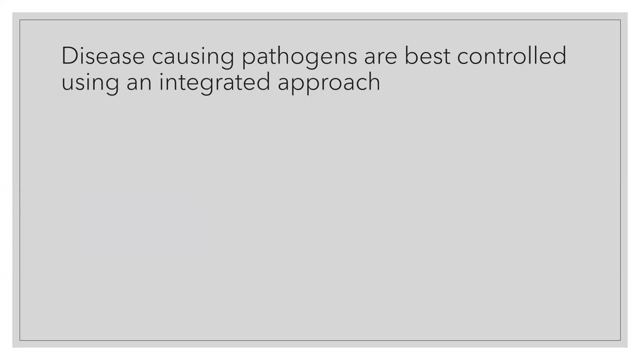 So we know that can really dramatically reduce heavy metals risk in things like leafy greens and roots, which I'll show you later. So disease causing pathogens are also- I want to focus- best controlled, really using an integrated approach. So I'll talk about how. 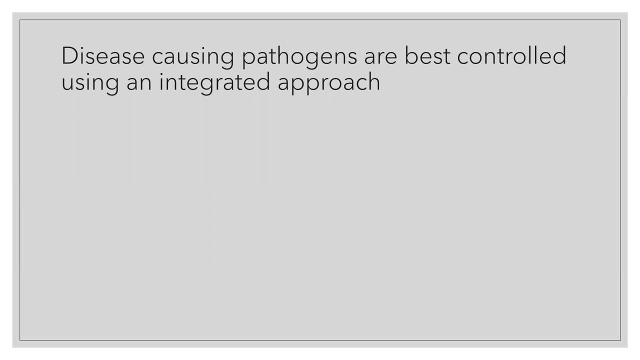 we're using soil amendments, but it's good to always step back and just think a little bit about what causes pathogens as a way to develop more of an integrated approach to manage them, And so when we look at what causes pathogen outbreaks, we often point to this disease triangle. 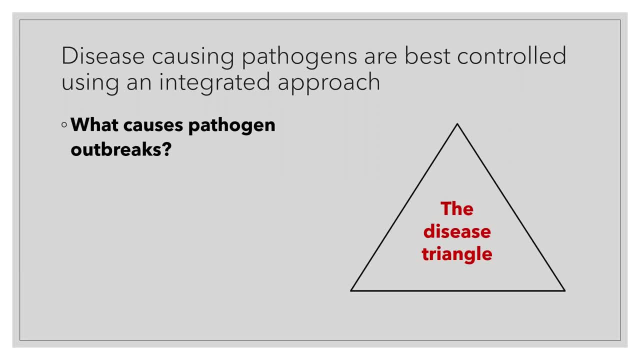 which highlights three factors that need to be present for a disease outbreak to occur. First of all, you need to have the presence of a susceptible plant. You need to have the presence of a susceptible host. Next, the presence of that unwanted pathogen. 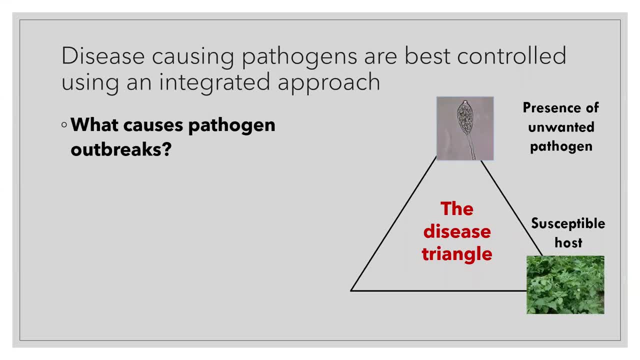 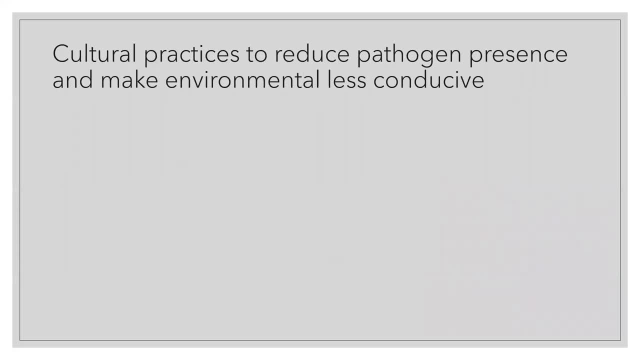 In this case, this is an oomycete Phytophthora pathogen And then a favorable environment for that pathogen to grow, And so, again, there's many ways to think about controlling pathogens that cause disease, And there's some simple things that you can do ahead of time to really try to make. 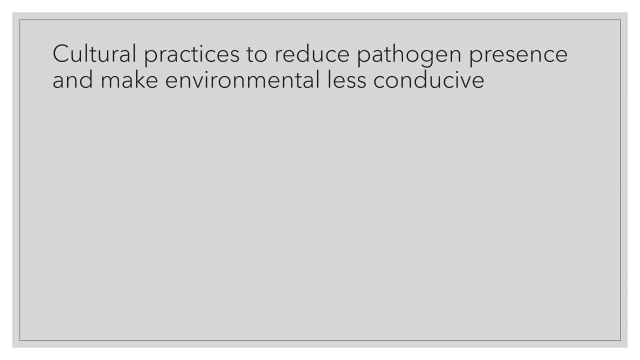 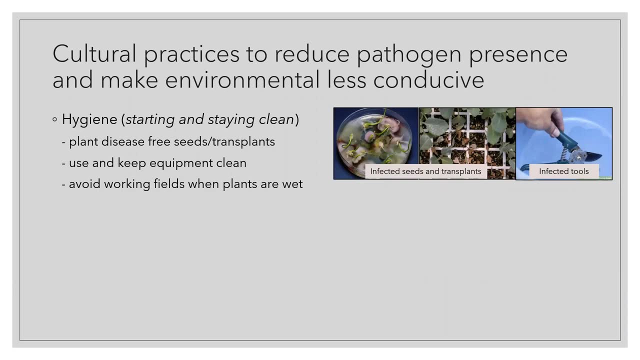 both reducing pathogen presence, but also making the environment less conducive. For example, proper hygiene- just always starting and staying clean. There are pathogens that can be transferred on infected seeds, transplants, infected tools, And so making sure you're always starting clean is a great way to help reduce some of the risks and also avoid working fields in the morning when they're wet. 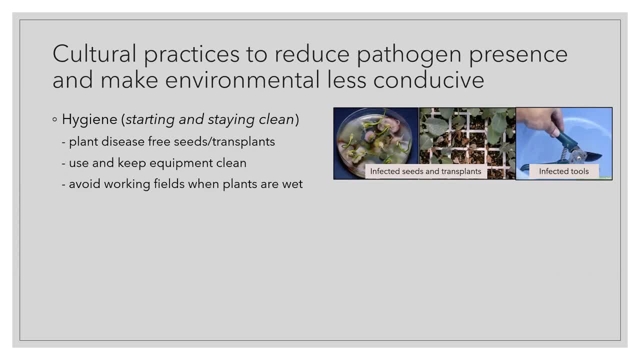 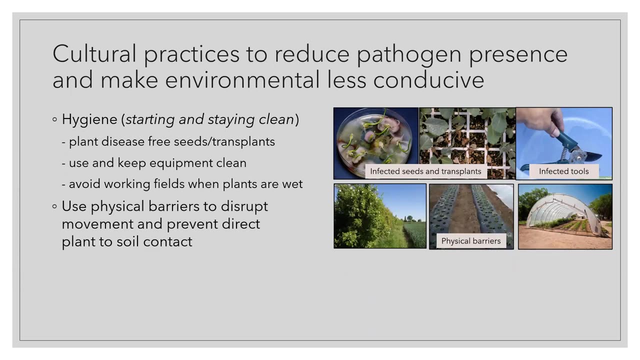 because you can actually move pathogens On your body or your tools, as you're from one area of the field when you move through that. So also there's lots of ways to just use physical barriers to to help disrupt the movement and protect plants from some pathogens. 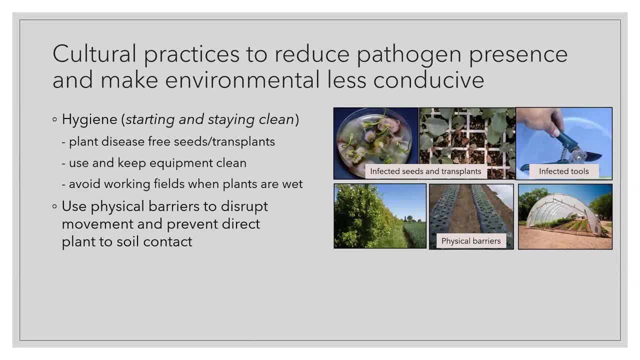 things like barriers here that prevent some wind flow, But, more importantly, there's a lot of soil pathogens that can live in soil And splash up onto plants and infect them on the leaves, And so using things like physical barriers like these raised beds here or covers like this high tunnel here can help to reduce some of that soil splash and reduce disease outbreaks. 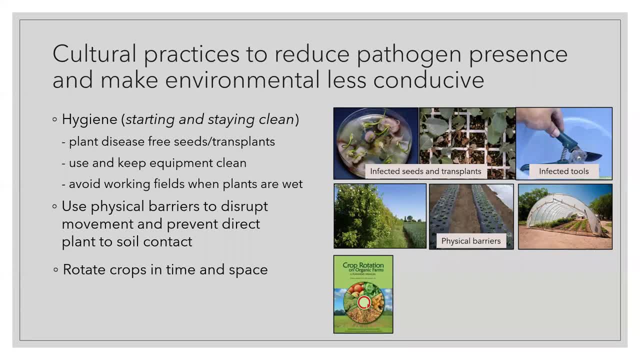 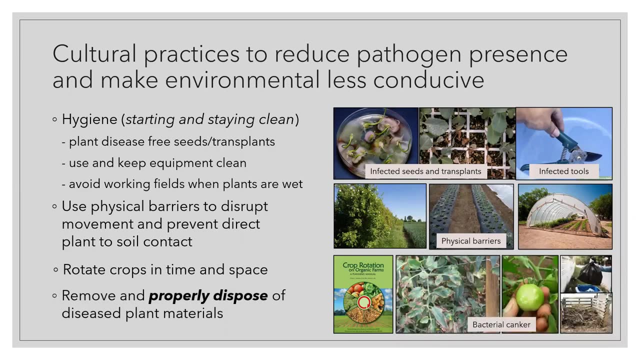 Of course, rotating crops and time and space, And if you don't have this resource, definitely check this out. It's available for free through the Sustainable Ag Research and Extension Program, SARE. You can download it And then also always think about removing and properly disposing of diseased plant materials. 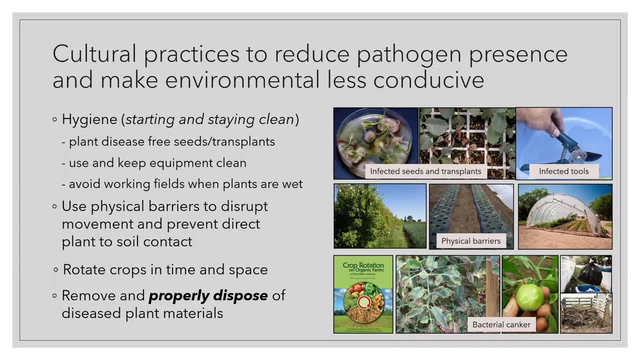 So some pathogens like bacterial canker here can survive for a long time on infected plant material in the soil. If you put it in a compost bin and don't really get that heated properly, you might not destroy that. So in some cases, particularly with pernicious pathogens like this, 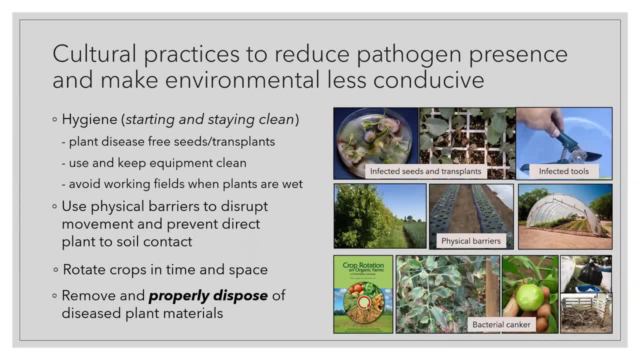 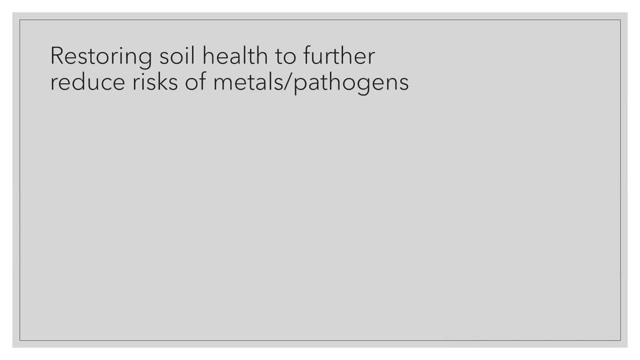 you might want to actually bag those up and remove them from your system. So now we'll get more into the heart of the matter and what we can do, how we can think about these relationships between soil health to further reduce the risks of metals and pathogens. 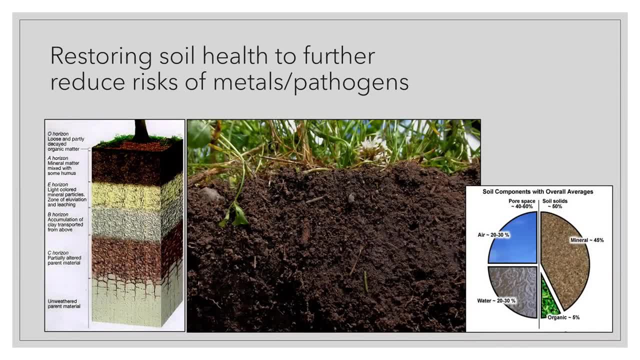 So healthy soils look something like this: They developed over millions of years, And so on the left you see this soil profile where you have this nice rich, dark topsoil up at the top And as you go farther down, less weathered parent material and so less productive soil. 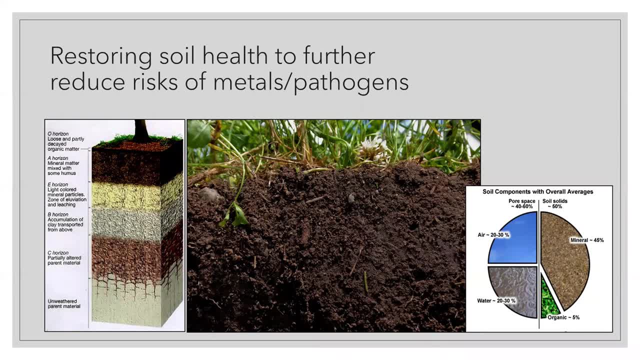 Soil should look kind of like the middle here: darker, crumbly. It smells nice like soil and it'll have a distribution something like this: This is pretty general, Where about half of a soil is actually space For to facilitate air and water movement. 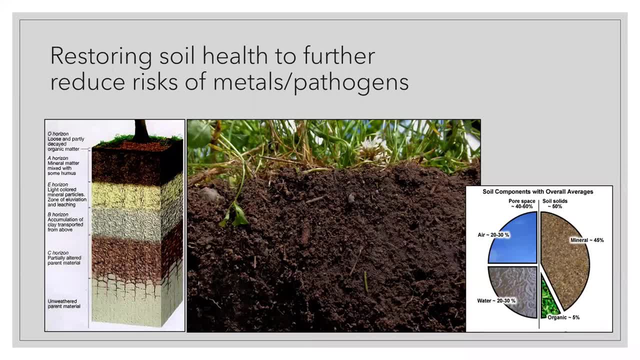 And then you have about 45% minerals, sand soil and clay, and anywhere from 0 to 5% in a normal mineral soil organic matter, And so when you have balances like this, we know that healthy soils can provide a lot of great agro ecosystem services, such as providing nitrogen. 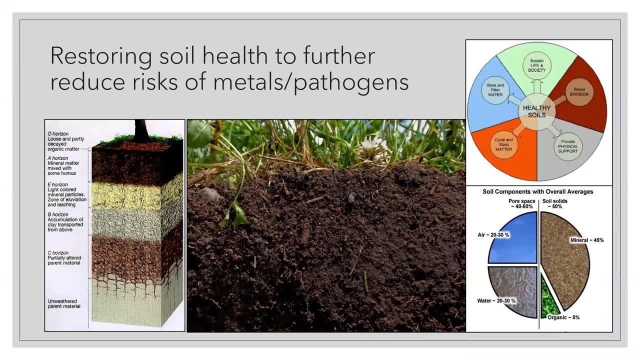 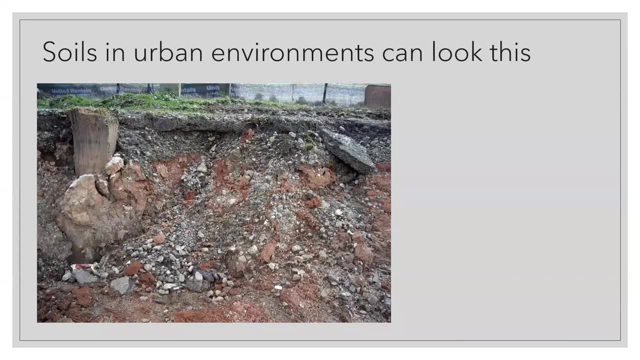 nutrients, suppressing pathogens- you know all these things that that soils can do. Unfortunately, though, in cities, we can sometimes come up to something that looks like this, And so I always throw this out in my students where, when I teach, urban ag. 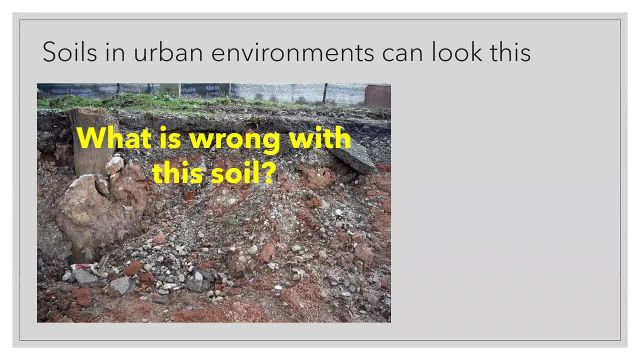 you know what is wrong with this soil, And there's a lot of things that are wrong with it, unfortunately. So it's obviously full of debris that needs to be removed, But when we start thinking about soils and how it acts, we can see that that profile has been destroyed. 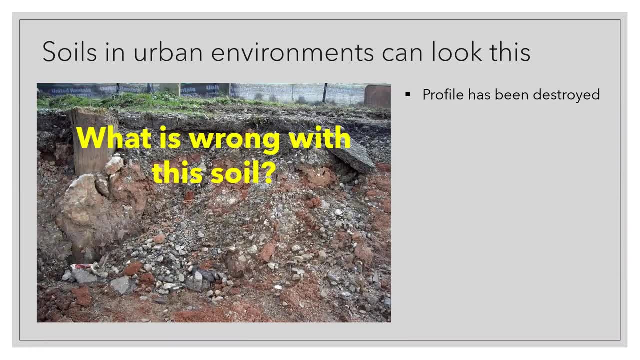 A lot of that. that really nice topsoil might be gone. It lacks soil structure and tilth, which will disrupt how roots and water is moving through that. soil Lacks organic matter and nutrients, which are really important for feeding plants, as well as soil biology. 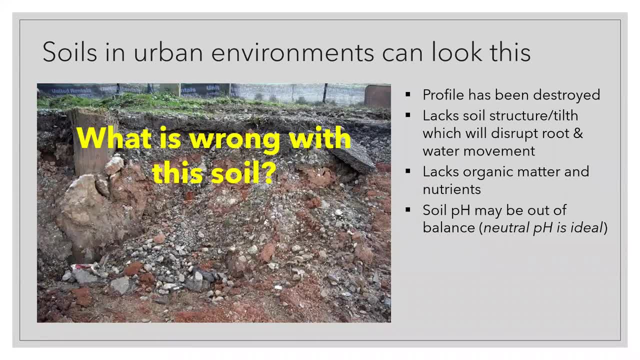 The soil pH is likely to be out of balance, And just you know. quick caveat: neutral pH is generally ideal between 6.5 and 7.5. To get a proper nutrient uptake, The biological activity is likely to be very low. 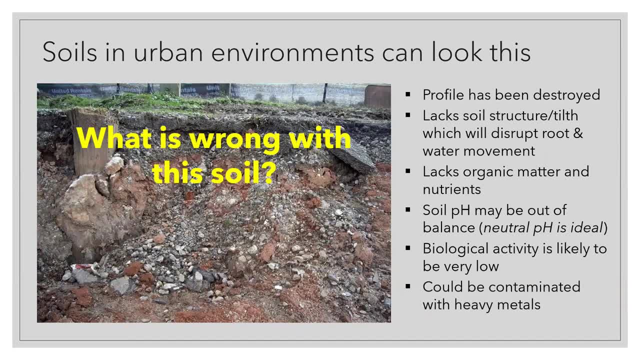 And then, of course, it could be contaminated with heavy metals. So what can be done to improve this soil? Again, if you're starting something this bad, you've got a lot of work to do in sorting through that soil and removing a lot of that debris. 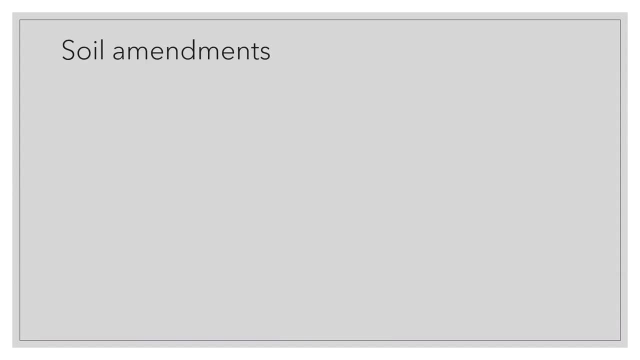 But we're going to talk more about the topic at hand and that is soil amendments, And so there's a whole lot of different soil amendments that we could talk about that we've explored in my lab and other people you know around the country and world have explored. 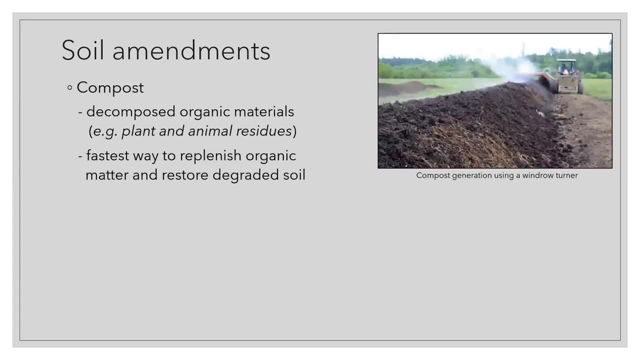 But today we're going to talk more specifically about composts, which are just simply decomposed organic materials generally derived from plants or animal residues, And this tends to be the really fastest way to the fastest way to replenish organic matter and to restore a degraded soil. 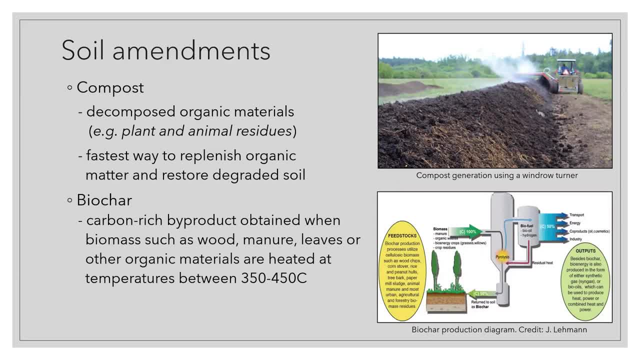 And we're also going to talk about biochar, which is another soil amendment that's received a lot of attention, especially around heavy metals and some pathogen work, which, if you're not familiar with, that, is a carbon rich byproduct attained when biomass. 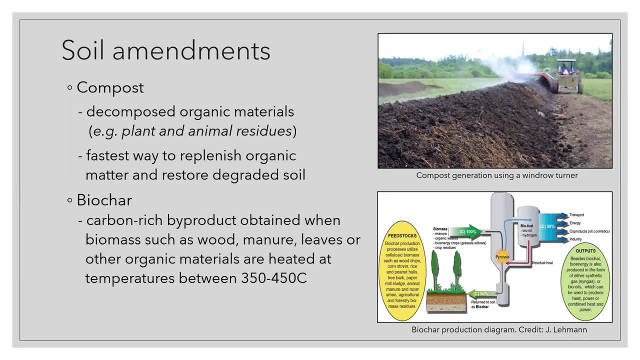 which can be anything, and other organic materials are heated at temperatures between 350 to 450 degrees Celsius generally, And so both of these, as I've said, have potential to address heavy metals and pathogens. but you're what you'll see as I go through these slides is that we often see lots of 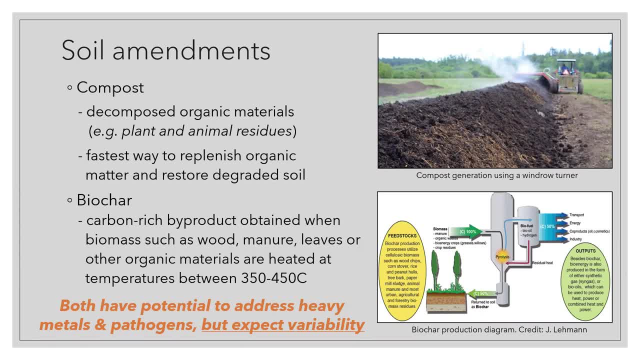 variability. So not all of these do what we'd like them to do, And there's a number of reasons for that. And so when you're thinking about, you know, using soils as a way, you know to, to help plants. 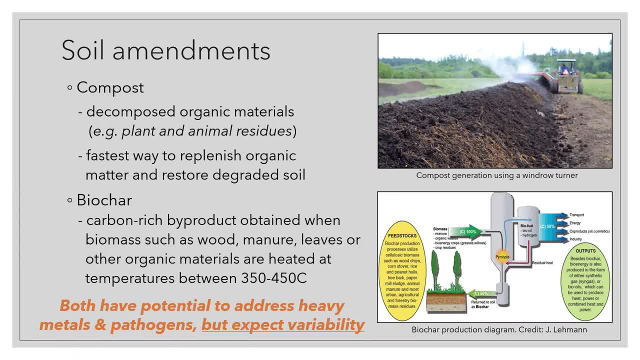 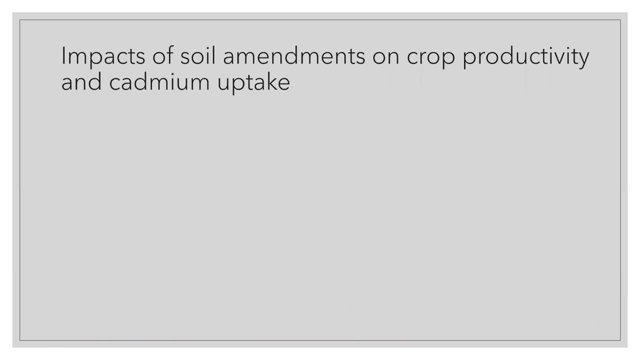 especially with pathogens or metals. remember that this is one technique out of many tools that you should be using to address problems. So, first of all, you know what? what's some evidence that these path or these soil amendments can influence some of these? 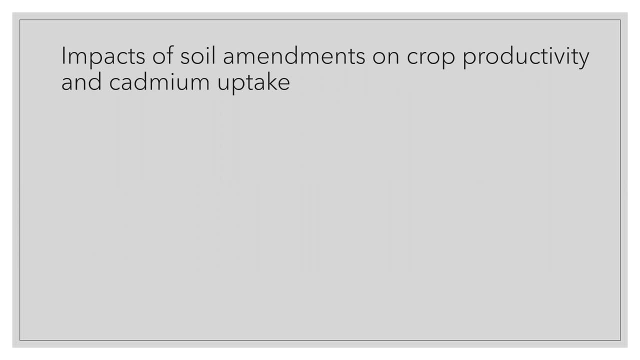 the heavy metals and pathogens, And so first we'll just talk about a couple studies we've done, really focusing on cadmium. We often work with cadmium because we know it's the most bioavailable in the soil. It's very toxic at small concentrations. 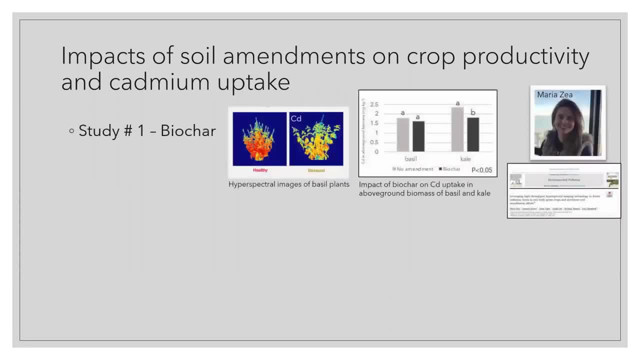 both to people and to plants, And so this is one study that we recently wrapped up. This is Maria Zea. She was a master's student in my lab, And, and really the focus of her study was trying to develop the use of hyperspectral imaging to be able to detect. 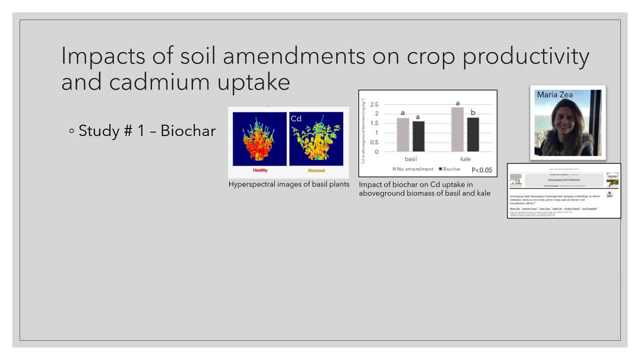 and start to develop better ways to deal with heavy metals. And so that's this cute little picture you see here, because this allows us to see things we can't see with the naked eye. So we can see when plants are stressed or not. 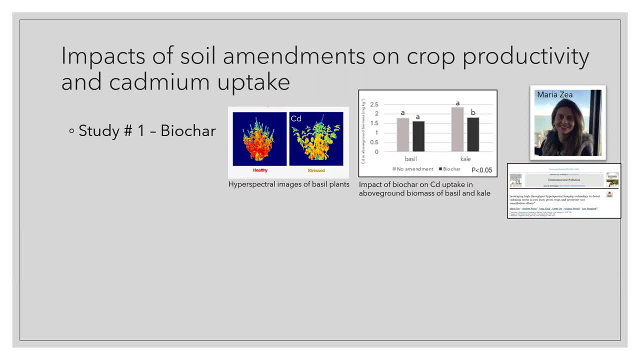 But as part of this she looked at one local woody biochar and wanted to see if that can. we could both detect that. but also would it really reduce cadmium uptake? And she had some pretty high rates within her study, going from zero all the way up to 15 parts per million cadmium in the soil. 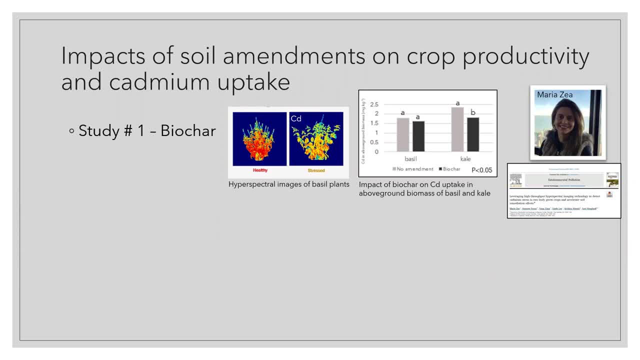 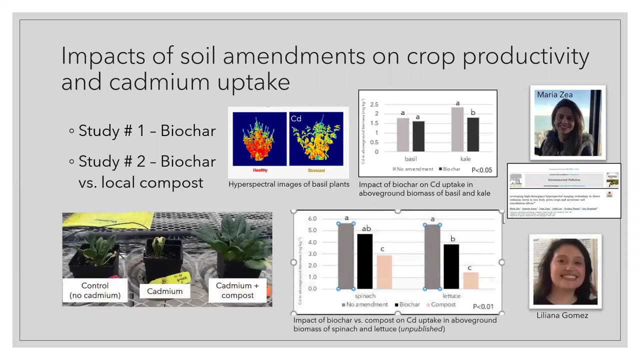 And so she really only saw a very slight but not statistically significant difference with basil, but did see a reduction overall in kale, And you can learn more about that in the study she recently published in environmental pollution. Second, this is another study we did: 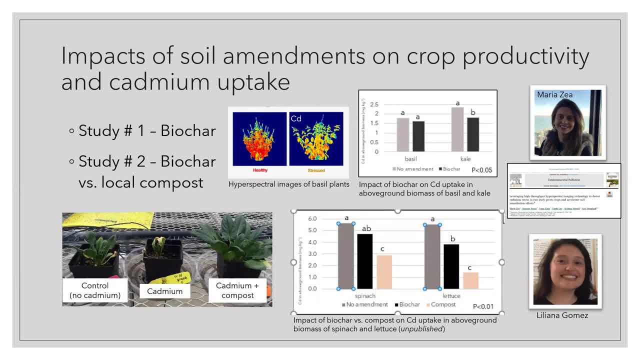 This is Liliana Gomez, who was looking at a number of different soil amendments and their capacity to reduce cadmium uptake, And I'm just going to focus in here on another biochar that we tried, as well as a local compost, And I love this set of pictures that she developed here on the left. 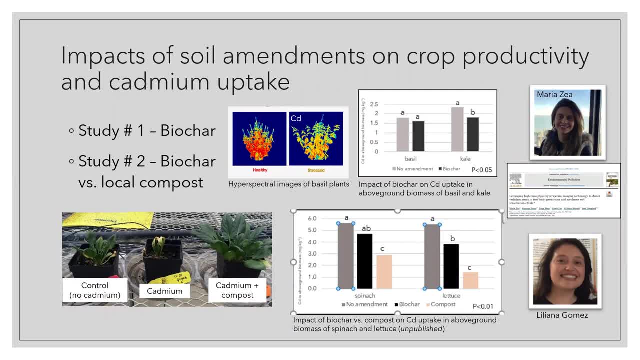 You can really see this is the control. This is a spinach plant that had no cadmium. When the soils are amended with cadmium we get quite a better response, But when she had both cadmium and this local compost in this case, 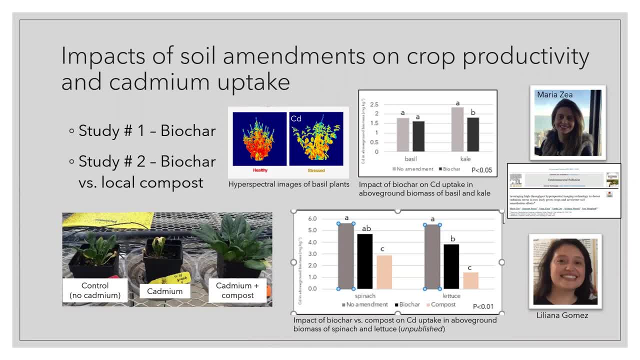 dramatically reduced, improved the productivity of the spinach as well, as we saw a nice linear decline in cadmium uptake. And so with the spinach again, the biochar did not reduce cadmium uptake relative to the control, but we did see some reduction with the compost. 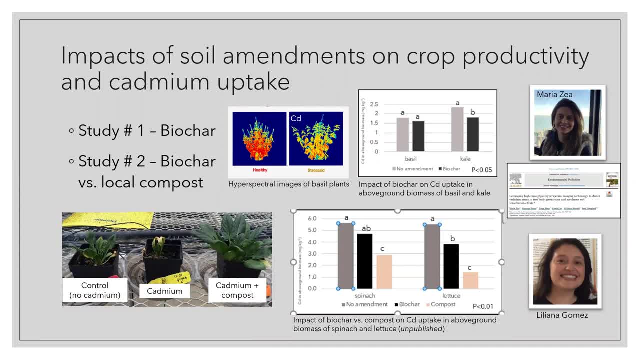 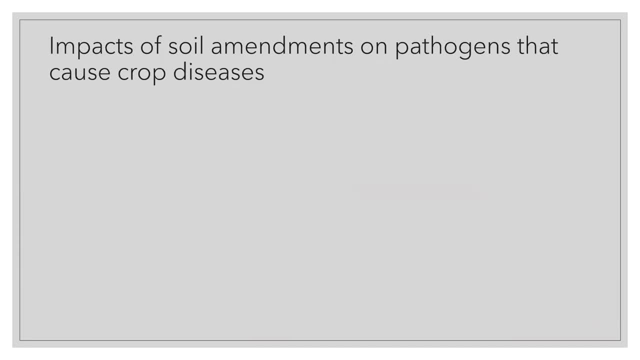 And then in lettuce. we saw a decline in both, but the most impact from using that compost. So next, what about the impacts of soil amendments on pathogens that can cause crop disease? So we've also done a number of studies in this area and looked at different 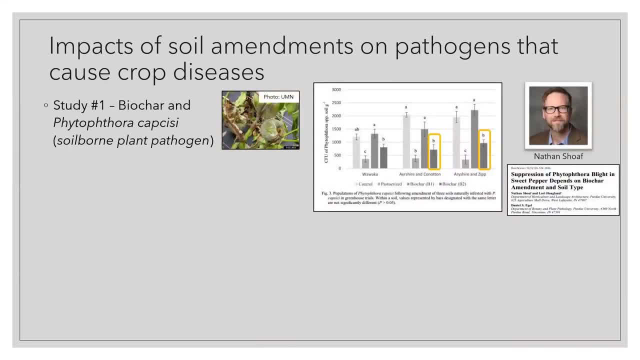 ways to deal with that, And so one study I want to highlight here. this is Nathan Shoff's work, who's now our urban agriculture coordinator here at Purdue University, But this was a study he did a few years back, looking at investigating whether two different types of biochar could save. 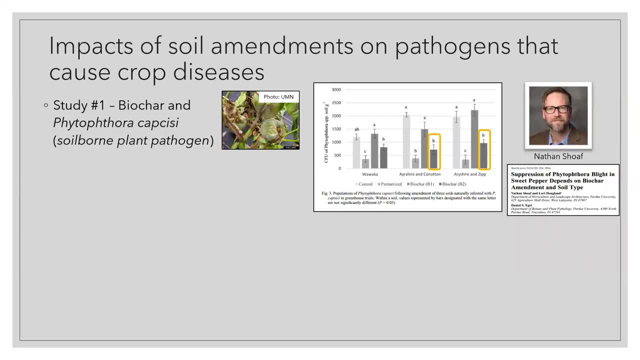 the soil-borne pathogen Phytophthora capsici in pepper. And so there, he used three different soils And if you look at this figure here, this is the this colony forming units of Phytophthora that were left in the soil after the. 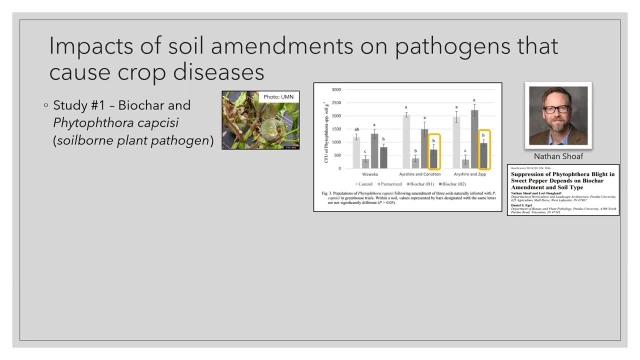 treatment and the crops were grown, And so I've got these little yellow squares here to point out that. so, on the left is just the control, The next one over is pasteurized soil treatment, And then we have the two biochars. 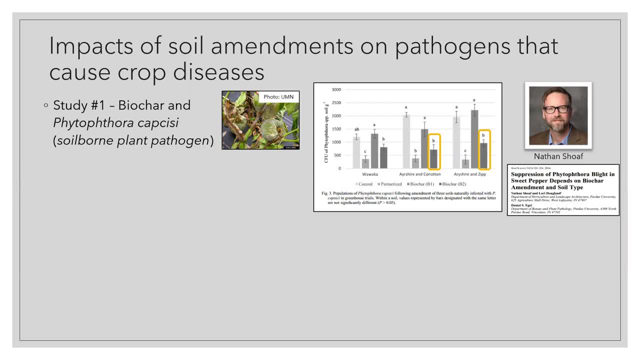 these two bars on the right and the three soils along the bottom, And so, really, what I want you to see here is one of the biochars worked well in suppressing the disease relative to the control, but in the other biochar did not, and it worked in two soils. 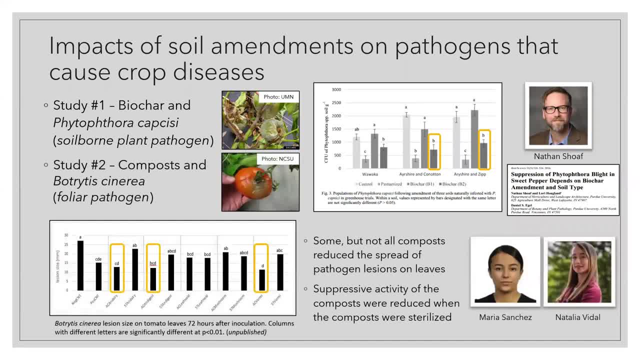 but not another. So next, this is another set of experiments. we've been doing two at a time and we've been working with other students- Maria and Natalia worked on this- where we've been working with a number of local pathogens or compost. 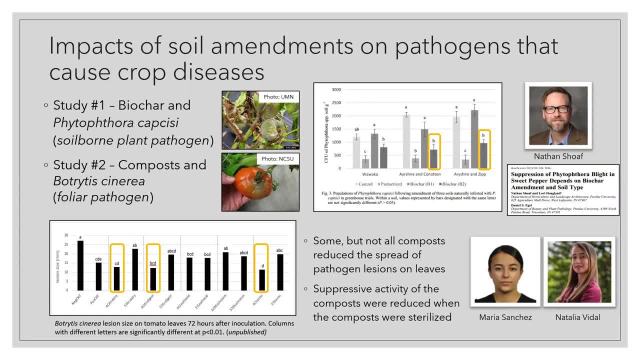 sorry, and seeing if they could actually induce systemic resistance in tomato, So making tomato stronger and more resilient against foliar pathogens, in this case Botrytis, which causes gray mold. And so if you look at this figure here on the bottom, 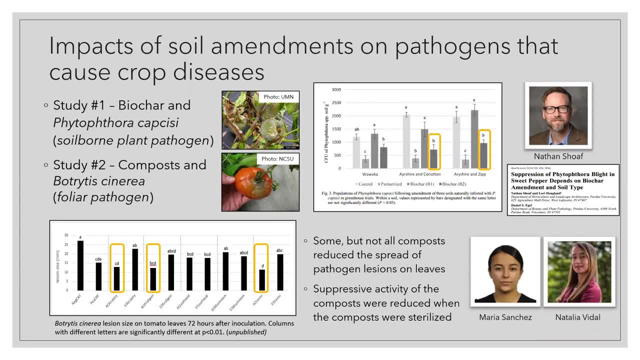 on the left is the control. They had no compost. And then we have a trichoderma positive control next to that And then five different composts and the composts were either active or they were sterilized to move, remove their potential biological activity. 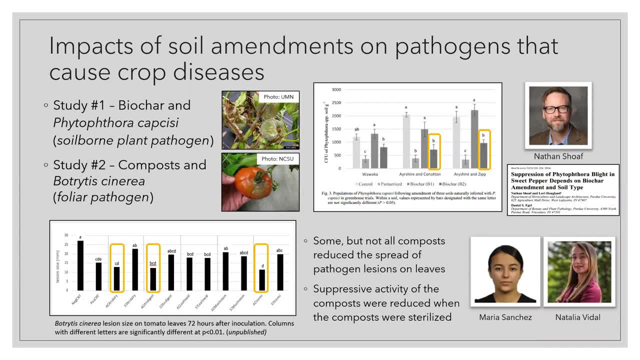 So we could really understand what was potentially causing pathogen suppressiveness. And so what you can see here again, the ones kind of highlighted in gold are the amendments, the active amendments, that reduced the spread of the pathogen on the leaves relative to the control. 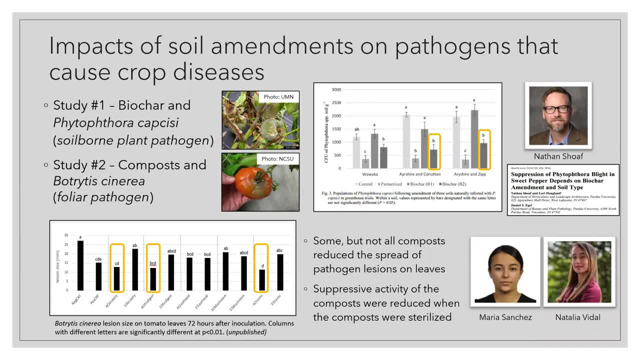 And so some again, but not all of these path or composts were pathogen suppressive, And the suppressive activity was reduced when the composts were sterilized, So indicating more of a biological component that we're digging into a little bit more right now. 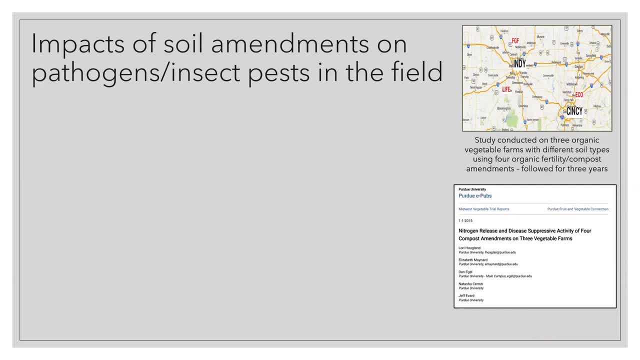 So next, what about in the field? I just want to quickly highlight this study. This was a several year project that we did at three farms near Indianapolis and Cincinnati several years ago, where we applied for different amendments in the field And we looked at natural infestations of pathogens and pests as they occurred. 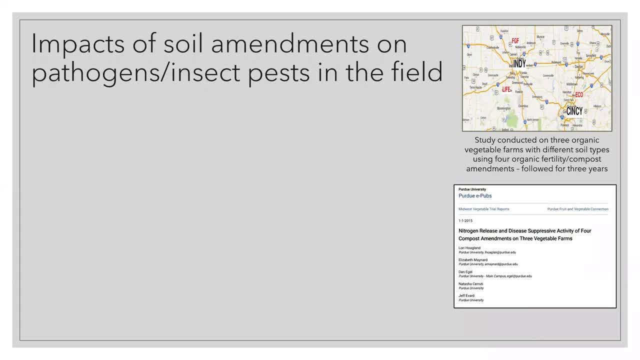 and then tried to understand what was happening, how much that related to things like nutrient uptake or increased microbial activity in the soil, And so I'm going to show you a lot of figures. Don't worry. The main point is just seeing some of this variability. 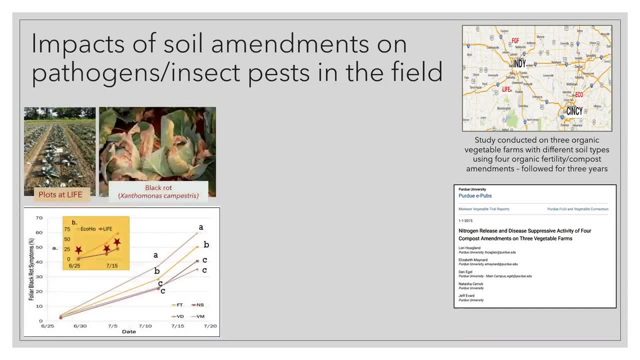 So in the first year we planted cabbage in all of the fields, And so one of the pathogens that came out that we saw at all three locations was this black rock caused by Xanthomonas, And in this little figure here you can see the foliar symptoms of black rot over time. 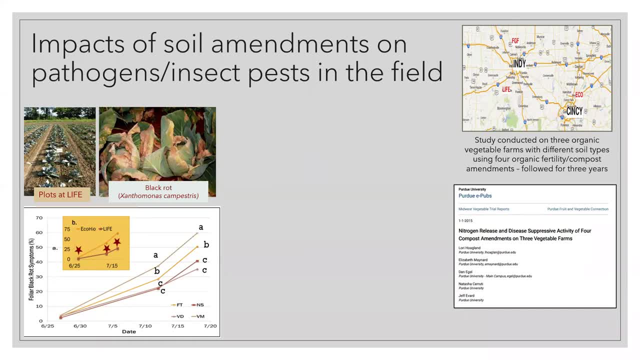 And these are these four amendments that we were testing, And so we did see a difference between the amendments and how much they were suppressing the development and damage caused by this disease relative to others, But we also saw some differences between the farms In the second year. 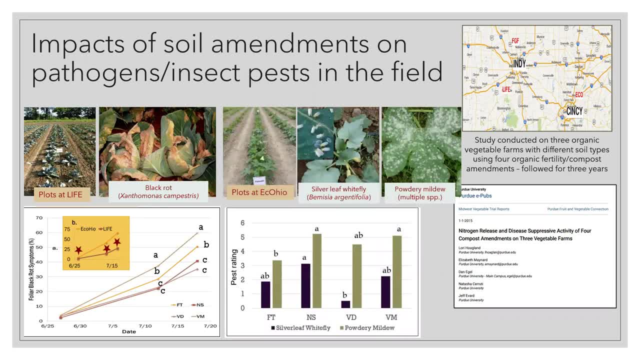 we've planted squash at the three locations and we had two pests that came out. One was the silverleaf whitefly that caused some damage and the other was powdery mildew that was caused by multiple species. And again on this figure, 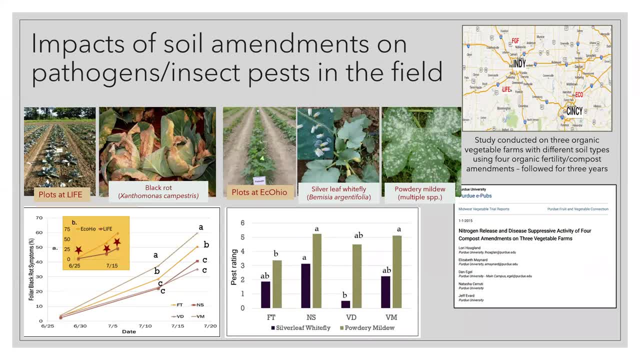 you can see that there was variability in how the amendments were influencing the pest ratings. in this case we're measuring. So the silverleaf whitefly, for example, this amendment was very effective in suppressing the outbreak of this disease, And so we were able to see that there was some variability in that pest or damage caused by that pest. 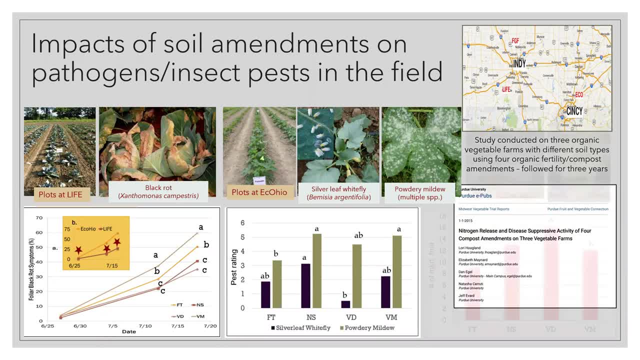 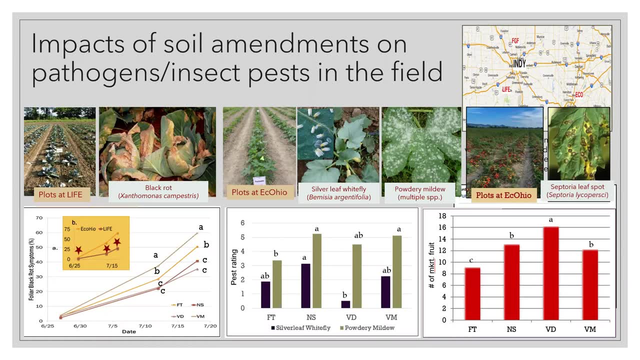 And there was some variability also in powdery mildew damage. In the final year we grew tomato And just to say these were. you know, we're compounding the effects over time. So looking at changes over time and we 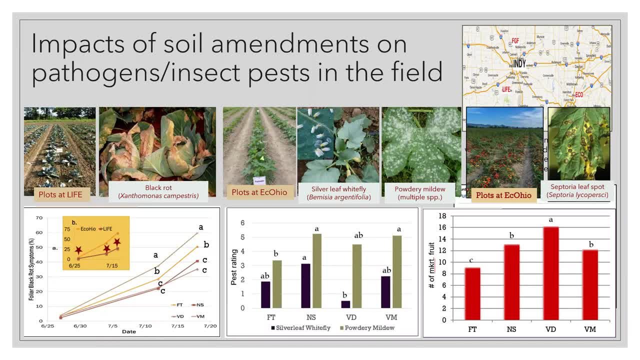 and this septoria leaf spot was something that came out. It's a big problem for us. here in the Midwest We grew this just paste tomato, but we also saw differences in how the amendments- in this case this is- marketable yield. 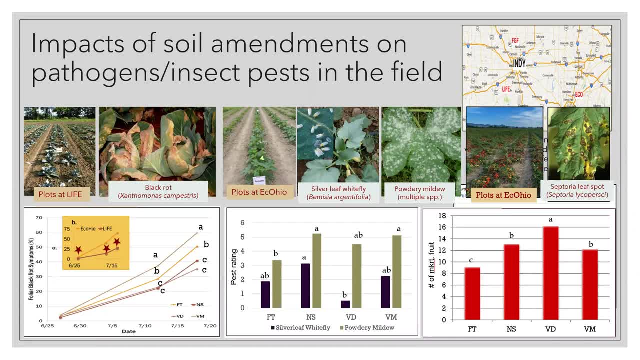 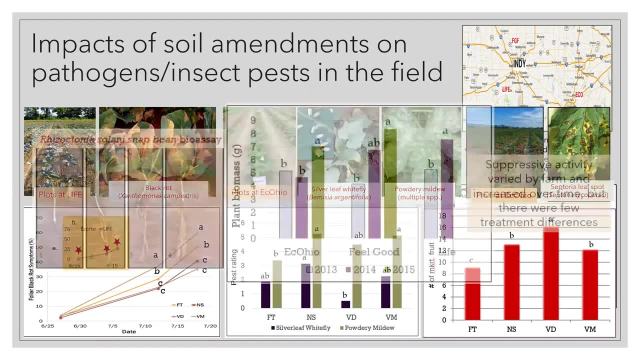 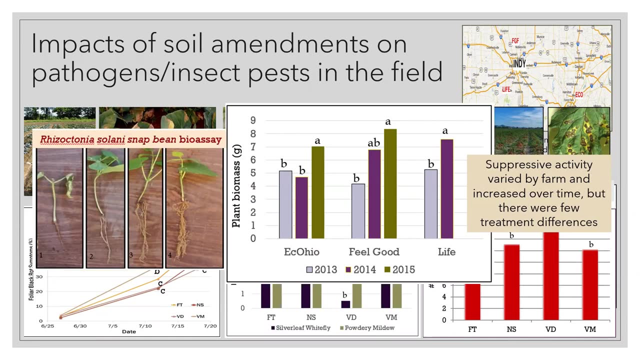 So we saw differences in damage, but also this influenced marketable yield. So this VD amendment was where we saw the greatest benefit. So, lastly, we wanted to see, okay, three years of amending soils with these composts. What happens if we take the soils now and add a soil borne pathogen? 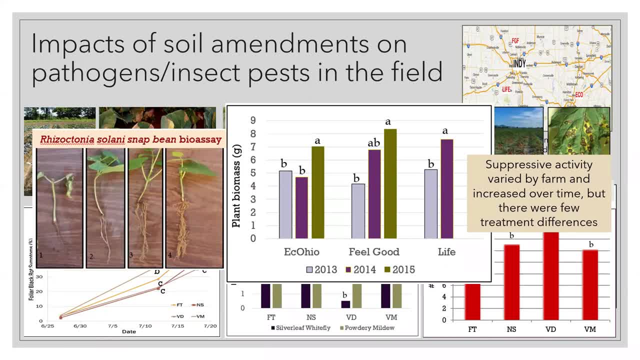 Have we changed the resilience of these soil communities? And so we took the soils and we inoculated them with rhizoptonia in the lab and grew snap bean And then, over the years, looked at how this changed, suppressed activity, And so this is plant biomass. 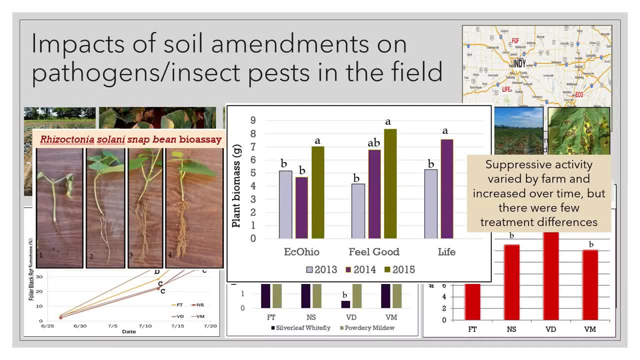 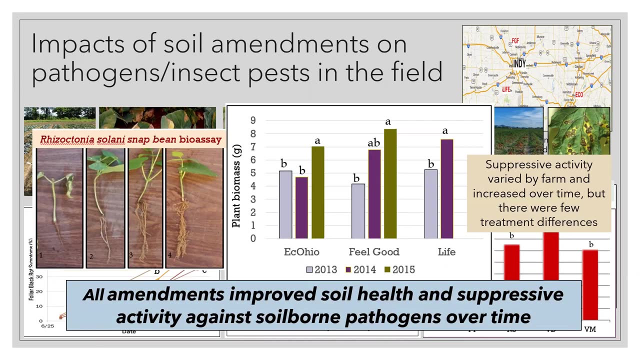 So this is how well the plants basically survived in these systems, And you can see that there was some variability among farms over years, but really over time we saw that all of the soils became more resilient- More resilient against soil borne pathogens, And so in this case too, 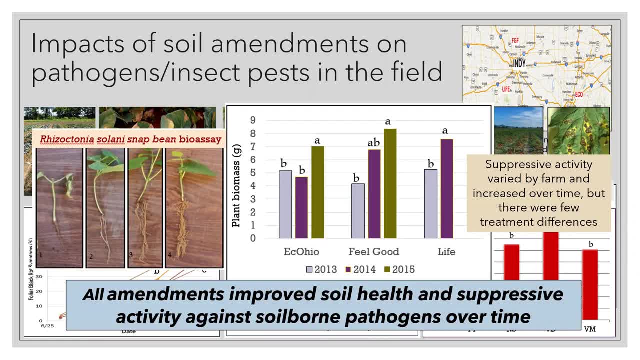 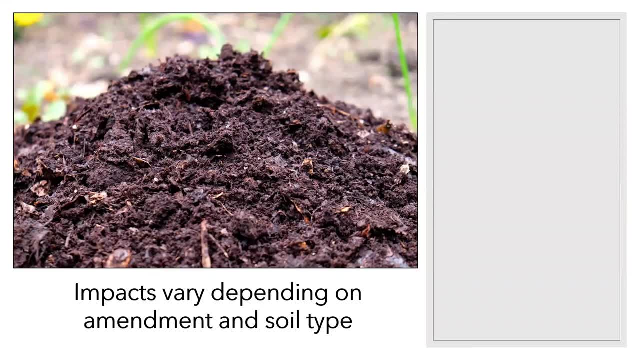 all the amendments improve soil health and suppressive activity over time. So what I was showing you there was a lot of data, a lot of slides, a lot of different amendments, And so one of the points I want to make, which is really challenging when you start thinking about soil health and trying to manage it with soil amendments: 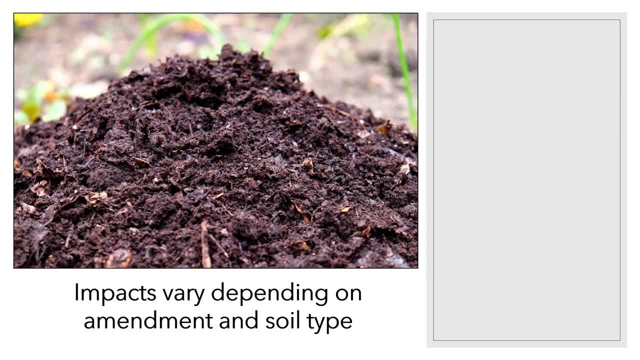 is that we do see the impacts vary depending on the amendment and soil type, So it's very challenging to manage, And so now I want to move just a little bit more in. you know why is this the case. We're continuing to work in this area to try to better figure it out so we can provide better recommendations for you. 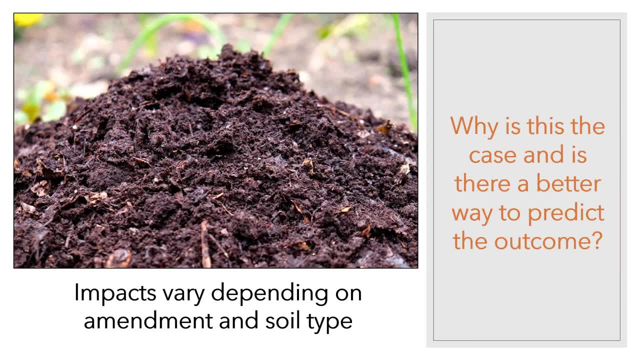 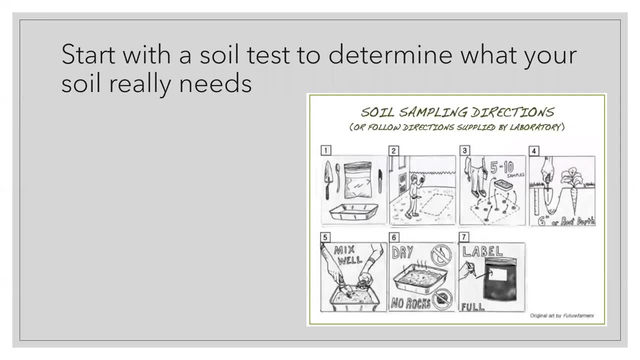 But these are some things I hope that might help as you think about ways that you can better manage your soils to deal with these stressors, To deal with these stress factors. So, first of all, you know you should always start with a soil test to determine what your soil needs really are. 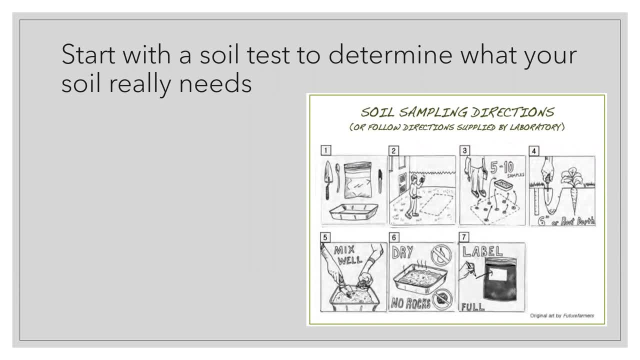 You know what is the current status of your soil? Is it, you know? is the pH off? Is it low in organic matter? Do you have metal contamination issues? And I would encourage you to reach out to your local extension educator. 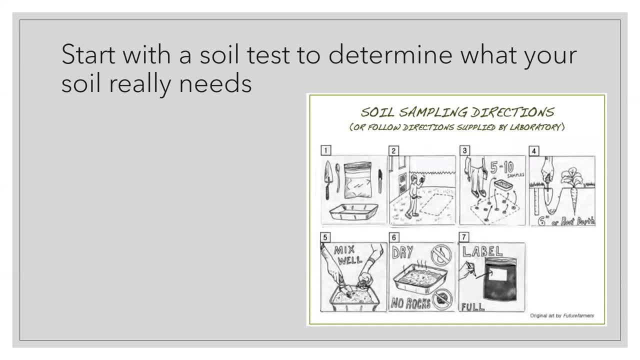 people in the Soil and Water Conservation District, or NRCS. They're they're very knowledgeable about that. They know a lot about how to take good soil tests and how to interpret the results, And so once you get these, then you can start to think about a little bit more. 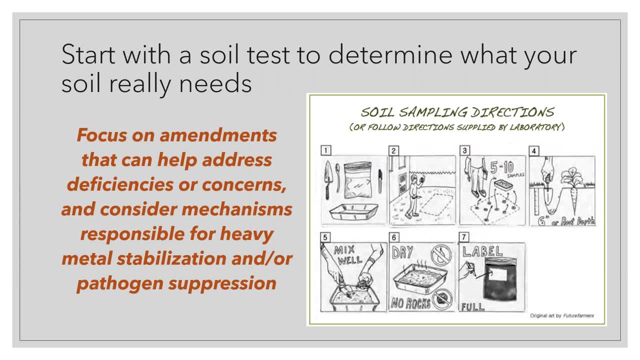 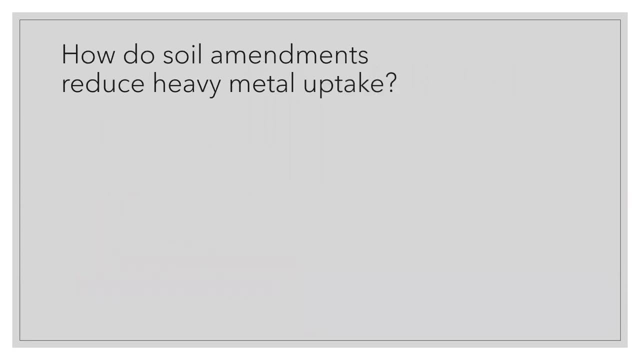 What are amendments that I can specifically use to address deficiencies and try to get my soil in a more healthy state to prevent heavy metal uptake as well as pathogen outbreaks, And so it's also helpful to- yeah, just think about two potential mechanisms. 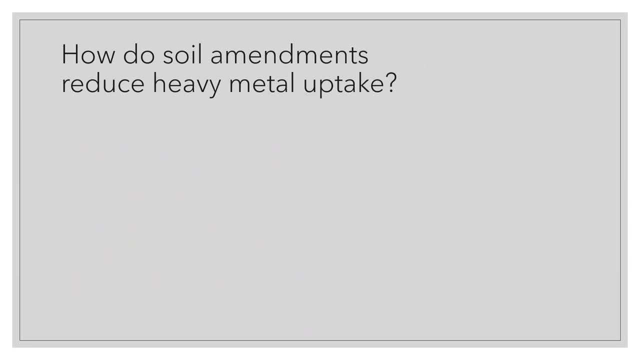 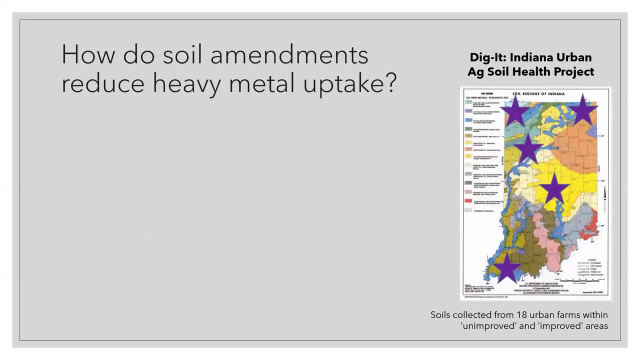 And so these are some ways that we know that that can influence some of the variability that we see in different amendments and different outcomes, And so I just want to focus or just briefly use one of this other study that we've been doing working on the past few years. 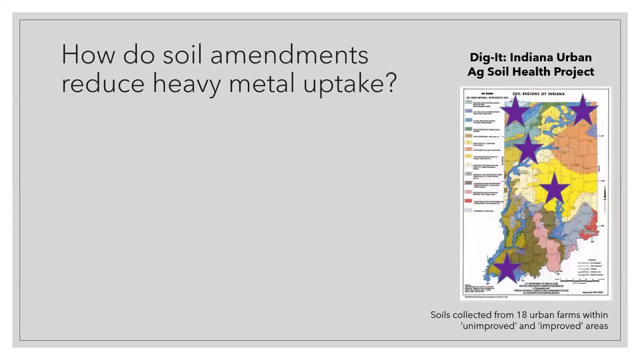 It's called DIGIT, the Indiana Urban Ag Soil Health Project, where we've went out and collected soils from 18 urban farms across the state and five different municipalities And we've done a lot of work on that And we collected soils from both unimproved and improved areas to try to understand how soils are changing. you know, in our farmers- urban farmers- meeting their goals. 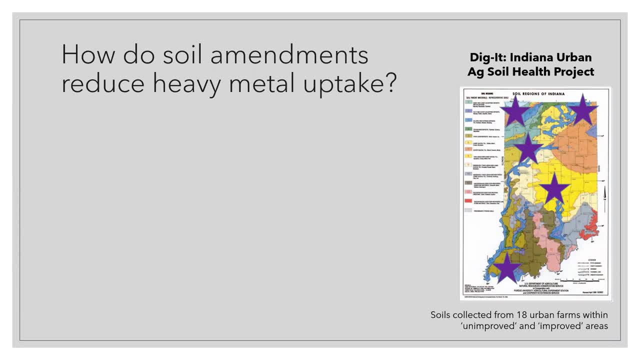 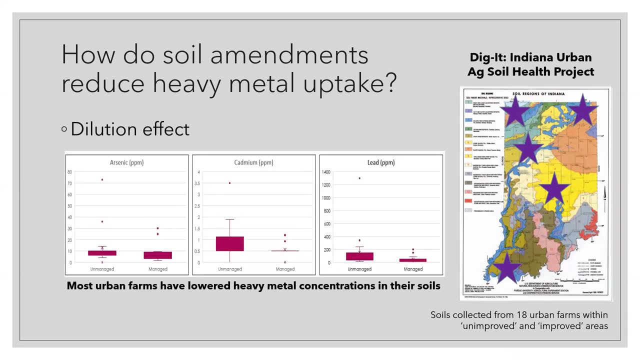 And where might they be running into problems. And so one of the things we saw, fortunately this is heavy metals in these sites. This is arsenic, cadmium and lead, both on the left- the managed, unmanaged sites and the managed sites. 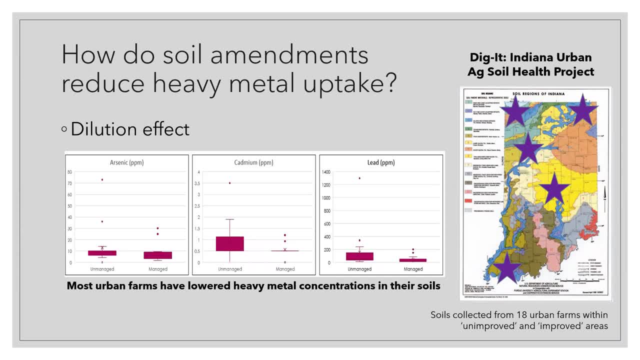 And so we did In most cases see a reduction in the amount, total amount, of heavy metals that are in these soils. We do have a couple kind of outliers, areas of concern, But in the most case we saw a reduction. 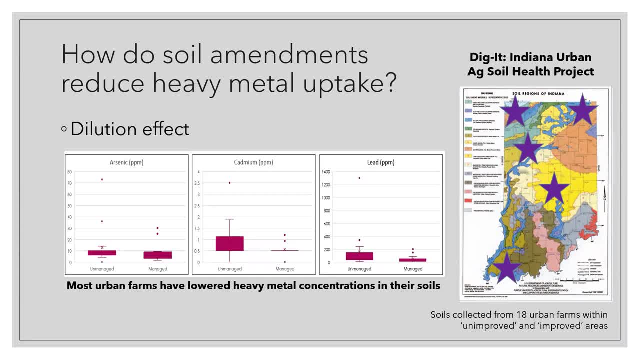 And we think this is primarily due just to a dilution of fact that people are adding a lot of amendments really approving increasing the organic matter in the soil, which just decreases the relative amount of heavy metals and therefore improves the safety within these systems. 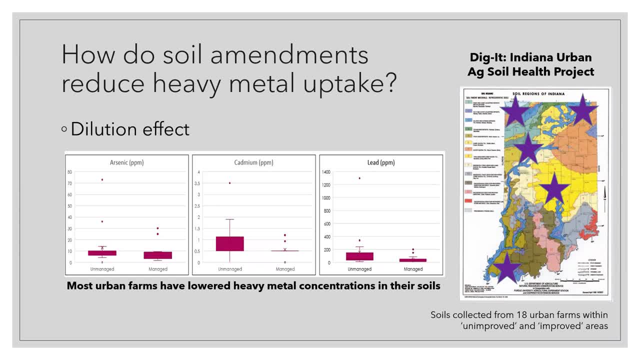 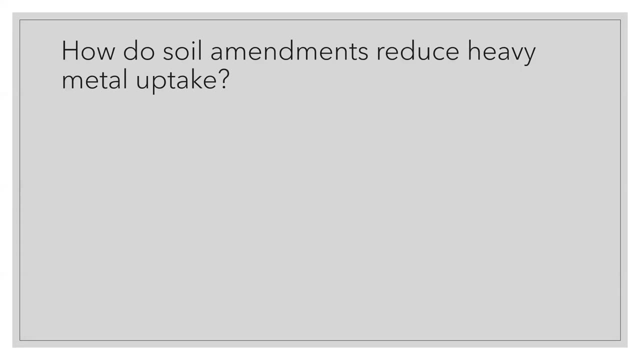 So if you know your soils, or you know, have some metals, they're deficient in organic matter. This is one way you can potentially reduce or improve your safety. So there's other ways that soil amendments can reduce heavy metal uptake, And so, first of all, 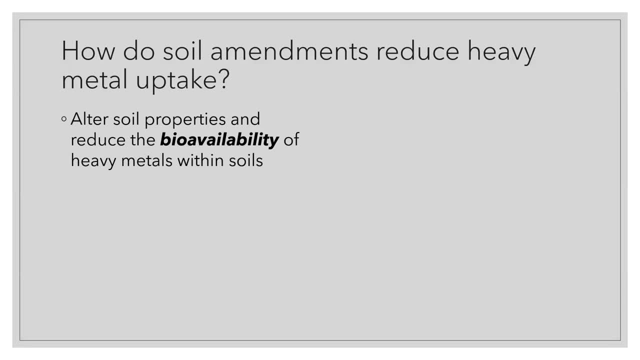 many of them can also reduce heavy metal uptake. Many of them can alter soil properties. that therefore reduces the bioavailability of heavy metals. So not all metals within soil are going to be in solution and available for crop uptake, So some of those can be bound in various ways that help to prevent crop uptake and therefore improve crop safety. 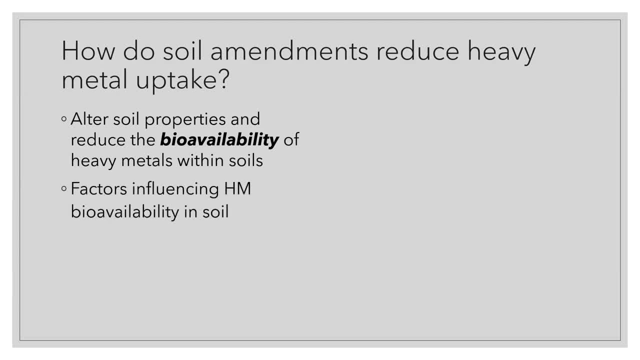 And so there's a number of things that can influence heavy metal bioavailability in soil, And what we know the most about is just various chemical properties. So there's been a lot of work over the years in trying to understand the role of chemical properties in reducing bioavailability. 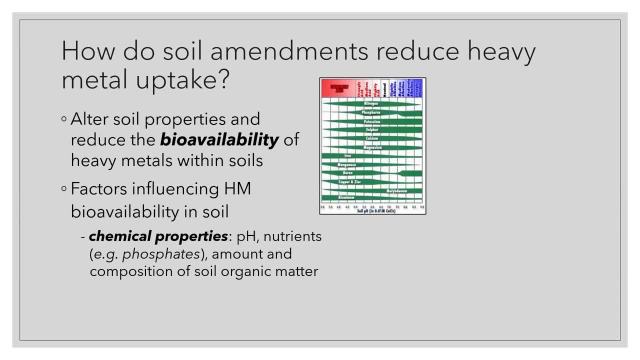 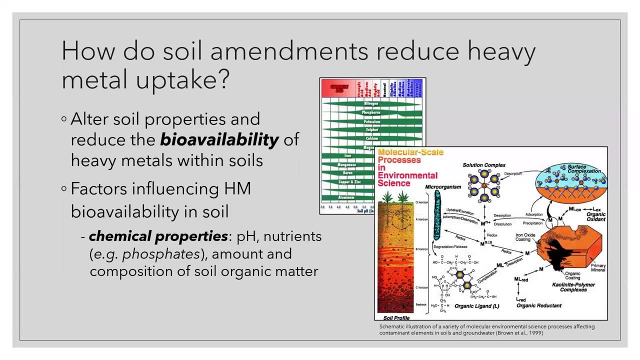 So things like pH is one of the most well studied. We know that most heavy metals tend to be more bioavailable at lower pH, So raising the pH of your soil can reduce the bioavailability of metals. And then there's all sorts of other ways, like the composition of the organic matter, that can bind heavy metals in various ways. 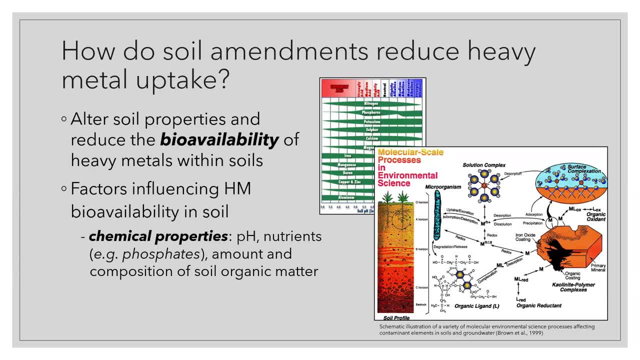 And so we know amendments are made with different chemical chemistries, different chemical arrangements, And so that can influence how well they are due at binding metals. Both the nutrients they provide- things like phosphorus and zinc that might be in there- can also play a role in binding those metals. 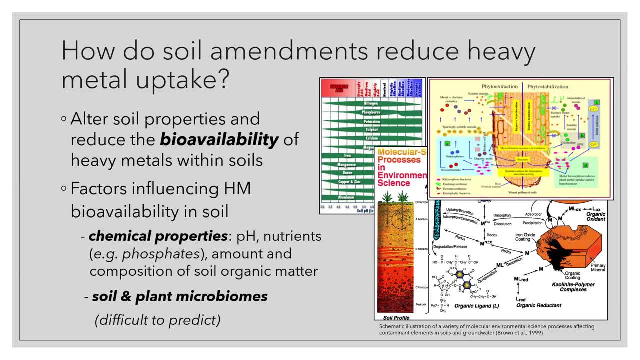 And then we know also that soil and plant microbiomes can influence the bioavailability of metals, both increasing in some cases, which is great if you're working with a phyto extraction, But if you're wanting stabilization, there are different mechanisms, And so there's a lot of people working on this, including in my lab. 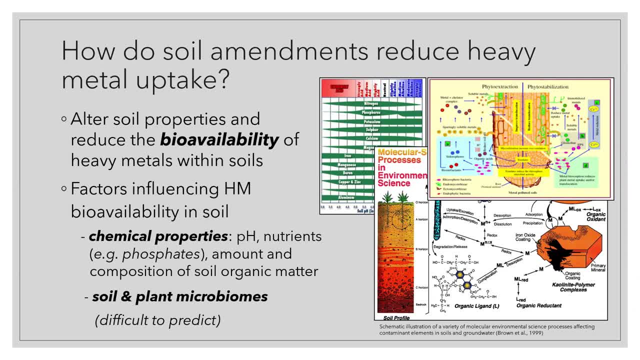 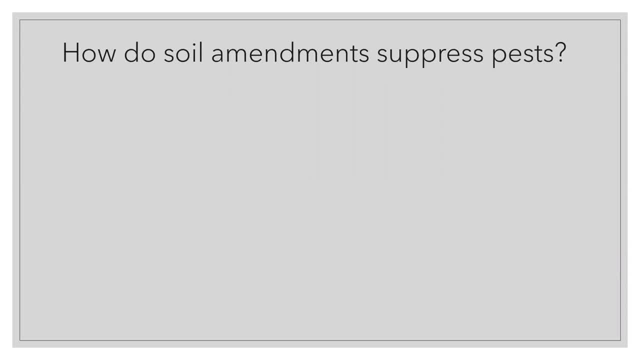 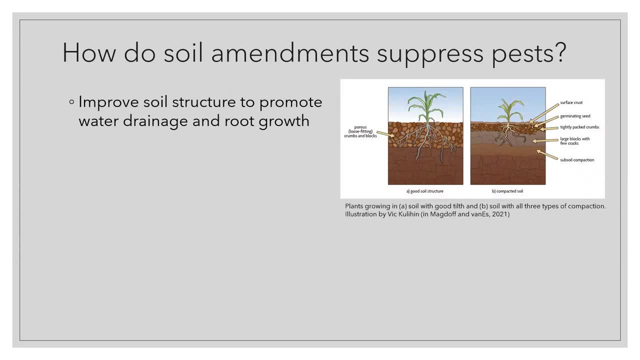 It's very difficult to predict, But we know that can play a role in some of the variability we see. So how are soil amendments suppressing pests? First of all, we know that a lot of soil amendments can just improve soil structure to promote water drainage and root growth. 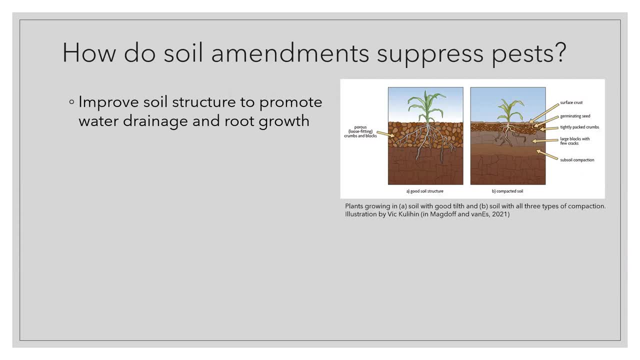 So in these city soils we can have very compacted soils, So water doesn't drain very well, A lot of soil borne. pathogens thrive in wet soils where roots can't grow well. So you know if you're in those types of situations bringing in bulky materials. 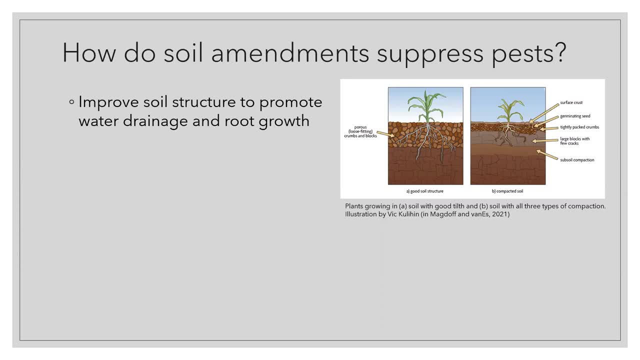 again like compost that can just increase the organic matter. improve the structure of your soil can go a long way in helping to suppress pests. Some compost have, and other amendments have, a little bit of plant nutrients in it too, which can of course make plants more resilient, stronger against pathogens. 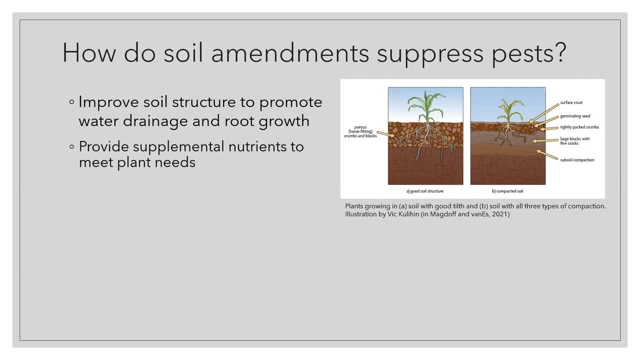 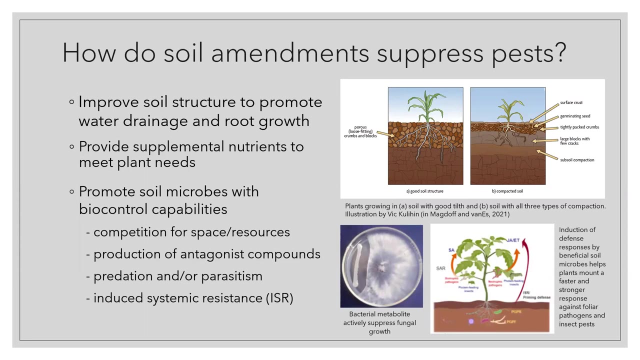 So, again, looking back at your soil test, what nutrients might you be deficient in is important to having healthy plants and resisting pathogens. And then, lastly, the area that I think is most interesting is all these beneficial microbes that can be within these types of amendments. 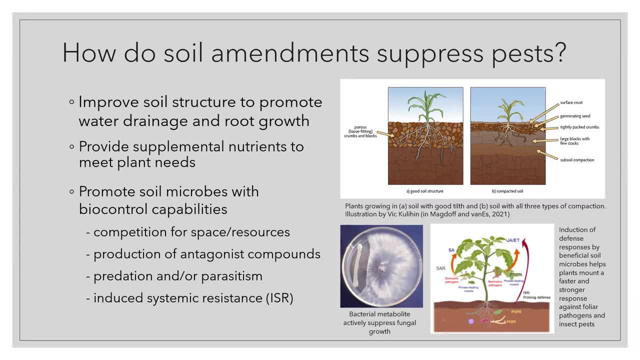 or that can boost natural populations in soil that have direct and indirect impacts on suppressing the pathogen, And so some of these might be Producing antibiotic compounds. like you see in, this little petri dish is kind of choking out the fungal pathogen. 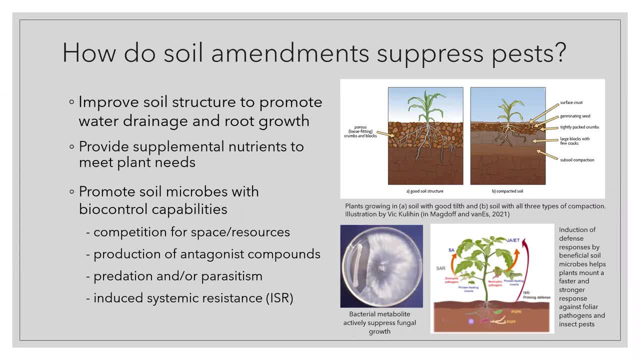 or they could be inducing systemic resistance. So basically increase kind of like a vaccine that the plant, it boosts its immune system and then it kind of regulates, But then when a pathogen lands on it it can mount a much stronger and more effective response against the pathogen. 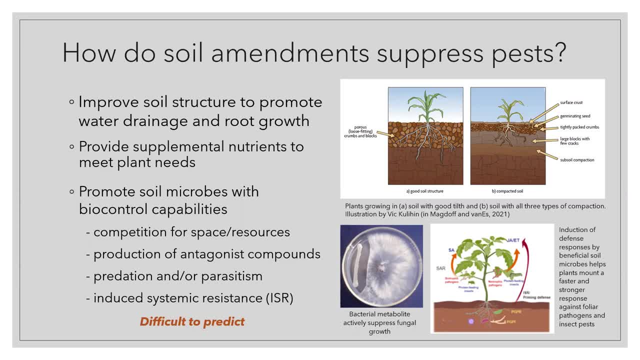 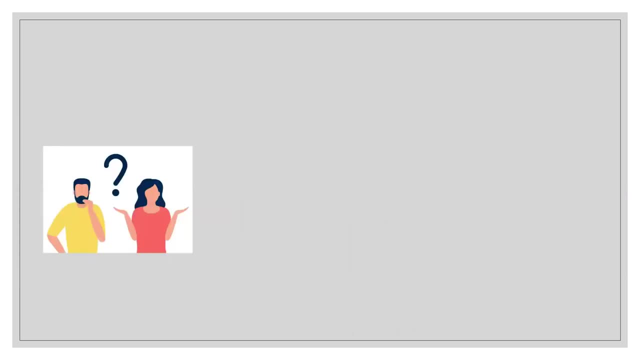 And so, unfortunately, this part is really difficult to predict. There still needs to be more work. exactly what makes one pathogen or one compost or amendment more suppressive in the case of some of these beneficials. So you're probably still thinking, wow, OK, that's a lot of information. 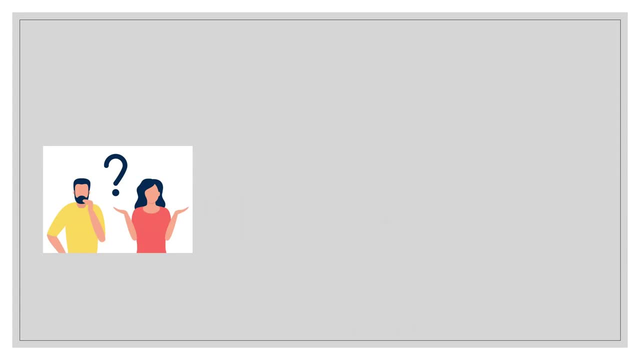 How do I take that and use it in some way to really better improve my soil? And so a lot of people And I think a lot of what we're seeing in a lot of systems now, is that OK. so we don't really know which one's best. 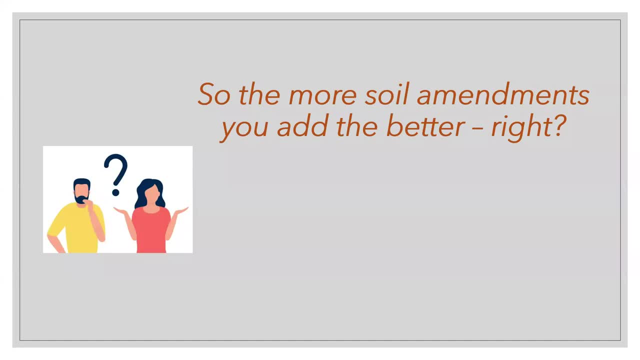 So we just, the more soil amendments you add, the better right, Like you know, just kind of in this case, hedge your bets, increase the soil as much as you can, and then you'll have the best healthy plants. But unfortunately it doesn't really always work that way. 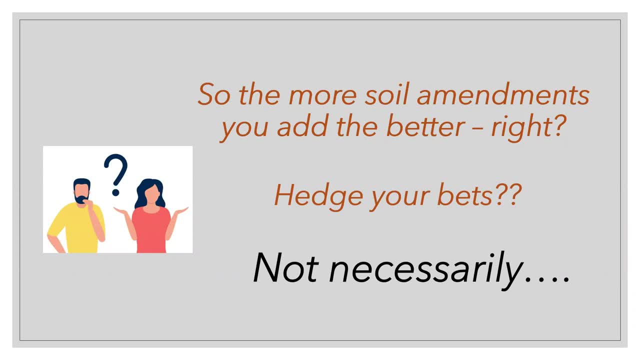 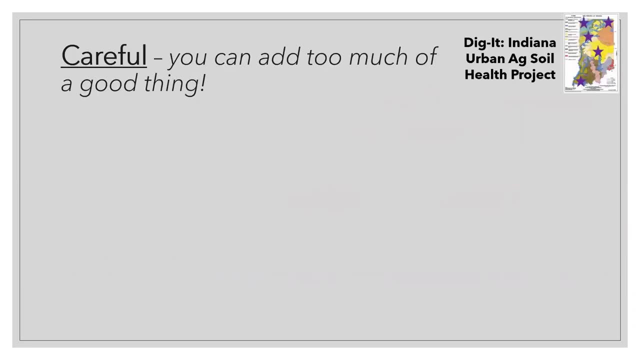 And so it's important also just to think and moderate, And moderate the amounts that you're actually adding to soil, And we'll talk about why. So, first of all, you need to be careful, because you can add too much of a good thing. 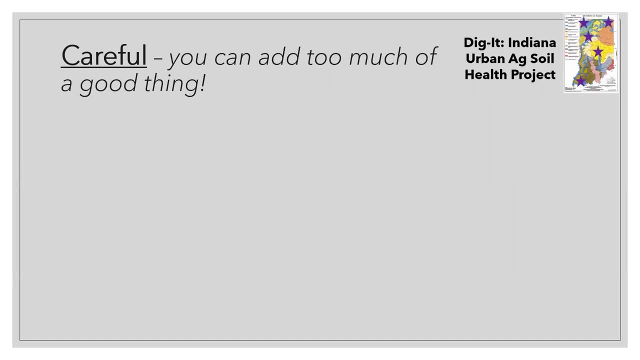 And this is something that I think we have seen through this project, where we've been working with all these growers across the state and trying to understand how people are managing their soils in urban ag systems- using a lot of amendments in many cases. So, of course, we've seen positive trends. 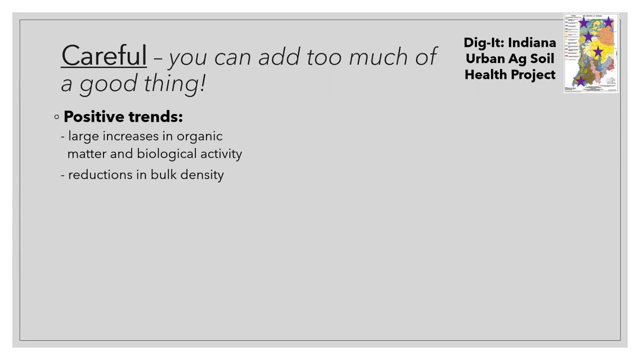 Things like large, dramatic increases in organic matter and biological activity- as people are adding lots of amendments- Reductions in soil bulk density, which is great. You know roots can move through the system more easily. You have space for nutrients and water too. 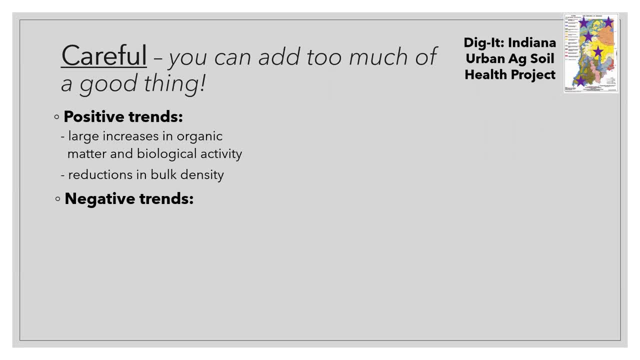 But unfortunately we're also seeing some negative trends associated with so much Of these soil amendments being added on some of these urban farms. For example, we've actually seen several farms where there's a decrease in wet aggregate stability because there's the soil is just so high in organic matter. 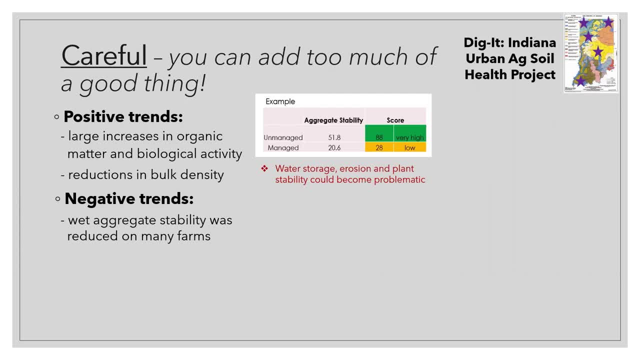 There's not enough of mineral particles to really start to bind and create natural soil aggregates, And so this can potentially make soils more productive. Soil is more prone or less prone to water storage, more prone to erosion, and plant stability within those soils can become a problem. 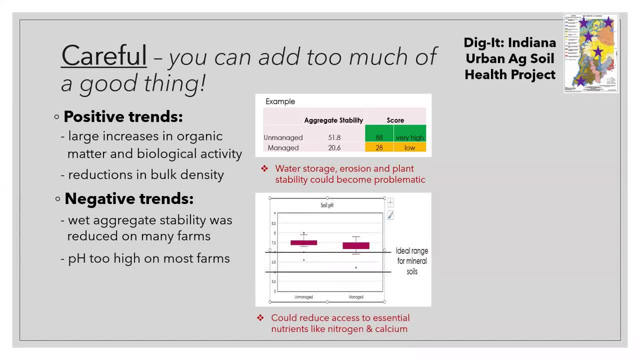 We also see that on most farms the pH is generally too high. So, as I said, you know, raising pH is important to reduce heavy metal bioavailability, But if you get too high then that can actually interfere with the uptake of other substances. 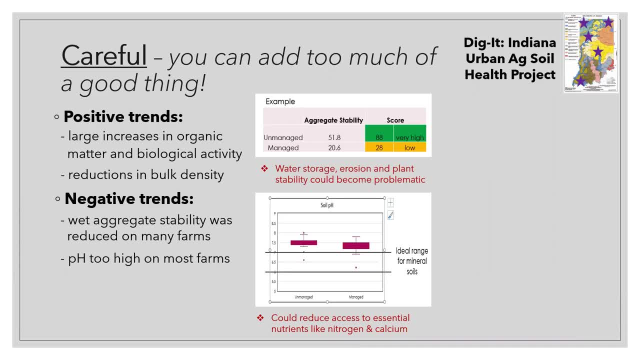 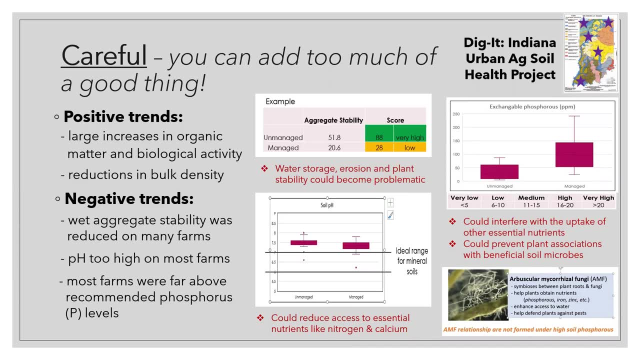 Other essential nutrients in the plant system. And then most farms were far, far above recommended levels for soil phosphorus. So phosphorus is an important element that plants need, But when you get too much in the system you can be prone to water quality problems. But it can also interfere with proper uptake of other essential nutrients And we know it can prevent plant associations with certain beneficial microbes, like our muscular mycorrhizal fungi, which help plants get nutrients, as well as other things like helping them suppress pests and deal with water. 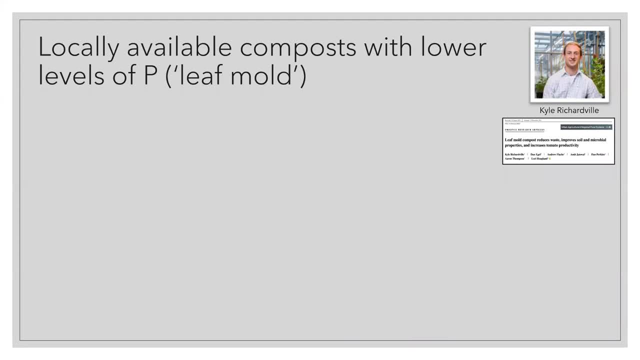 So we've also been doing studies to say, OK, how, how can we kind of manage some of this? What are ways we can think about kind of better, you know building the soil without you know running into it? So we've also been doing studies to say, OK, how how can we kind of manage some of this? What are ways we can think about kind of better, you know building the soil without you know running into it? 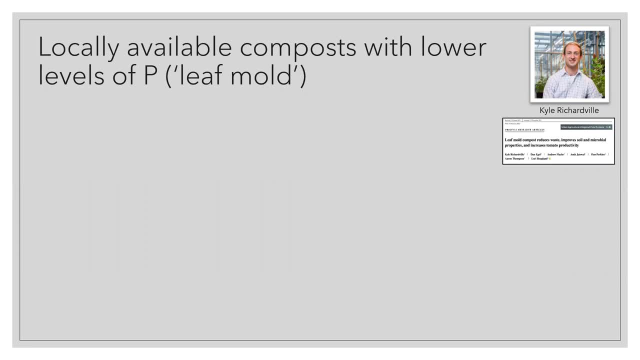 So we've also been doing studies to say, OK, how, how can we kind of manage some of this, What are ways we can think about kind of better, you know, running into some of these problems. And so again, going back, soil tests are really important, not just in the beginning. 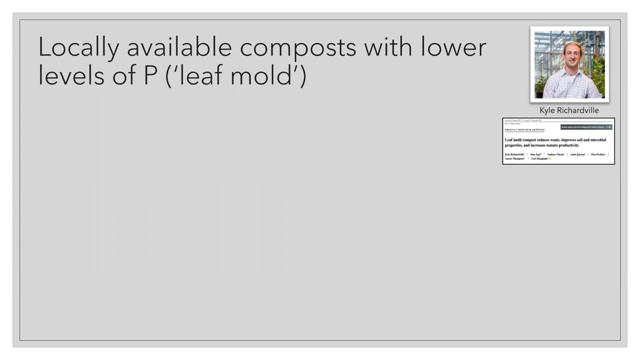 but over time to really see how your soils are changing and if you're starting to cross some of those critical thresholds. So we're also investigating: are there other amendments that we can use that will have benefits but maybe not run into some of the problems. 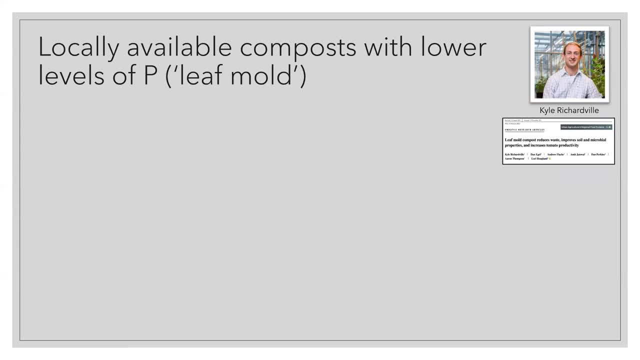 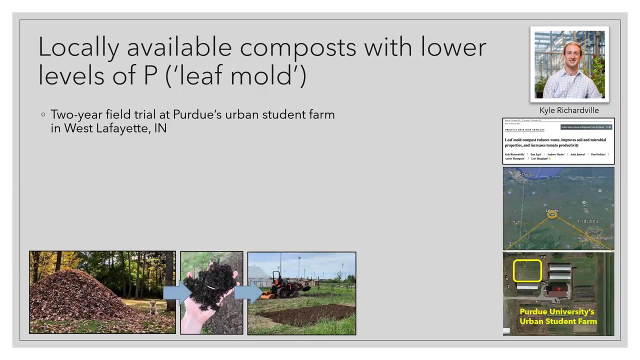 And so, in this case, this was a student who graduated recently, Kyle Richardville, who did a study investigating leaf mold compost, which has lower levels of P relative to some other composts that are made from, say, animal manures, And so he did a two year study at our urban farm here in West Lafayette, which, if you don't know where we are, this is Chicago. 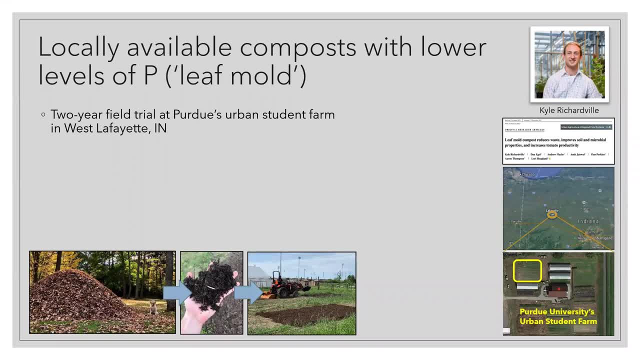 We're right down here- And this is an amendment that's commonly available in many urban systems. It's kind of a passive compost process. It's thought to generate more fungal dominated and higher C to N ratio composts, And so we were interested. The farmer we were working with was producing this and reporting a lot of great benefits. 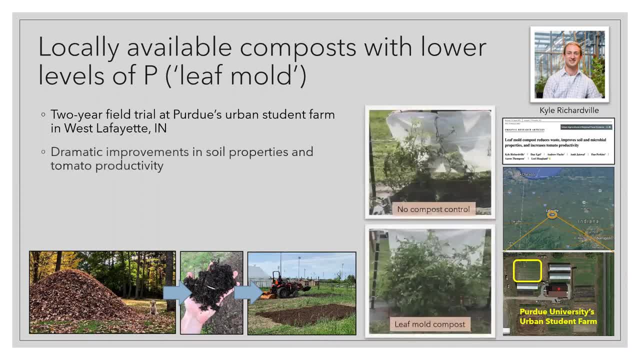 And so Kyle did a study, He applied this, Of course, he saw dramatic improvements in soil properties. So the soils at the site were pretty degraded after tilling, you know, leveling the site and making it available For our student farm. And so you know, it wasn't a surprise. 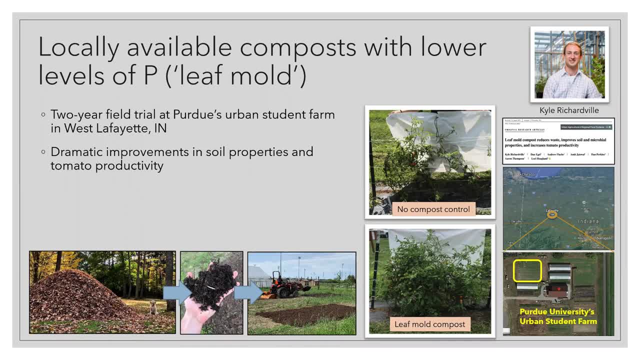 He saw really nice increases in both soil properties as well as plant health, tomato health. He also observed increased populations of beneficial microbes with pathogen suppressive capabilities near the tomato roots, And he also saw that this particular amendment was better at helping support a beneficial fungal inoculant, Trichoderma harzianum. 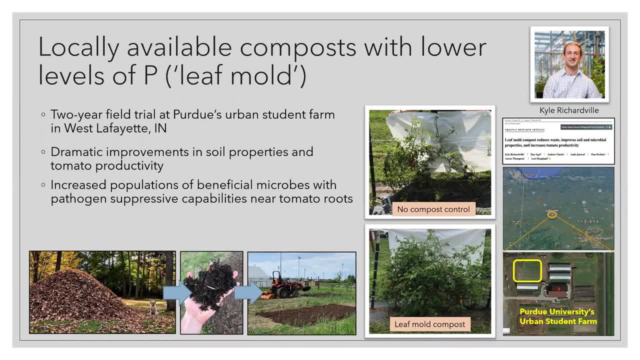 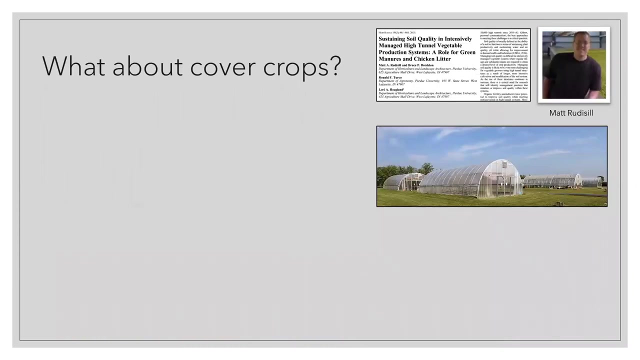 that can also help. That can also help plants to fight pathogens, And he observed reduced incidence and severity of foliar diseases in the tomato plants, while reducing the buildup of soil phosphorus relative to what we've seen with other common amendments, especially those derived from animal manures. 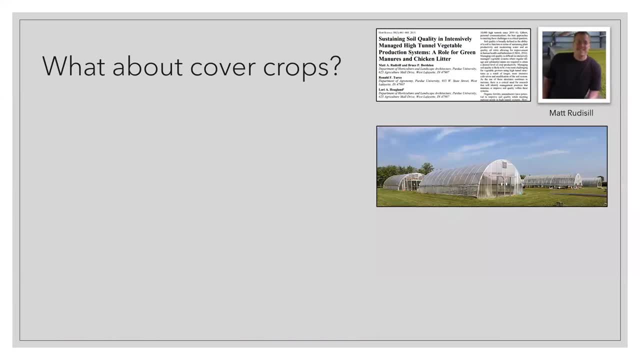 So another way to build soil health- It might take a little bit longer But, you know, can avoid Some of the challenges associated with things like phosphorus buildup- is just using cover crops, And so this is a study that was done a few years back by one of my students, Matt Rudisill, who was looking at in high tunnels, which are very popular in our region. 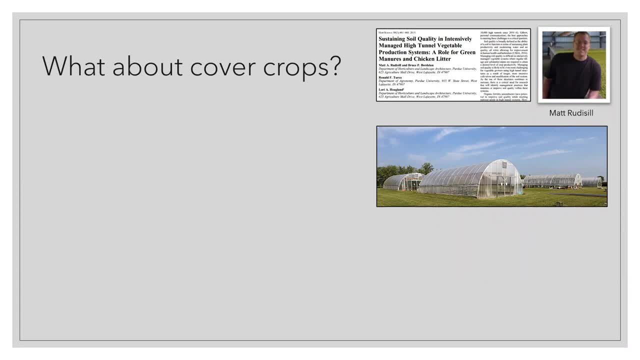 And wondering, you know, is there, can we? first of all, he wanted to know, can? is it possible to meet plant nutrient needs while also improving soil health and avoiding pea accumulation, Using more green manures- a vetch, in this case, amended with some alfalfa- versus the more traditional animal based composts? 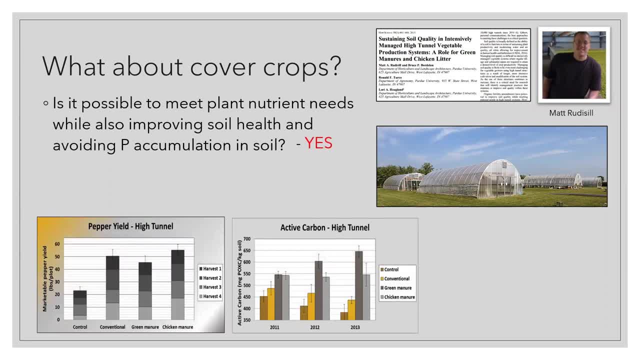 And so he saw that, yes, growing pepper, this is yeah, over. this is only one year, but this is in year three. He had repeated applications that the green manure maintained yield, as well as the chicken manure and a conventional fertilizer. 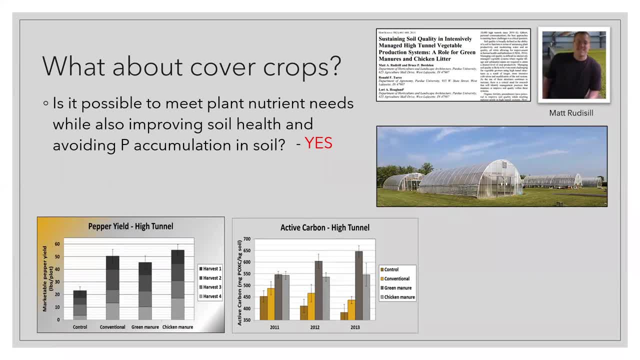 So much better than the conventional fertilizer. Yeah, So he had control with no fertilizer, But also really nice increases over time in the health of the soil, And so this is active carbon And this is the green manure on the right where he saw really nice buildup in soil health. 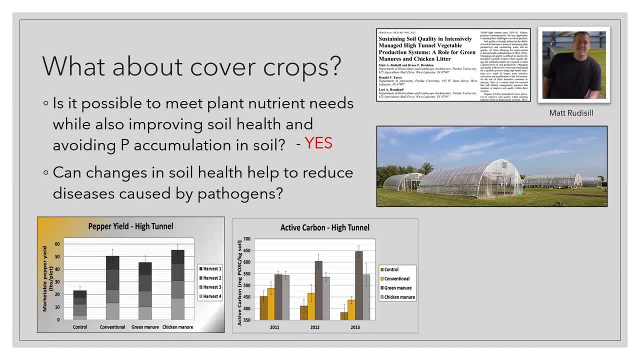 So next we wanted to follow up on that and say: can changes in soil help help to reduce diseases caused by these pathogens? And so we took soils from those plots after three years Again amended them With a soil borne pathogen Rhizoctonia and did our bean assay and saw that actually this soil that we saw that was the healthiest from this more green manure based treatment was the best at suppressing pathogens and helping the plants grow in this system. 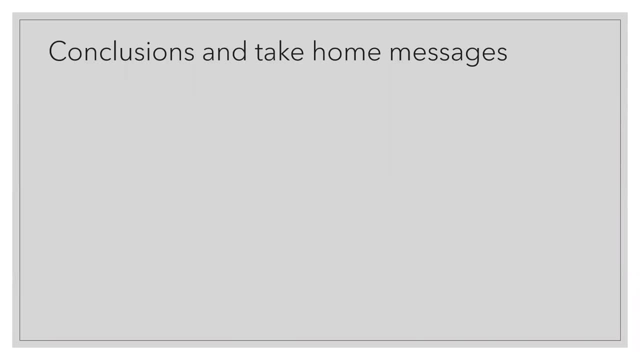 So some conclusions and take home messages from all of this around amendments: First of all, always start with a comprehensive soil health test To know the status of your soils, and repeat, Identify soil amendments based on your specific needs, what you're interested in. 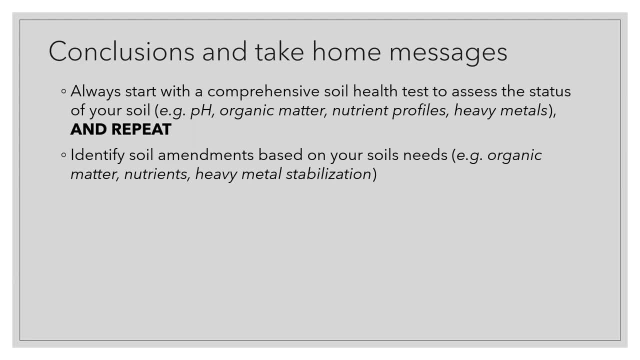 And again your extension. educators and folks at soil and water conservation district and an RCS can help you with that. Think about testing your compost. So some compost potentially in urban environments could be contaminated. Most companies are testing them at this point, But just make sure you think about that. 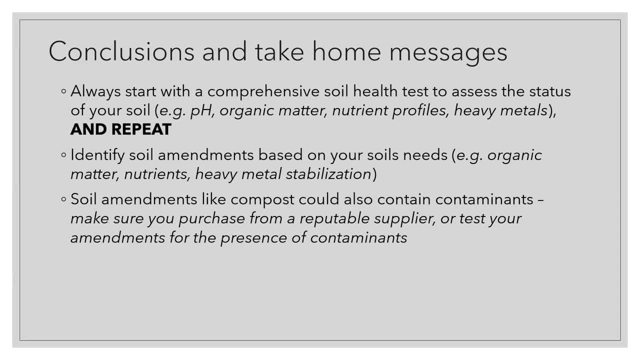 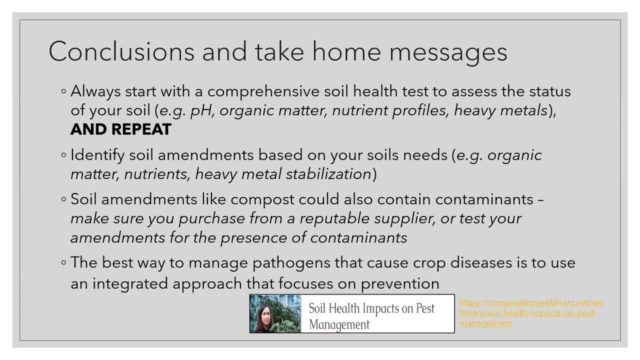 When you're, you know, thinking about what to choose And then again just driving home while you know. we know soil health is important And it's part of a sustainable management plan. It's only one tool in your toolbox. 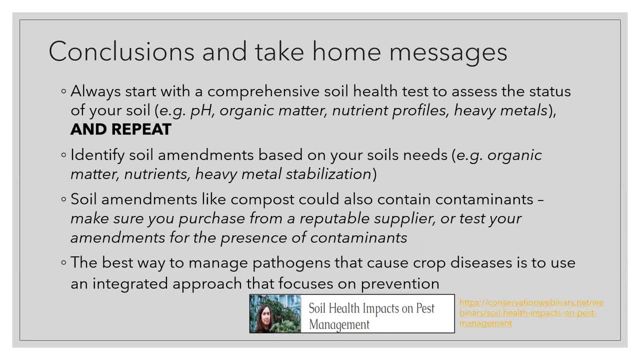 So always use multiple approaches to think about mitigating heavy metals and with pathogens, Really think about that prevention, And so we didn't have time to talk a lot about this, But this is another webinar that's available on eOrganic that I did a few years ago that talks more about different ways to manage pests. 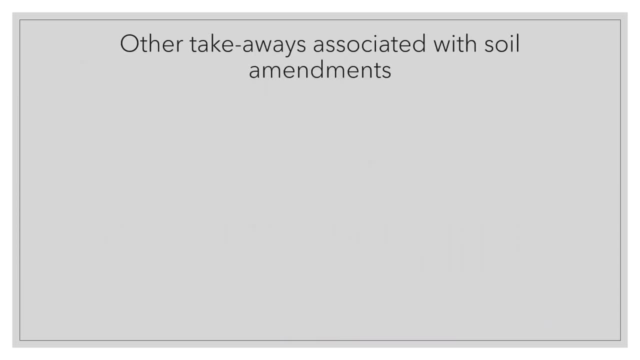 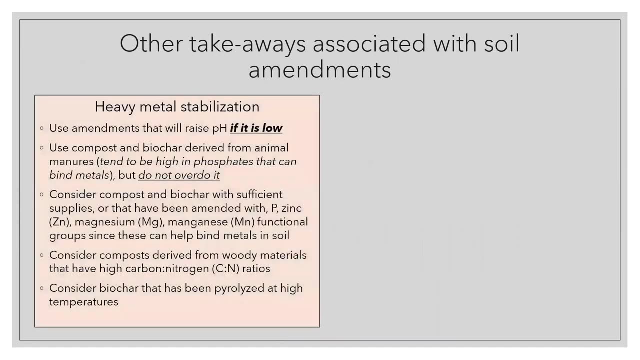 So quickly. I'm not moving very fast here. I want to just- you can come back and look to this because it's a lot of information- But just some other takeaways in terms of heavy metal stabilization and kind of summarizing the literature, what we know. 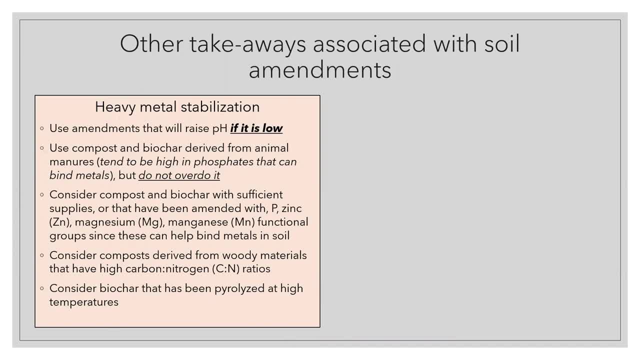 You know, raising pH again if it's low. important Using wastes that have, in this case, animal manures, because things like phosphate can help to bind metals, But don't overdo it. Consider composts and amendments that are also perhaps enriched with other things like phosphorus, zinc, manganese and magnesium. 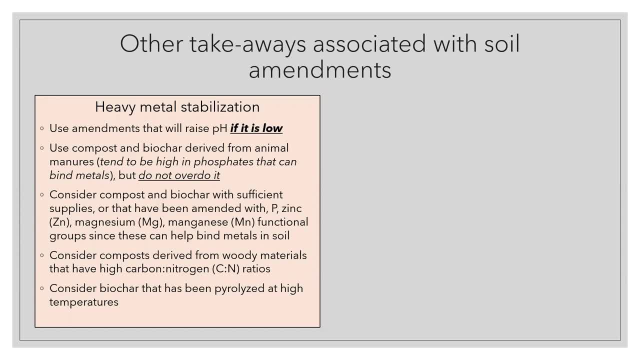 Because these have been shown to be good at binding metals. Then also wastes with high C2N4. And then, of course, you know we're going to talk a little bit more about that, But those with high C2N4 ratios and biochars that have been pyrolyzed at very high temperatures. 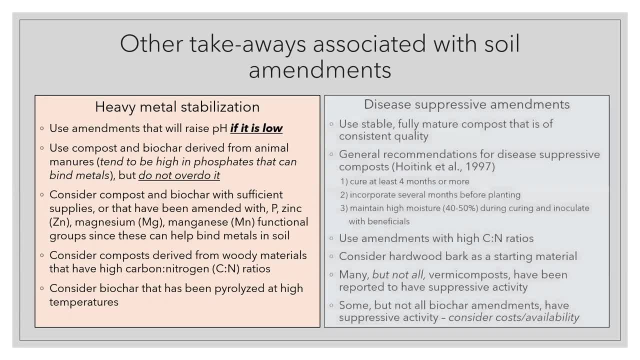 Those tend to be better at binding metals, And then, on the compost side, always use stable, fully mature compost that's of consistent quality and has been properly cooked so you're not moving pathogens through the system. It's a great review article. It's a little bit older but it still has lots of great information covering work that Harry Hoytink did over in Ohio. 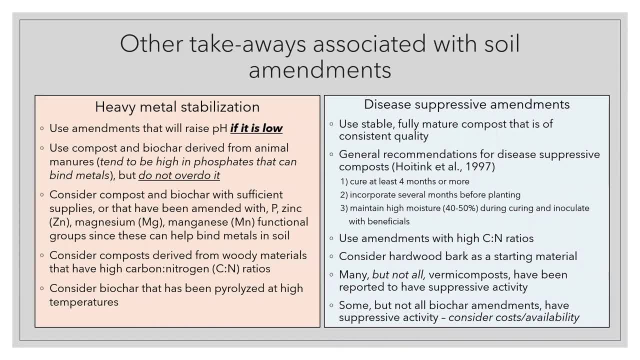 A few years back about potentially what could make compost more pathogen suppressive. He talked about ones that have been cured for longer time periods, maintained high moisture and perhaps inoculated with beneficials- Some other things that we've seen. amendments that have higher C2N ratios tend to be a little bit better in pathogen suppressiveness. 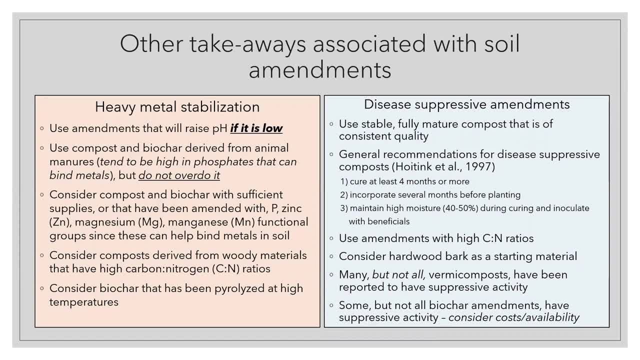 Things with hardwood bark And then vermicompost. We've seen some variability there, but across our studies vermicomposts have been a little bit more pathogen suppressive than some other composts. And with biochar, you know, just consider costs and availability because it is more expensive than some other composts. 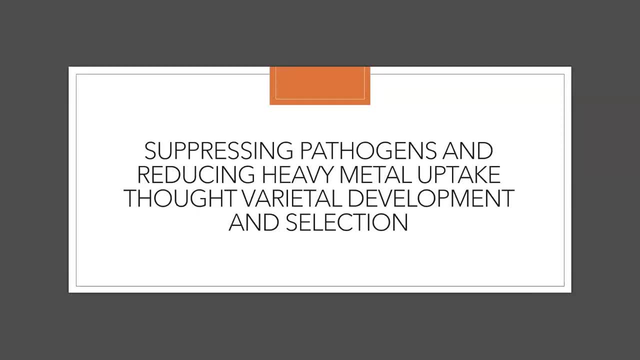 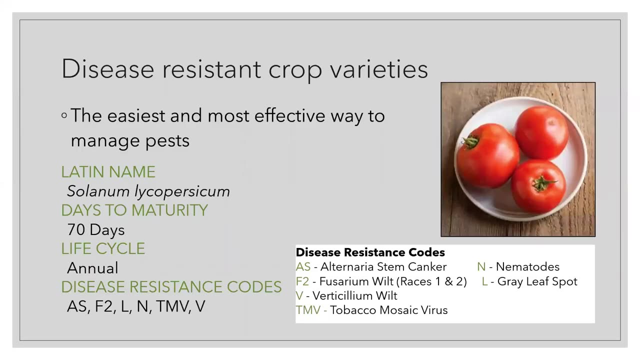 Okay, now we're going to switch to kind of the other side, What we've been doing with thinking about- you know how- also using plants, How to suppress pathogens as well as prevent heavy metal uptake. So, first of all, one of the most effective and easiest ways to prevent diseases, if there are resistant varieties available, is to use disease resistant varieties. 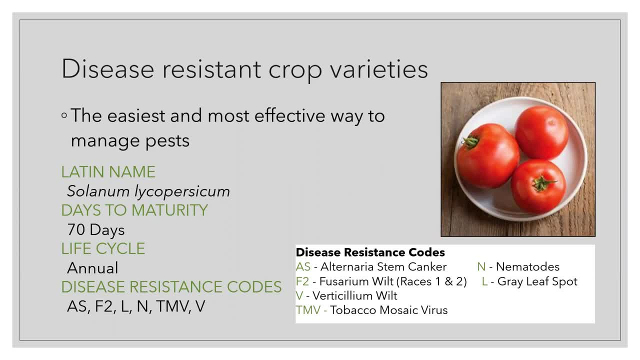 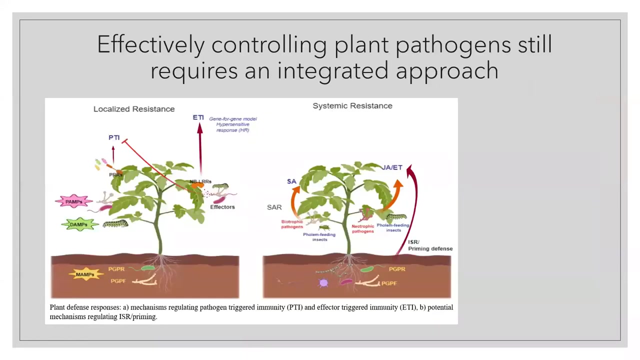 Like in this case, this particular tomato variety is resistant. It has genes been bred to have, genes that provide resistance. Strong resistance, kind of you know, stops the pathogen in its tracks to control many of these problematic pathogens. So, however, it's always you know, we know that effectively controlling plant pathogens still requires an integrated approach. 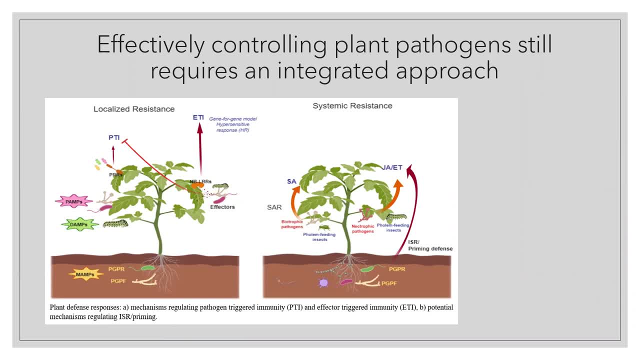 So, unfortunately, pathogens can evolve over time to overcome the resistance Confirmed. There's a lot of resistance conferred by a lot of these single resistance genes. So one of the things that we've been, you know, working on is what are other ways we can develop plants that maybe have a broader set of ways to fight pathogens? 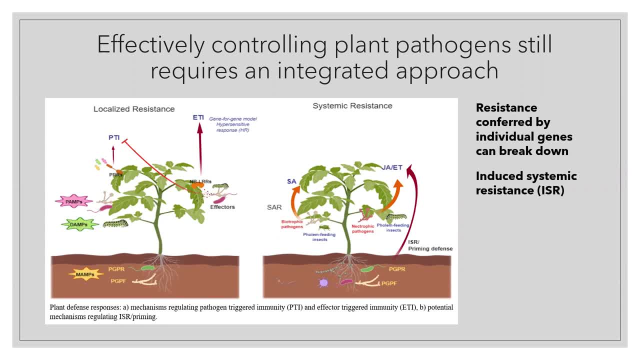 And so, again, we've been working with this phenomenon- induced systemic resistance- where beneficial microbes help plants to mount a stronger and more effective response against the pathogen. And so you know, we know, that this is part of this connection between soil and plant health. 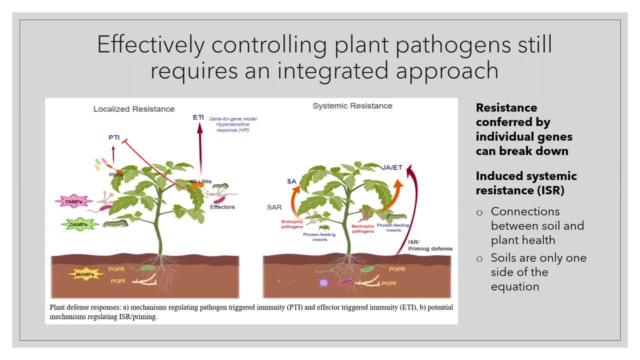 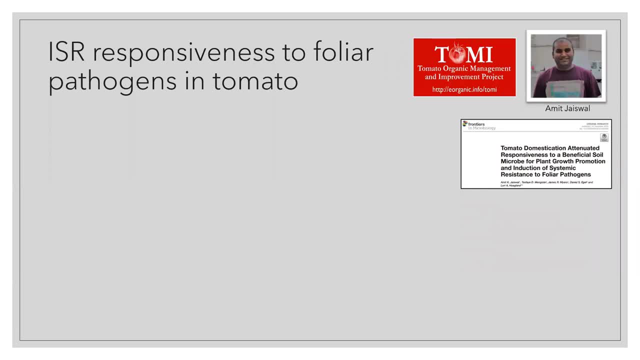 But soils are actually only one side of the equation. So you can make soils really healthy, but you also need to make sure you have responsive partners, And so that is one of the aspects we've been studying in the tomato organic management and improvement project. 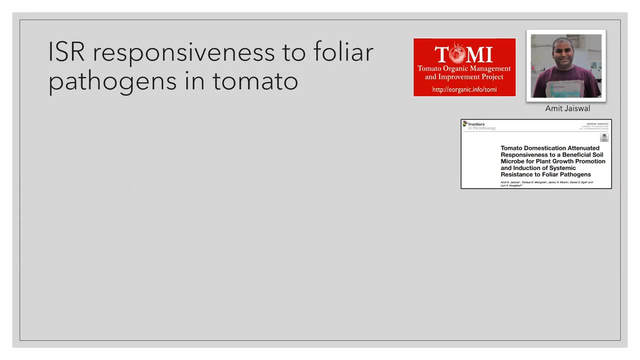 Project is this learning model. It's this learning more about responsiveness among genotypes to foliar pathogens in tomato And can we learn more about this so we can actually start to breed for it. And so this is Amit Jaiswal, who did a lot of work in this area. 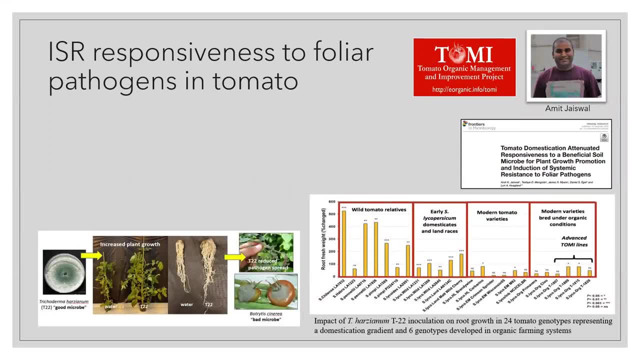 And so he started with just looking at this whole collection of genotypes over domestication. So from the wild tomatoes down to more modern varieties And then varieties that you know we're going to be looking at, And then varieties that both our program has been developing, trying through organic breeding projects and some other tomatoes from organic breeding projects in other locations. 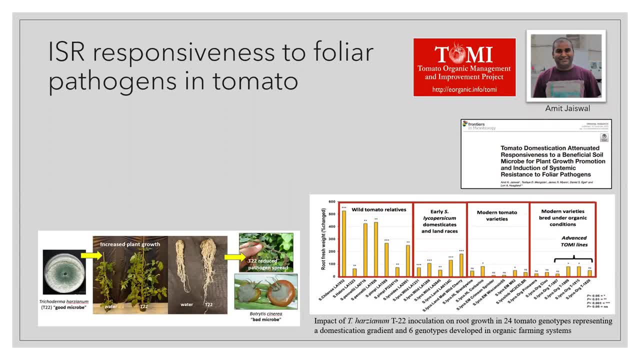 And so he saw big variability both in how the tomato genotypes were responding to this beneficial microbe- in this case Trichoderma- This figure here is around growth- and also responsiveness to this induced systemic resistance against both phytophthora. 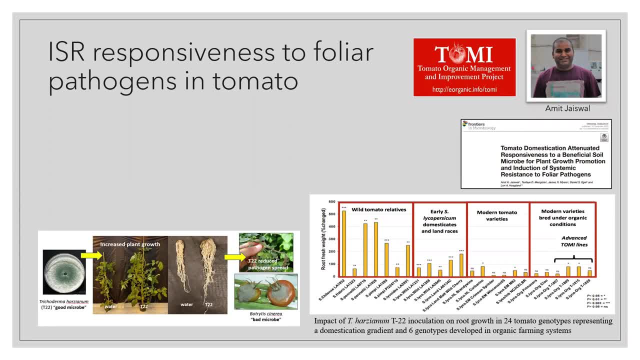 infestans and Alternaria solanae And so just some things. we saw this kind of unfortunately decline over time And that is we've domesticated plants. They seem to have lost this capability to really support these beneficials. But we do see a slight increase in kind of reversing that trend when we've been selecting within organic production systems. 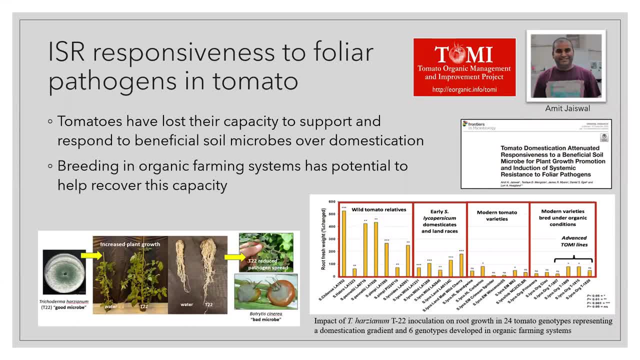 And so we've seen this step in the right direction, And so we have a lot more work to do to really to get this into your hands, so to speak, And we've been doing a lot of efforts. We're working with Julie Dawson now to see how well our efforts are paying off. 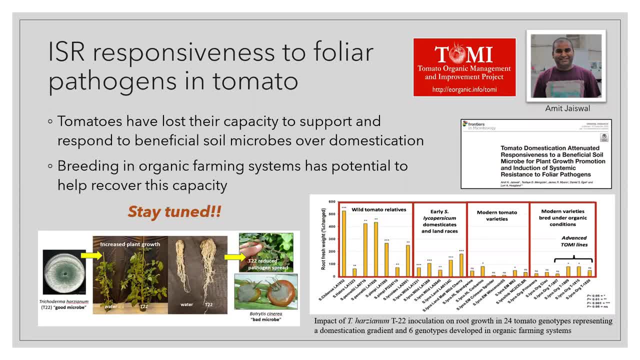 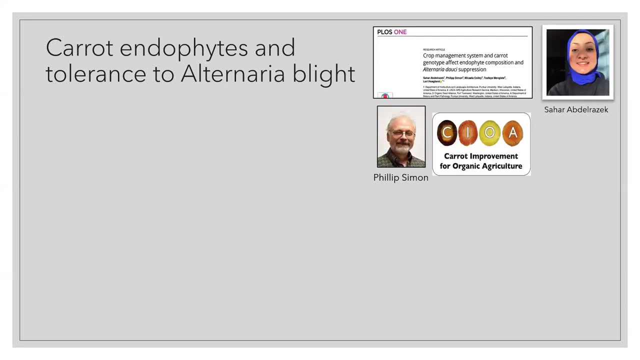 Can we actually start to select for this and advance it. So stay tuned. We're not there yet, but this is something we're continuing to work on and hope to have in your hands soon. So same, similarly, with the Carrot Improvement for Organic Agriculture Project, which is led by Dr 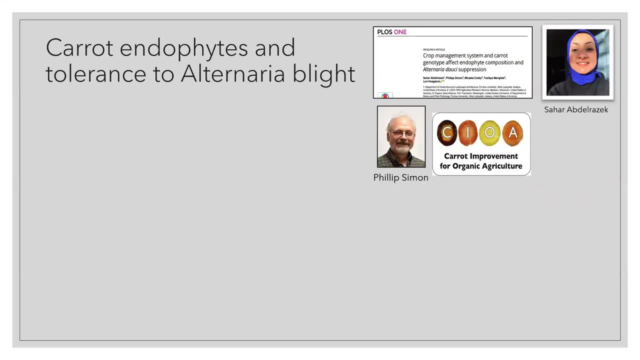 Phil Simon. He's with the ARS up in Madison, Wisconsin. We've been working to see can we find new ways to enhance pathogen resistance and bring that into breeding programs, And so this former student, Sahar Abdel Razek, was working on that. 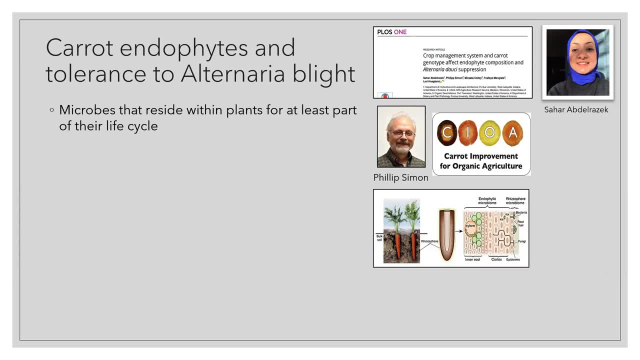 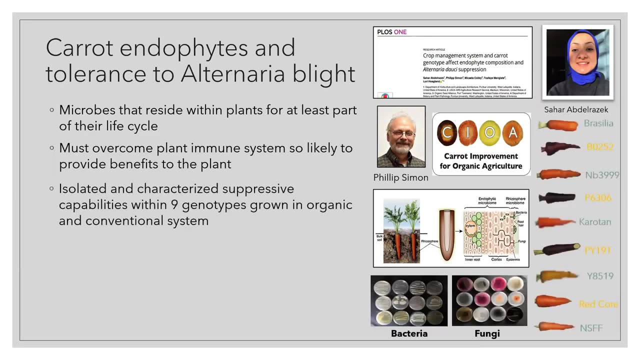 And she was really interested in endophytes, which are microbes that live with animals. They live with inside plant roots, And so we think these have a very close relationship with the plant, so they could be better targets to breed for, And so she did a study where she isolated and characterized the suppressive capabilities. 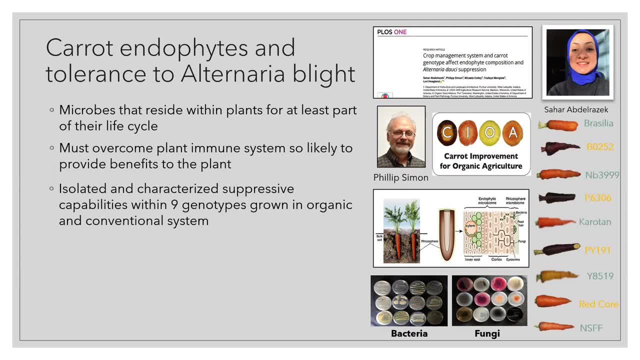 pathogen suppressive capabilities of all of these endophytes, bacteria and fungi you see here and these nine different genotypes grown in organic and conventional systems. And so she saw the endophytes were more suppressive against Alternaria dowsi when tomatoes were grown in organic. 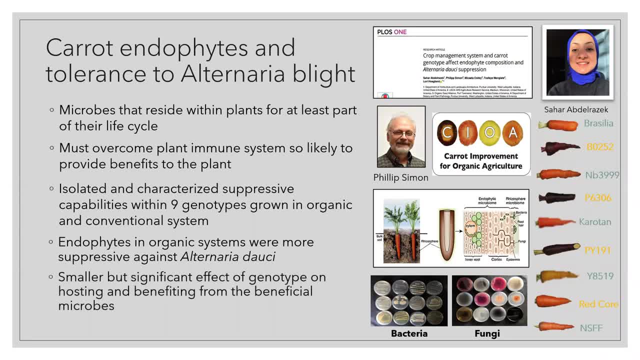 So that correlated with differences in soil health And there was a smaller but yet significant effective genotype on hosting and benefiting from these beneficial microbes. So again, we're still working on this, So stay tuned, But we do think within the next year or two within CIOA. 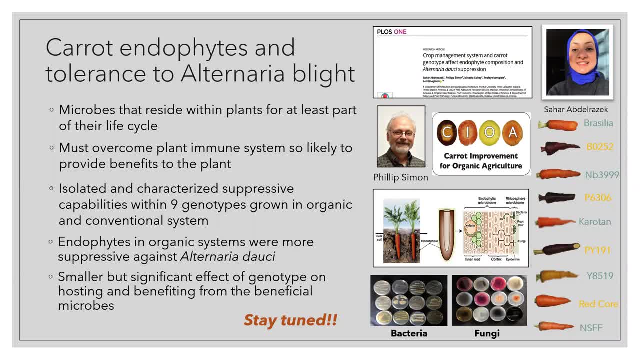 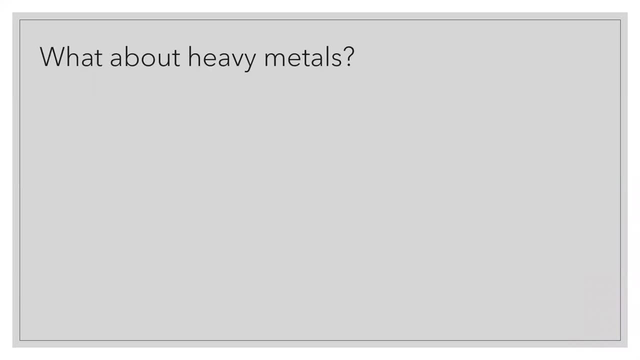 we will be releasing some new, improved varieties That you can use that have better pathogen resistance and also better nutritional quality. So what about heavy metals? This is kind of a newer area for us and, like the breeding, you know, breeding is a long term strategy. 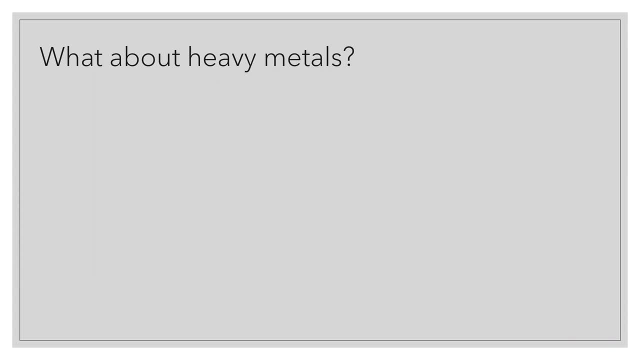 So you know we're just really getting going with this, But I just wanted to point out that we do know many crop genotypes and varieties do vary in their potential to take Up heavy metals. So in rice there's been many studies that have shown this and people have started to be working with that to select varieties that take up less heavy metals. 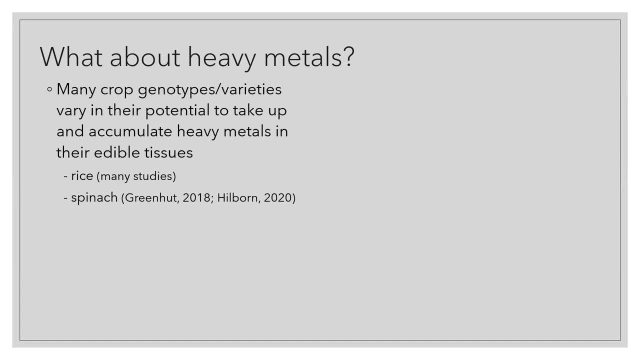 We know in spinach this has also been the case And the folks out at UC Davis- Charlie Brummer and Alan Van Dyson are doing- have started actually moving this forward, trying to select and understand the mechanisms here So you can have spinach with lower uptake. 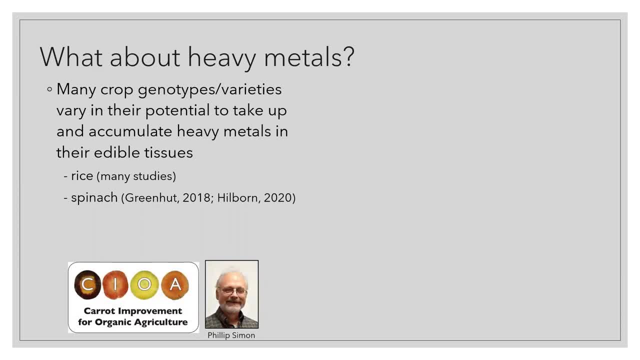 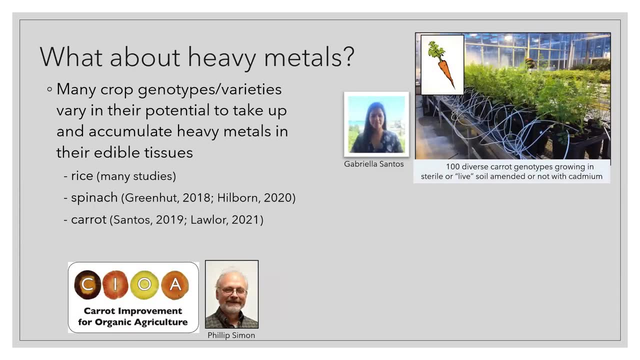 And we've also been interested in this with our carrot project, And so we started. we just went through and evaluated a very diverse set of carrot genotypes to see if we could identify ones that had lower uptake and lower and higher uptake. Phil and his former student, Aaron Lawler. 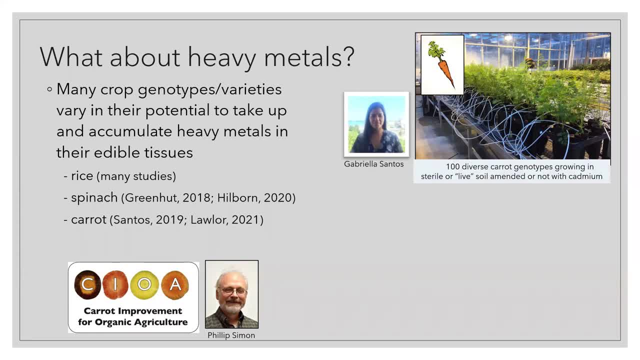 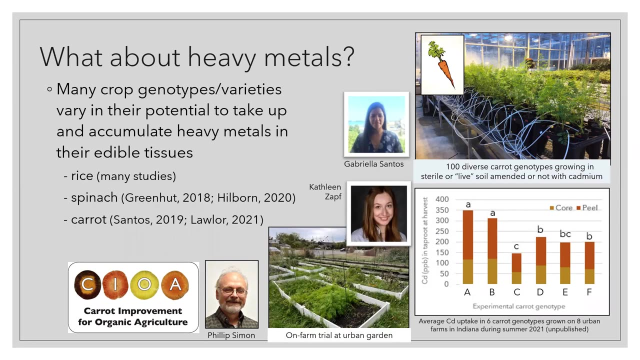 also did a very large study with many individuals to look at variation in uptake And we did observe differences in carrot And so we've been now following that through. This is Kathleen Zapp. We just finished her second year study of this, where we've taken some of those high and low carrot accumulators. 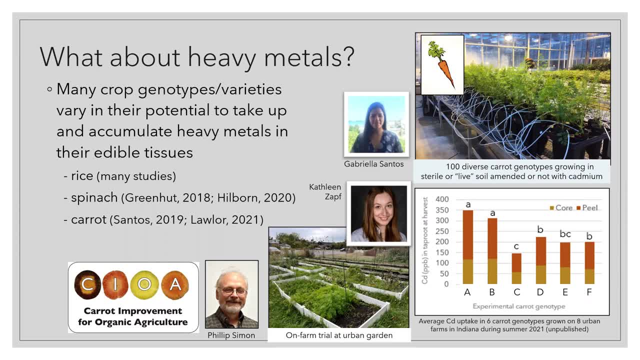 different genotypes and been growing them on a number of farms across Indiana that vary in soil properties and potential safety risks, And we are seeing that what soil is still a stronger factor. We do see some of this variability hold up in the field. 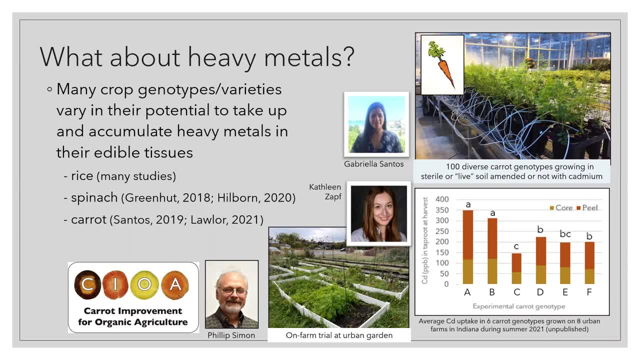 And so you can see here genotype C. this experimental carrot variety is much lower in uptake than A, And so, again, you need to stay tuned. We can't tell you today which varieties to plant, and we have a long way to really breeding for this. 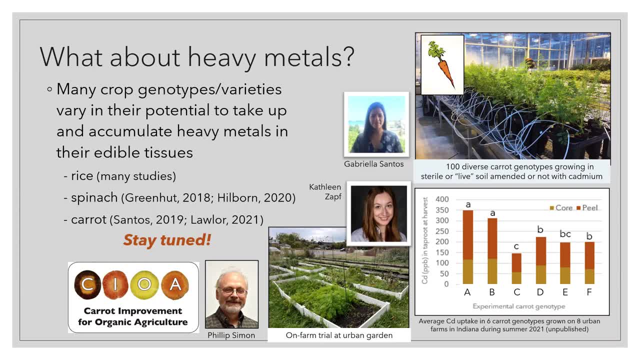 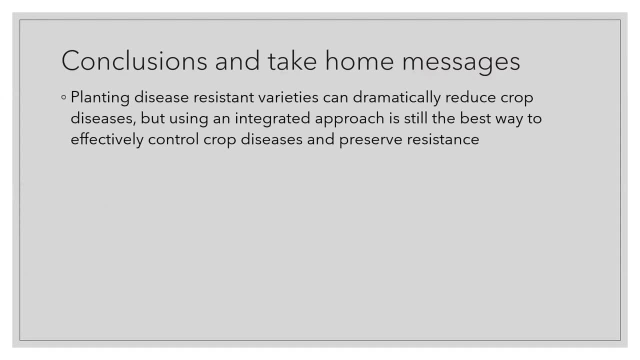 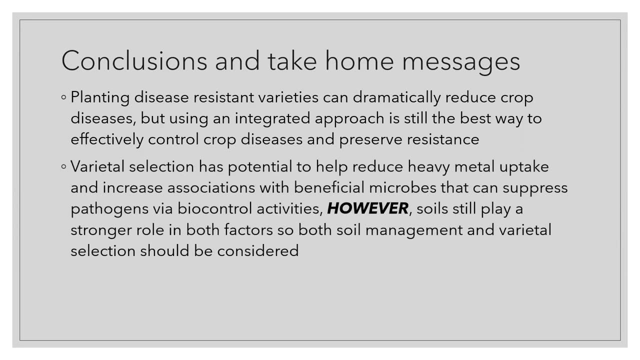 But we will be releasing some varieties soon. So some conclusions and take home Messages on this. you know planting disease resistant varieties can really reduce diseases, but an integrated approach is still the best way. Varietal selection does have potential to reduce heavy metal uptake, and increasing associations with microbes that can suppress pathogens can help. 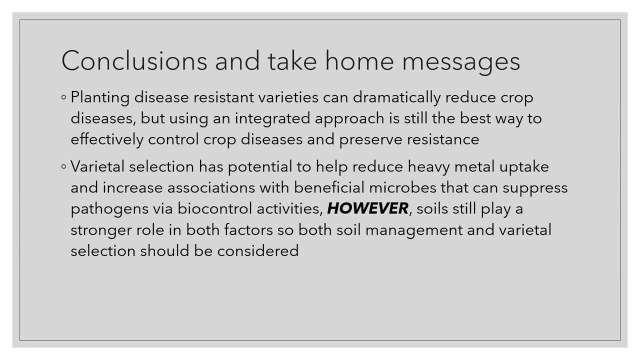 But soils still play a stronger role, So make sure you're always thinking about both soil health And varietal selection. And lastly, I just want to point out I love this figure because I think, in addition to showing differences in heavy metal uptake, 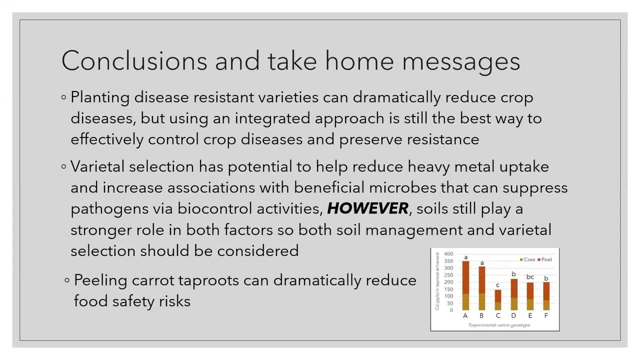 when you look at it, you can see that just simply peeling carrot roots can have a dramatic effect in reducing the danger of heavy metals, in this case cadmium. And so this is the darker orange, is the peel, And then the core itself is down here. 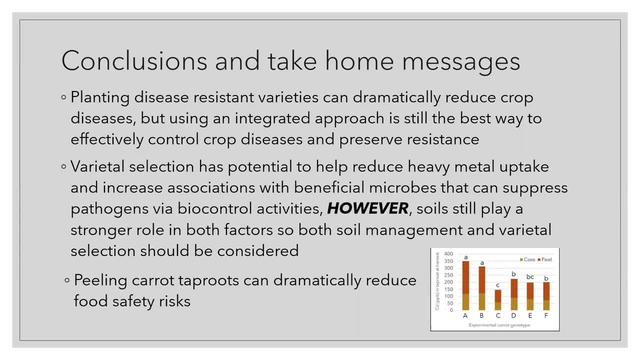 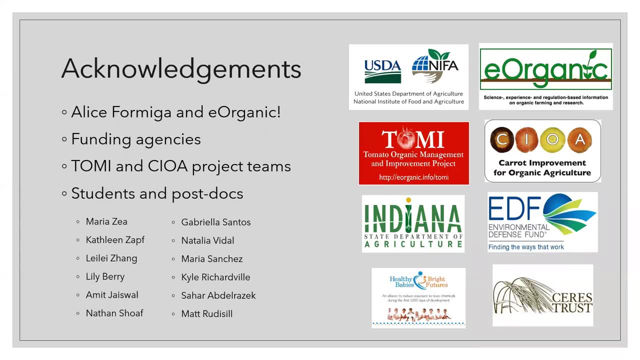 So always wash your produce and peel it. So just some quick acknowledgments. I really want to thank Alice and E Organic for hosting us, A lot of the funding agencies who funded our work over these years and many different students and postdocs that have contributed to this project. 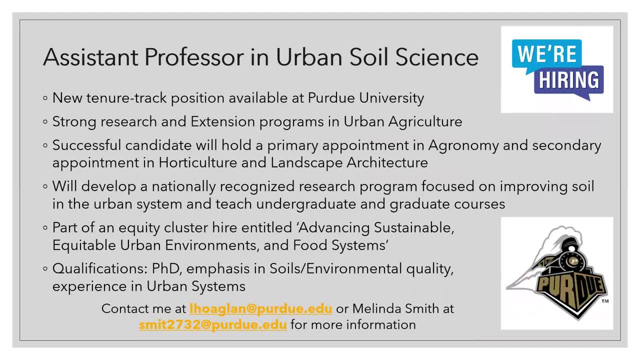 And then, lastly, I'm really excited to use this opportunity to help advertise For this new position that we recently got approved here at Purdue University. So we know urban agriculture is important and soils within cities are important for a whole number of reasons. 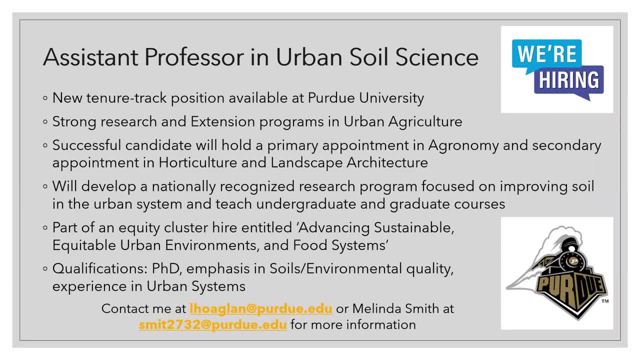 And so we are going to be hiring a new tenure track position in urban soil science. And, just to let you all know, Purdue has. we're located, you know, an area with lots of cities And we have a very strong both research as well as extension programs and urban agriculture. 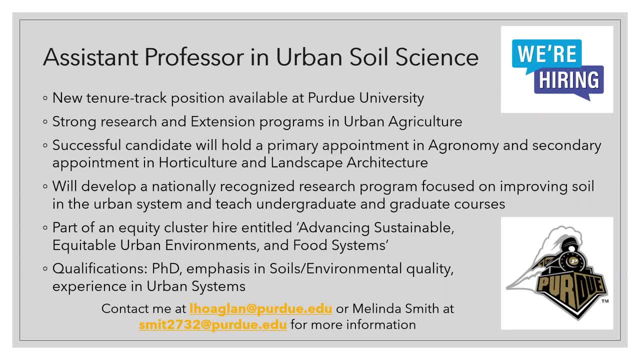 So you'll be joining a great team. This position would be jointly, mostly in agronomy, but also in my department, horticulture and landscape architecture. The position will be developing a research program around improving soils. You know, be great if they work with contaminants. 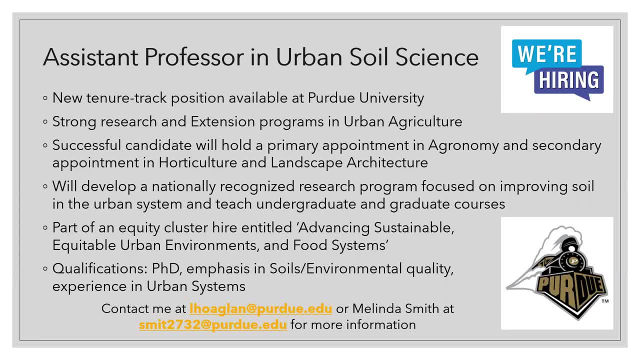 but there's all sorts of work to do Within cities is, in addition, also just working with local communities around restoring soils of teaching classes. This is part of an equity cluster hire here on advancing sustainable, equitable urban environments and food systems. So we're really appreciate your help and just getting this advertised widely as possible and through different channels. 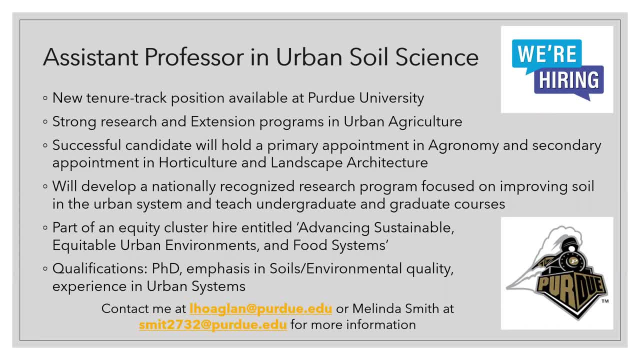 And we- we typically advertise in so we can make sure and get a very diverse and strong pool, And so if you're interested in this position, be sure you can reach out to me- I'm the chair of the search committee- or Melinda Smith for more information. 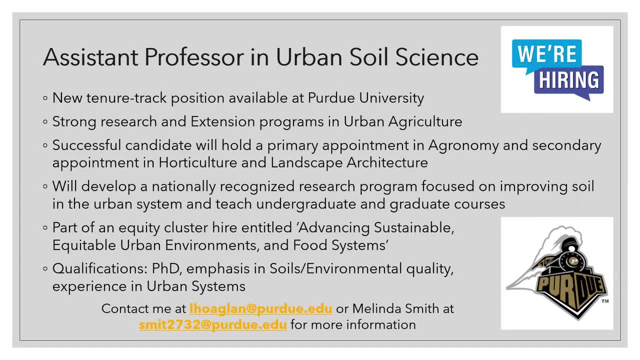 So with that I apologize, Alice. I think I went quite a bit over, but I thank you for your attention. Yeah, no, don't worry about that, But maybe you could just go back to the last slide, in case somebody wants to copy down that information. 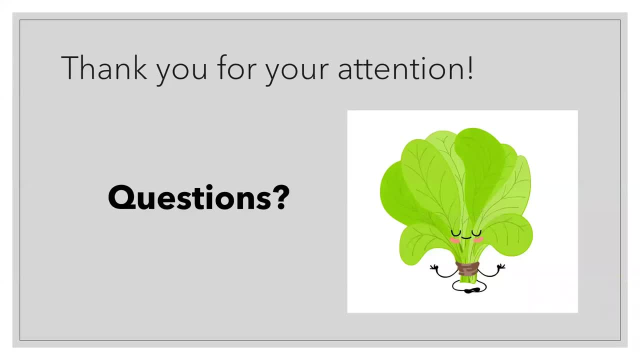 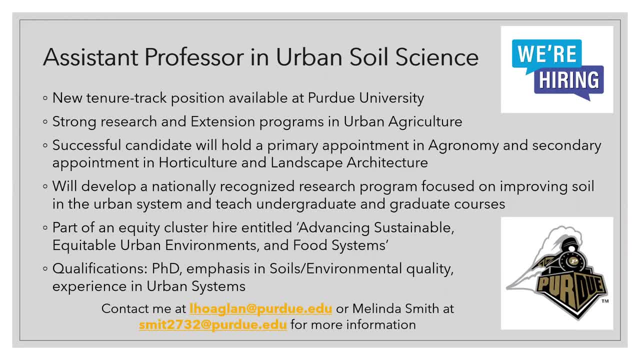 it's it. it's much in there and there's so much complexity as well, and we're about to start our Q&A, but I just wanted to remind everyone that we have one more webinar in this series next week on soil text testing. 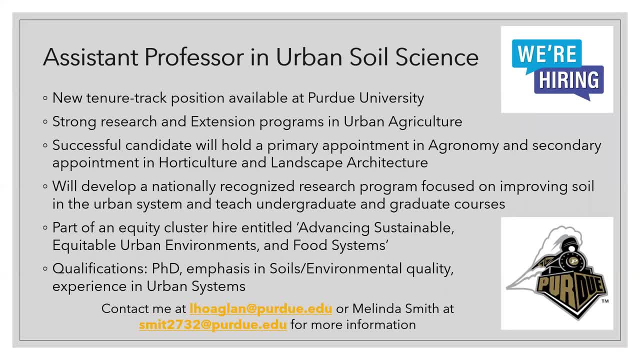 going into some depth about that by Roland Willhelm of Purdue and the recording of this webinar- in case you didn't absorb absolutely everything said and you want to check back on something- will be available within a week on the e cin万 00 거, as well as on the eOrganic web page. that lists all these webinars and we'd be grateful if you. 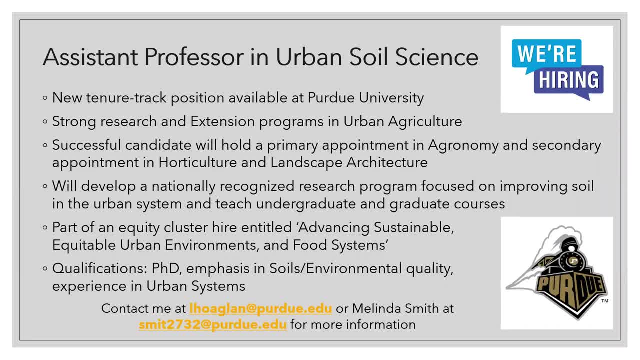 could fill out the email survey that you'll be receiving later today to follow up. But we do have a lively discussion going on in the chat and the Q&A and it was started well- the one in the chat- and there's a lot of different questions, but there's one that promoted some discussion about. 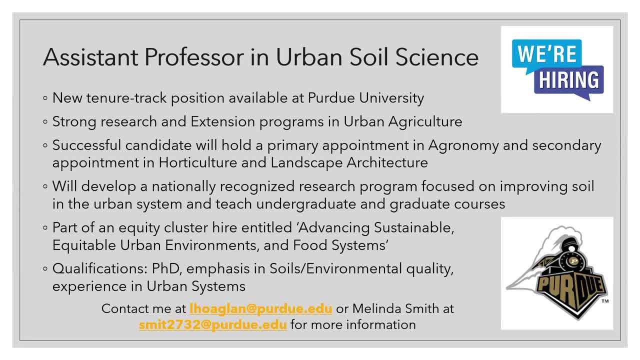 the cost of soil testing in general and then especially for heavy metals, because it really is expensive, especially for a lot of home gardeners, to conduct soil testing for heavy metals. So are there any ways that that could be made or any ways that people could get this done to minimize 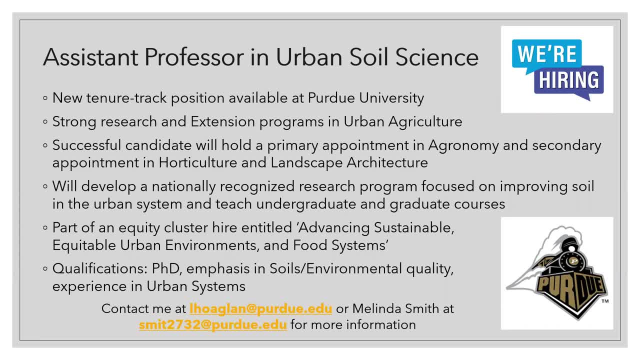 the expense? That is a great question and I wish I had a better answer for that and that's something we'll definitely. I'll ping Raleigh to make sure that he can investigate that a little bit next week and provide some better recommendations, because you're right, you know. 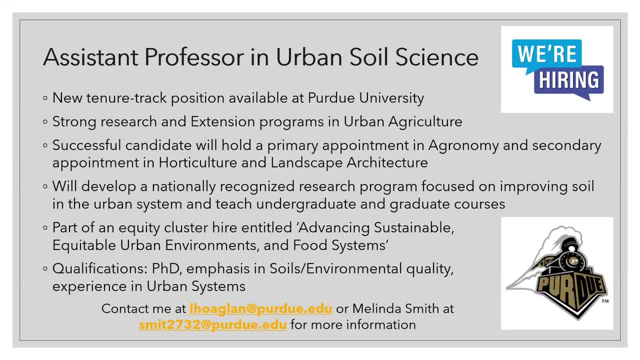 soil testing, especially soil testing for heavy metals, can be very expensive, especially if you're using the kind of most accurate technologies like ICP-MS. It can, you know, run $150,, for example, to test your soil Soil testing for heavy metals. However, I know there are programs across the country and many 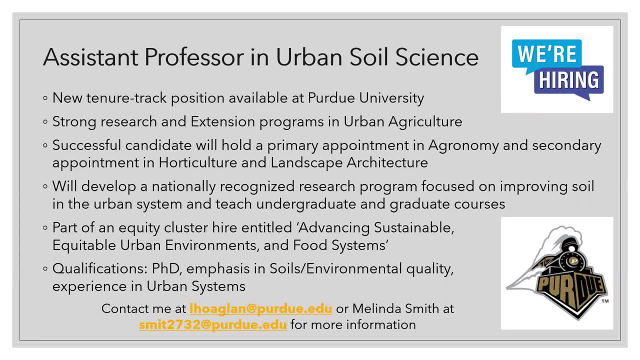 cities that are offering discounted testing for heavy metals. I know Chicago in the past has had a program where you can test your soils for lead for much cheaper. It's through a program at the university. I know our first speaker, Anna Paltseva, also provides some lower cost testing for. 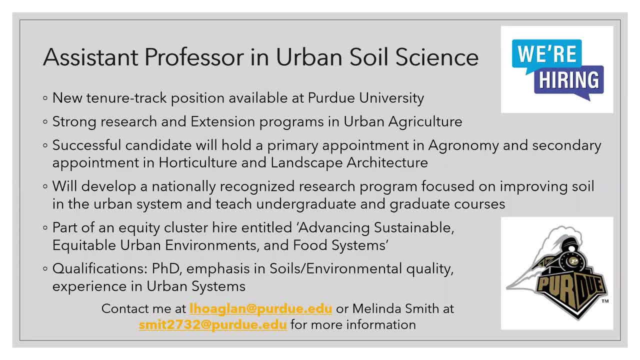 soil. She uses a different approach, XRF. that can more cost effectively, you know, monitor soils for heavy metals. So I apologize that I don't. I'm not aware of any programs like here in Indiana or other specific programs around the country that offer some of those cost savings. But yeah, I agree it can be expensive but it's very important, especially. 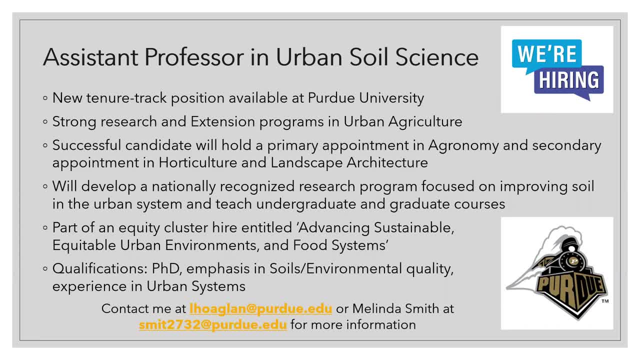 for people who are just starting in an urban Ag system to test your soils. Yeah, there was a question about a lab- interested in a lab that does cadmium testing in Minnesota- where Caleb said there's not a lot of affordable options So and the UMN soil testing lab doesn't offer tests for cadmium. so if anybody who's listening has any recommendations, feel free to post those. 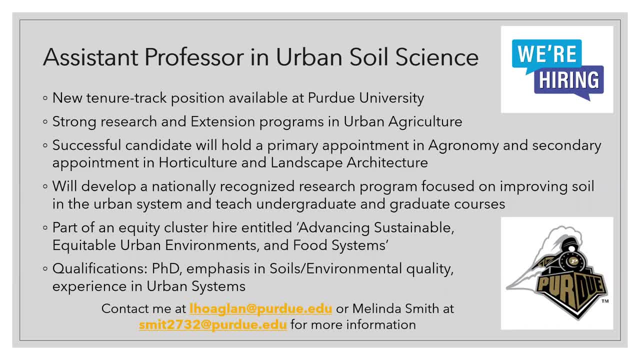 in the chat as well. if you don't know specifically, Lori, Yeah, I mean, I'd have to look it up. I know of a lab in Seattle that does really precise testing for cadmium, but it is expensive, Yeah. Yeah, that's a really good question and an important one, Let's see So. 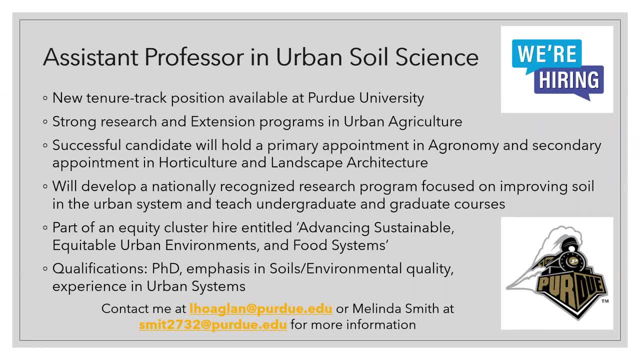 we have a bunch of other questions here too. Were the phosphorus levels in leaf mold lower than the phosphorus levels in compost produced using industry standards? Oh, okay, So that's an interesting question and I, you know, I don't know- off the top of my head, like of an actual 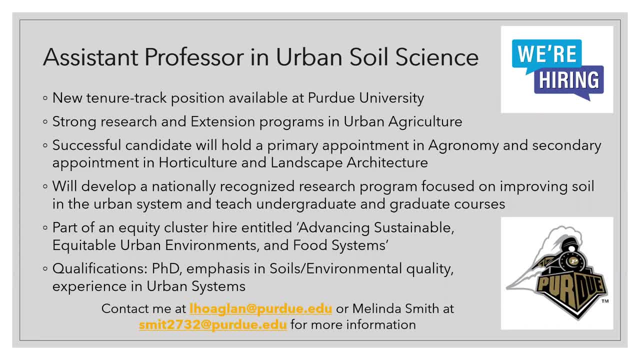 like industry standard for compost in general. You know what we see people are often the most using. are, you know, compost produced using industry standards? So I don't know if that's an interesting question. I don't know if that's an interesting question. I don't know if that's. 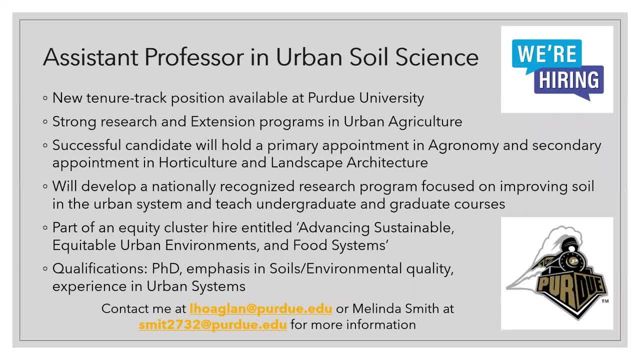 more animal compost derived from animals, and so those tend to have much, much higher levels of phosphorus relative to nitrogen compared to leaves. So the leaves- actually this leaf mold compost- had much lower like nitrogen-phosphorus ratios relative to most. 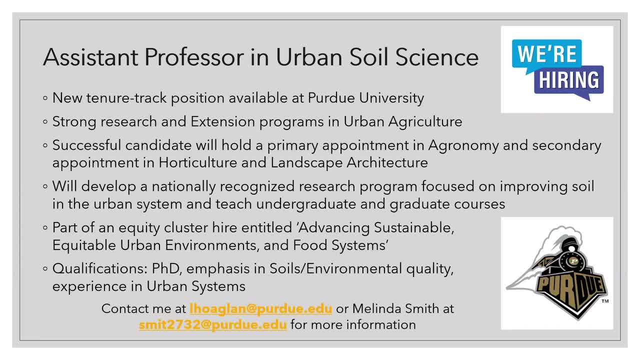 composts that we've seen, and that was one of the reasons why we were so interested in that. I'd have to look exactly how much lower it was, but yeah, that was why we were interested in it. Okay, Let's see. Have you used additional microbes from companies that sell them? 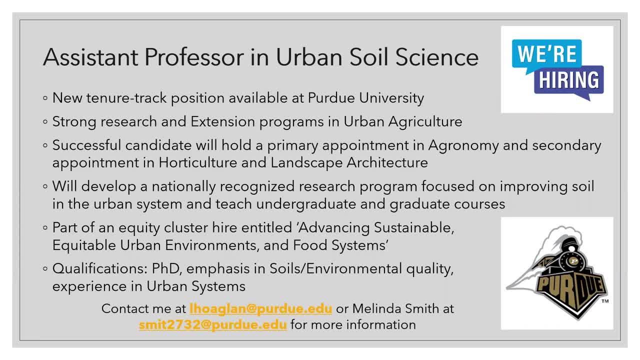 and if so, what did you add, from which company and did you see an increase in the microbial action? Yeah, So a question around microbial inoculants, and so that's something you know we haven't done a lot of in my lab because we're really 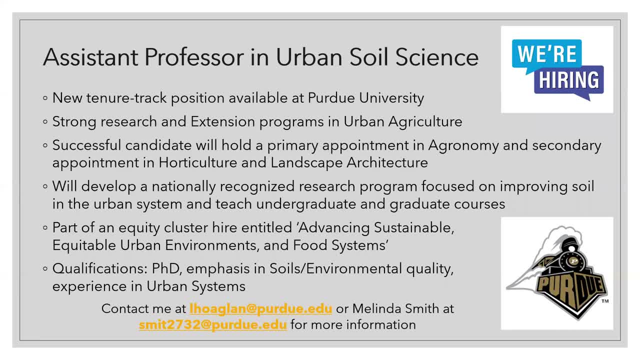 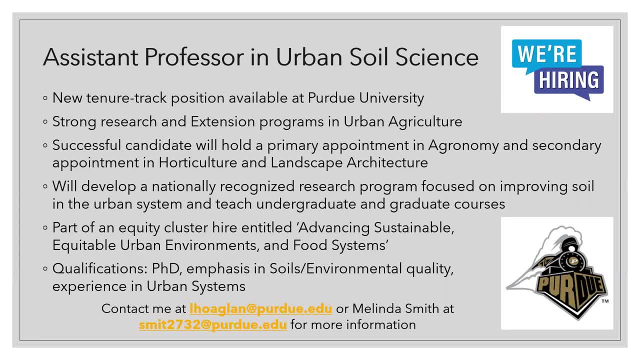 the compost, but we did inoculate the seedlings- or not- of tomatoes when they were going out into the field, and so we used a trichoderma harzianum T22 inoculant in that case that we used for a lot of our ISR studies, and it's Bioworks, I think, is the place that we initially, I know. 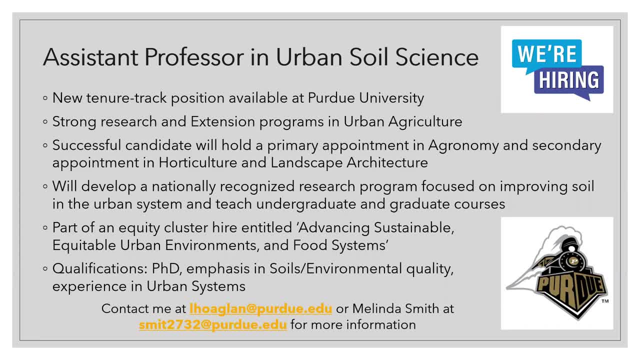 sells that. There are several companies that sell it and so in that case it was really interesting because we saw the amendment increase the survival. so the challenge with a lot of these microbial inoculants is when you go into a field system there's so much competition from the 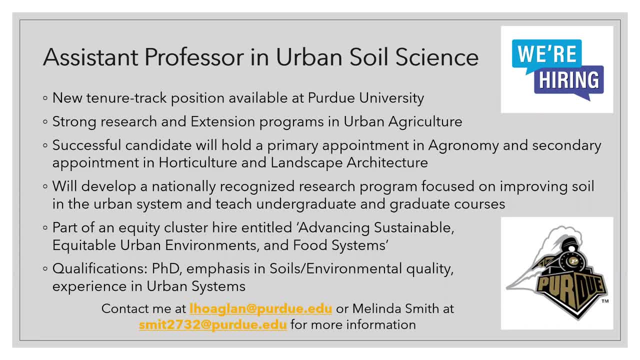 environment. So in some cases they don't survive well, and so we think, potentially, that this leaf mold compost was providing more substrates and habitat to keep that inoculant surviving for a little bit longer. Some other things that you know we've tried. I've collaborated with Dan Eagle. he's 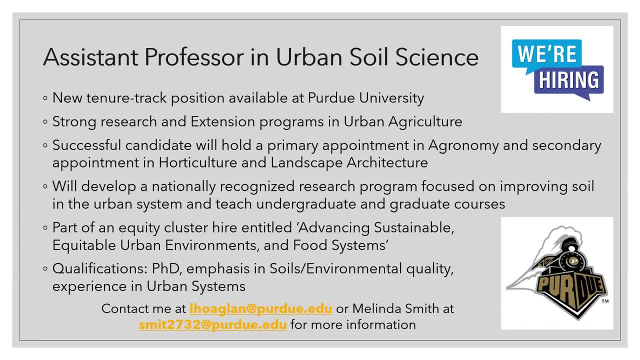 our plant vegetable plant pathologist here and we did do a study looking more at foliar sprays of different plants and we found that they were not as good as the leaf mold compost and so we did a study looking at foliar sprays of different microbial inoculants, both here in 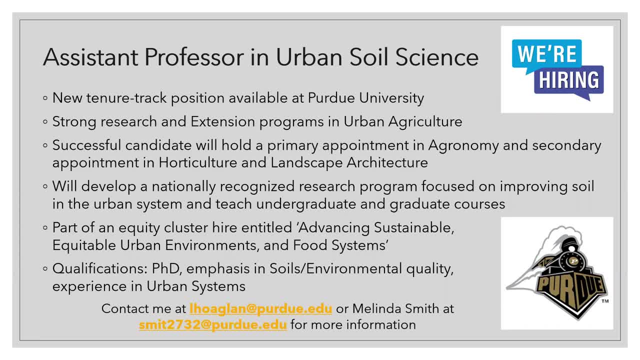 southern Indiana and North Carolina with Janine Davis's program, and so we tried some compost teas and you know different amendments that varied on both, like silicon, looking at different ways, and so in that case in that study I recall there was a gliocladium product that actually 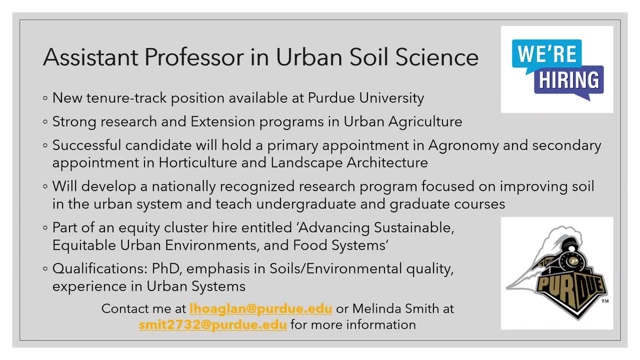 worked fairly well in both years, in both locations, to reduce the spread of foliar diseases, and so Dan Eagle would be the person to talk to more about that, and so, yeah, I guess I know there's a lot of work that's being done to increase the efficacy of these inoculants. 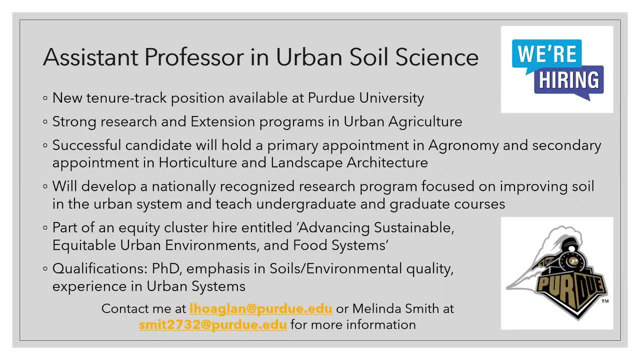 Last thing I'll say is we have experimented a little bit with mycorrhizal inoculants, and so we've actually found, though, that the native AMF tend to be more, you know, beneficial for the plant than some of the inoculants, and so, yeah, 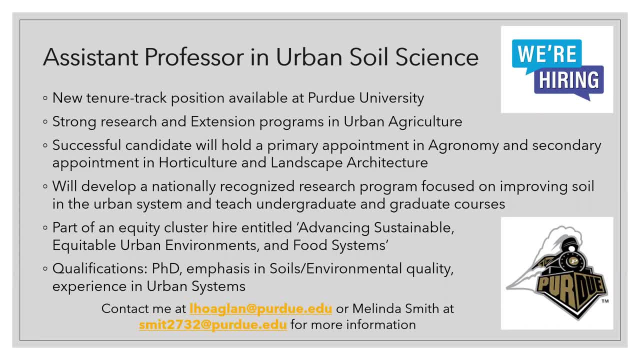 Okay, We have a couple more leaf questions here. One of them is: did Kyle use a variety of leaves or did he use specific types of leaves? Oh, that's a great question. So I remember we got that in the reviewing for this paper as well, and so, unfortunately, no, we used 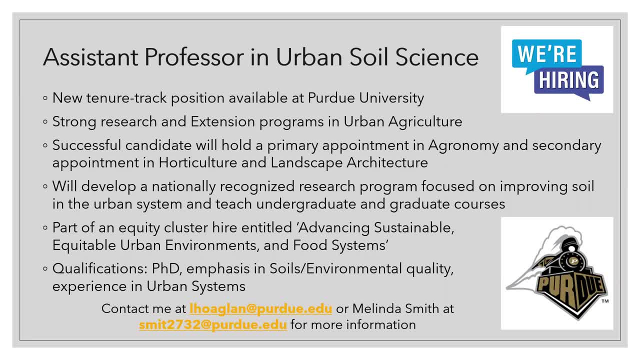 so it was actually a local farmer here, Dan Perkins, who produced that leaf mold compost and he just got all the leaves from the city of DeMott, Indiana, and so it was a mix of, you know, here we have mostly hardwood species, so a lot of sycamore, a lot of oak maple. 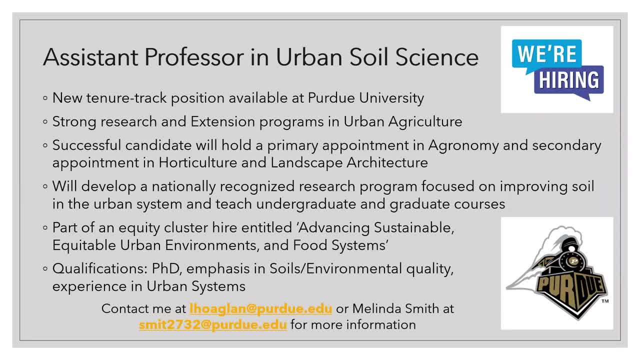 trees like that. that went into that. but I think, moving forward, we would love to do a study, you know, looking at different leaves and because we know that that's going to influence the properties of the compost. but yeah, 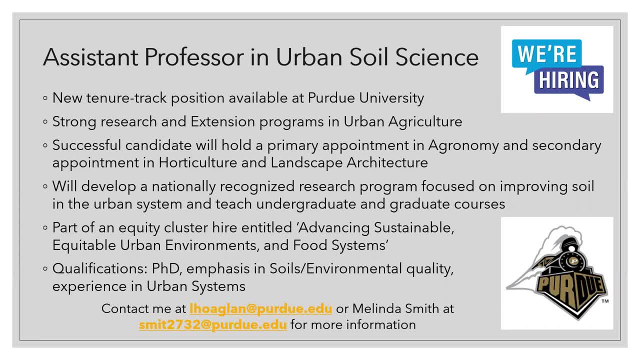 in this study- it was a mix, Okay- and also in using leaf mold from urban areas. are there concerns about toxins like petrochemical residues and are there any studies that look at that? Yeah, so that was another thing. yeah, that we discussed that in our paper and we were 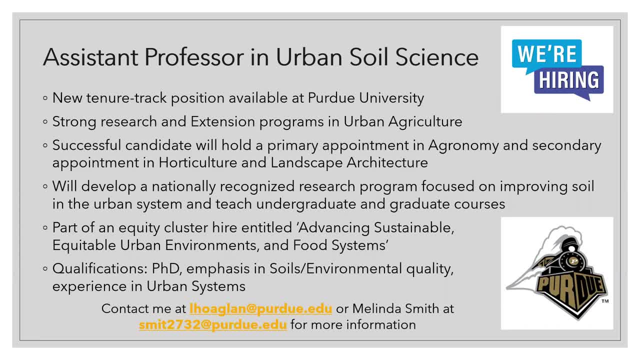 concerned about that and so, yeah, I think that's a good question. So in this case we did. we had the compost tested for different contaminants, both organic and heavy metals, because you know there have been some reports worldwide. I think there's one. 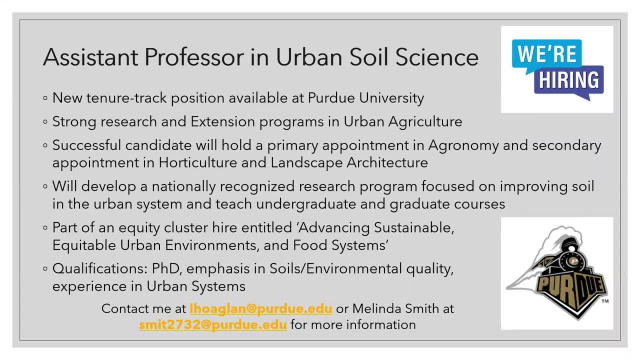 out of Poland, where they found some potential contamination in some of those urban forest wastes. In our case, though, we did not find any appreciable levels of contamination, and so, yeah, I think that's a good question. So, yeah, I think that's a good question. So, 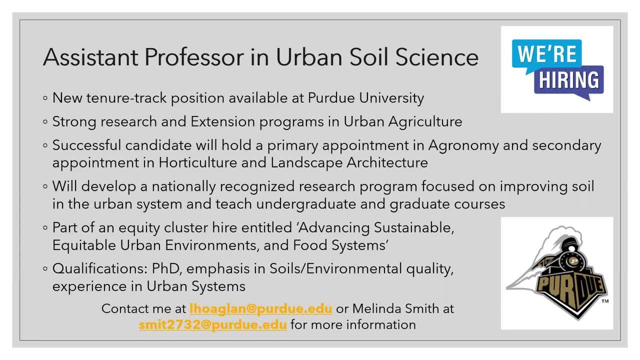 it was safe. Okay, yeah. and then John here commented that they use a large volume of used coffee grounds to enhance a high clay content soil. probably drink a lot of coffee, and is there a liability regarding heavy metals in used coffee ground? 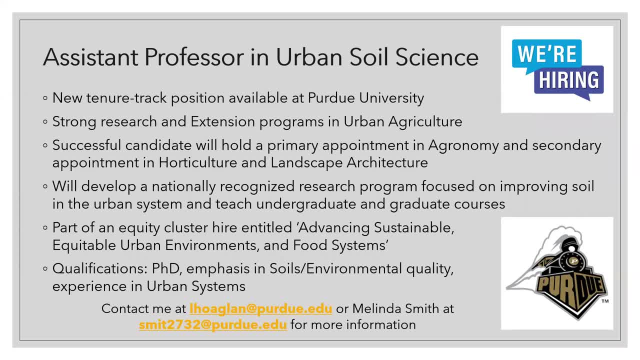 Oh, okay, so that's you know, I haven't done a lot of work with coffee, but I've read that coffee grounds can be a really good source of contaminants, and so, yeah, I think that's a good question. 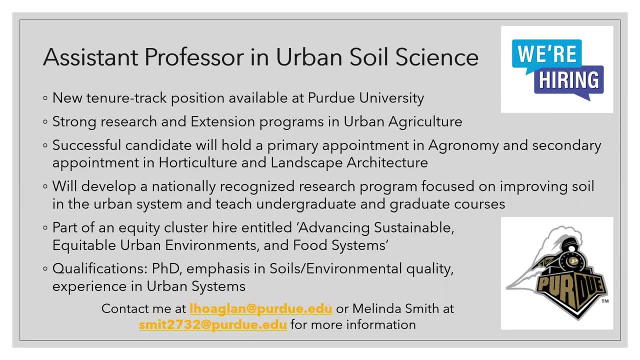 Great soil amendment, and so I think that there's definitely value in using those. In terms of coffee grounds being a heavy metal liability, I can't say for sure because I haven't looked into that, but my guess would be no, because I know I do work in South America where they grow a lot. 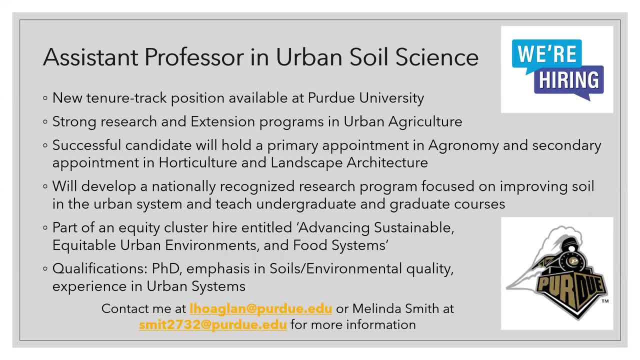 of coffee and cacao and chocolate. cacao does take up heavy metals, So that is a concern there, but coffee does not, and so I know, at least in the beans. I don't again I can't say for sure, but I wouldn't expect that to be a problem. 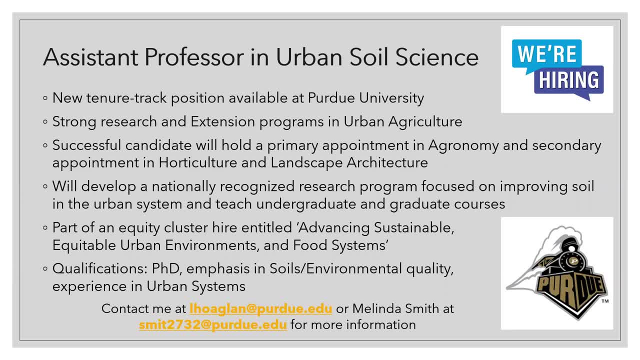 and so I wouldn't think the roasting and yeah, so I think it should be safe. but again, don't quote me on that For sure. yeah, you're not going to be held liable, No, don't. Okay, so we have a question from Courtney here, who's hearing that compost and 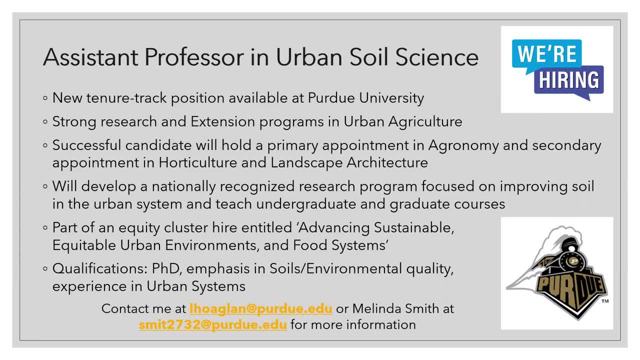 amendments suppress diseases, but they're still unclear how it helps with suppressing pests. Okay, yeah, so the question around compost suppressing pests or, you know, diseases, and I'm guessing the question is more around insect pests- is that correct? versus pathogens? 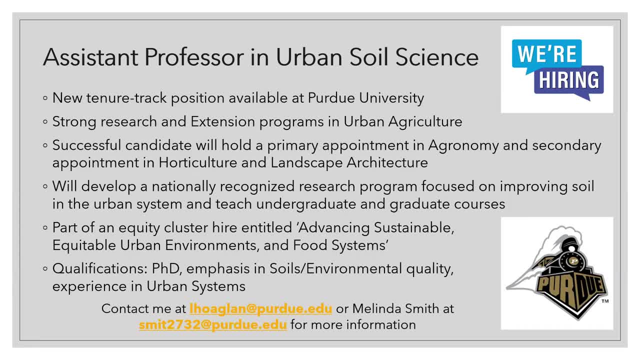 Let's see, Courtney, I didn't specify there, but pests in general. Okay, yeah, so pests in general. you know, again, that's my lab- we tend to focus more on pathogens that cause disease, but there is evidence also that 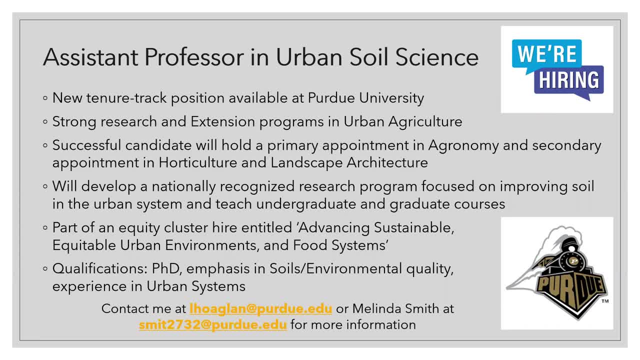 there are relationships between soil health and a plant's susceptibility to insect pests as well, and so there are some folks here like Ian Kaplan's group, I think, has done a little bit of work in that, and Laura Ingwell and one of her students, Katie, has started to do a little. 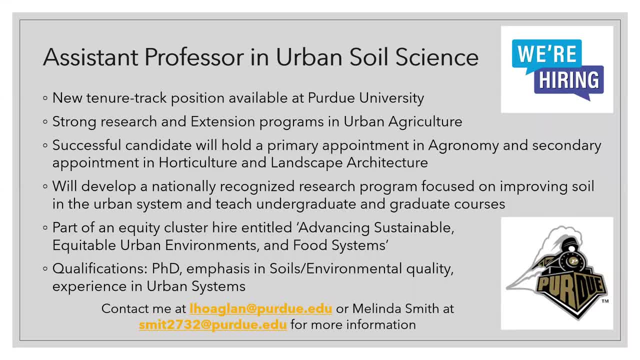 bit of work with that, with this black soldier fly compost, which is really cool, Okay, so I think that's a good question, I think that's a good question. I think that's a good question, And so you know, we haven't looked at it specifically, except in our field trial. 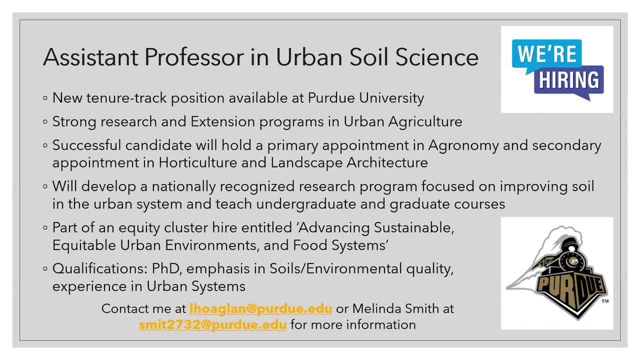 we did see differences in this little white fly that caused some damage in the squash systems, and so, similarly, just how induced systemic resistance can suppress or build a plant's immune system to make it more resilient against foliar pathogens. there is evidence also. 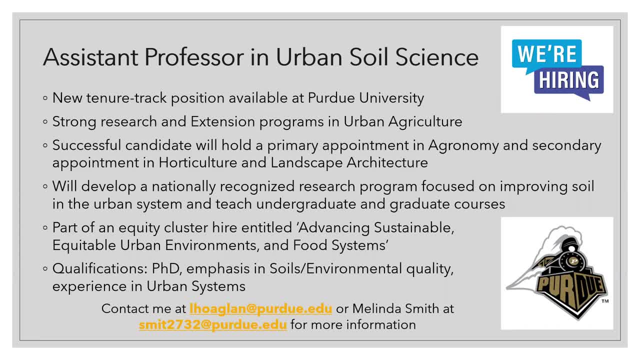 that that can help plants to resist insect pests as well. So again, I'm not the expert in that, but yeah, there are connections there, Okay. and then Lucy sent the link here, just at the end of the chat. you can see. let's see, she said thanks for the great presentation and here's a link to a. 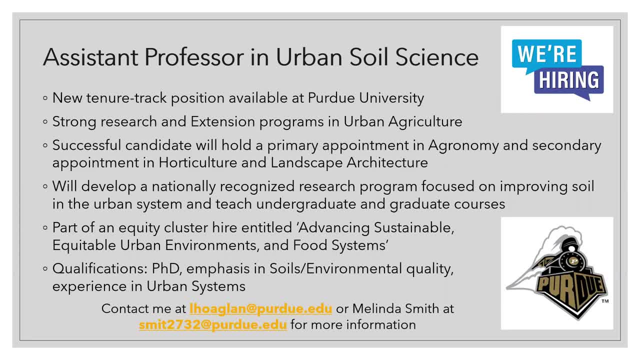 survey resoil contaminants for community gardeners and backyard gardeners that she worked with at Duke University. Okay, so if anybody wants to take that, you can click on that link there. Oh, and then Francine asked before: why is some compost sterilized? Oh, okay, so the question: yeah, why is compost? 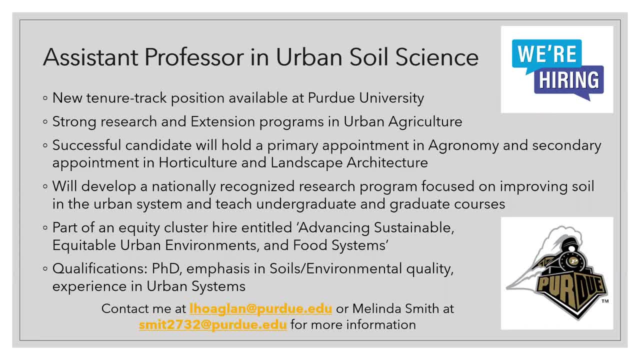 sterilized And most people don't do that. So we are doing that more for research purposes. So you know, we're trying to figure out what makes a compost suppressive and not suppressive. and so some things like a compost, some providing some nutrients, you know, making soil more friable. 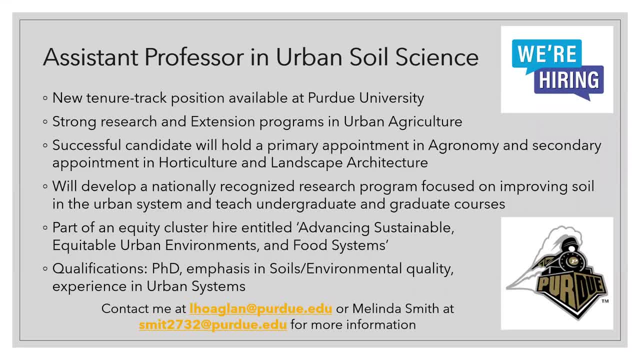 that could contribute some parts of pest suppressiveness. but there's also that microbial part that we're trying to understand, And so we, in our experiments, sterilize the compost, just so we can see how much of the effect is really due to the microbes within the compost. And so we 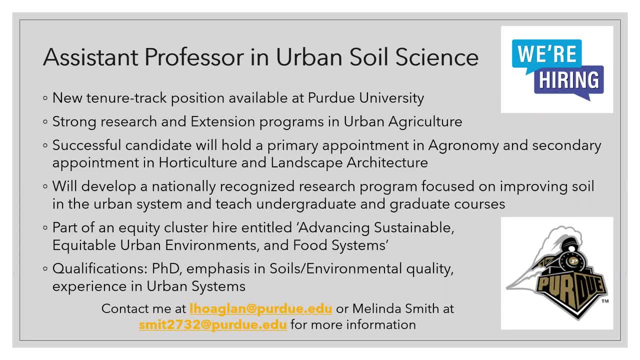 see in most of our studies very strong relationships between the microbes in the compost and suppressiveness. So again, we need to do a lot more work to tease that out. but that's why we're doing this. So I would never recommend anybody. 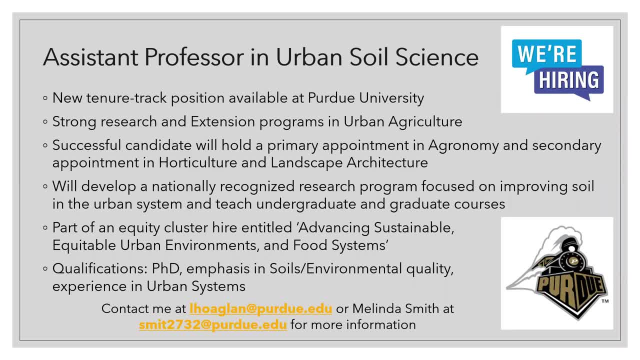 sterilize your compost unless, like it, you know, has some pathogen in it. but then I would probably say, compost it more because it's just not ready. Well, there are some sterile mixes sold as, for example, like for seed starting and that kind of thing. That's true, yeah, Okay, great, Let's see a couple more questions. 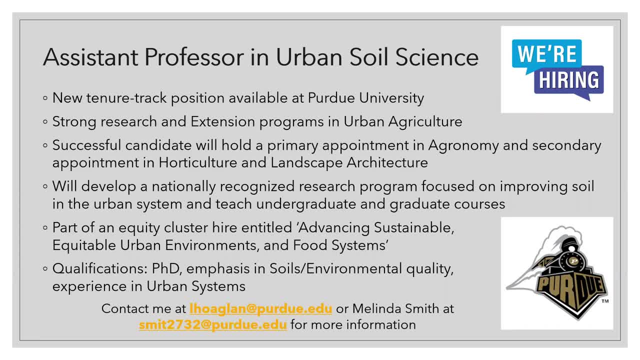 Collision of phosphorus. are there methods or studies that are being implemented showing alternative methods or resources of phosphorus? I haven't. I have read about mycorrhizae but haven't heard of anything else. Yeah, oh, that's a great issue to bring up in that. 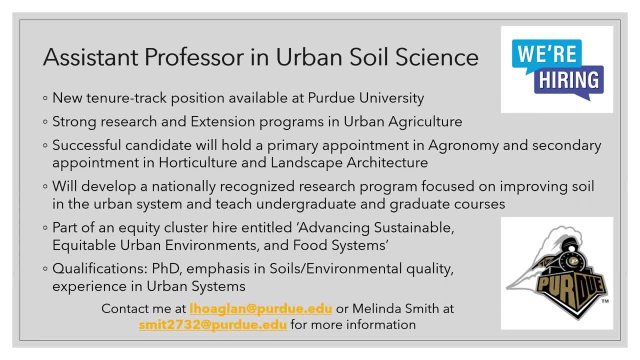 yeah, the world's phosphorus supplies are going down, you know, and that's going to be a problem in the future, And so I know there are some efforts here, like I've heard about. I know there's some people that you know they're doing a lot of work on. you know the. you know the. 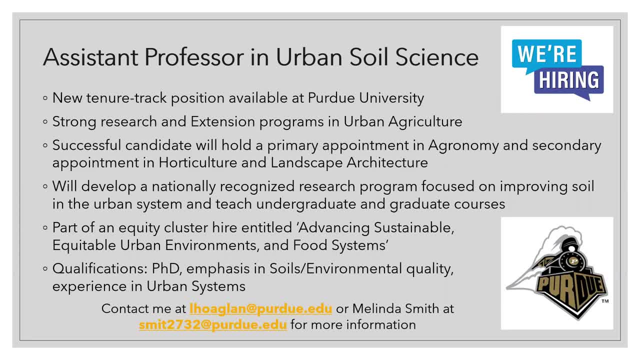 work on these drainage ditches along agricultural fields and are putting in buffers and using biochar actually to try to bind some of the phosphorus that's not being taken up by plants that's getting into waterways as one way to help kind of recycle some of that phosphorus. There's a lot of. 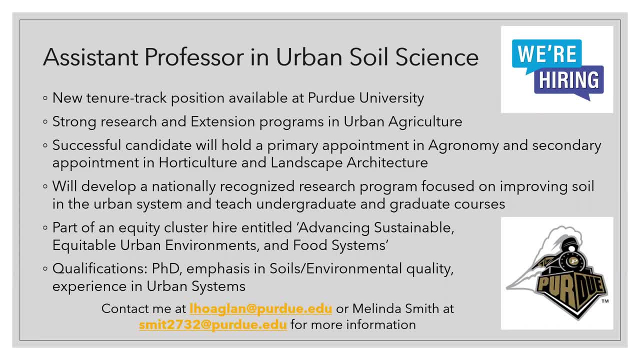 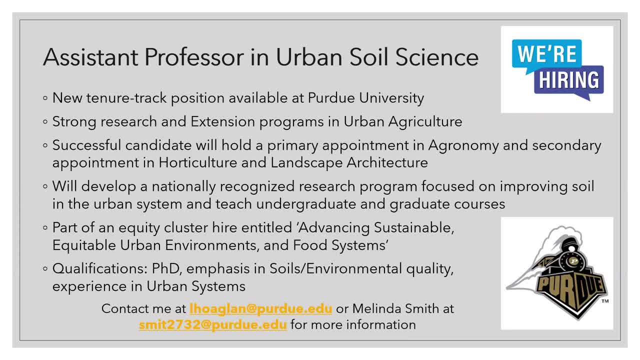 to be collected. So those are two that come to mind, But the point around mycorrhizas is important as well, because a lot of soils will have a lot of phosphorus in it, but phosphorus can be bound very tightly so the plant can't get it, And that's where mycorrhizae can be very valuable. 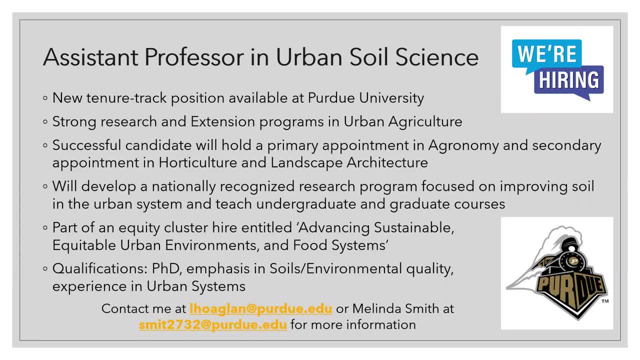 because they have the capability to increase solubilization of phosphorus to make it available for plants, And there are also some bacteria that have that capability as well, And so there are a lot of people working on microbial inoculants, also around microbes that enhance phosphorus solubility and availability. 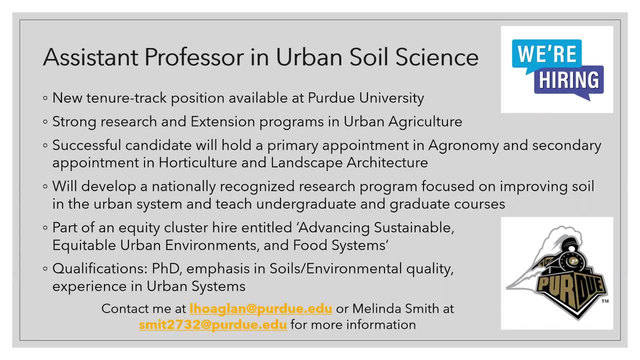 to plants. Okay, We have a question here from Antonio, who is wondering: how did native AMF populations differ across urban soils in Indiana And were any specific AMFs more prevalent across sites, And maybe you could tell us again what AMFs are? 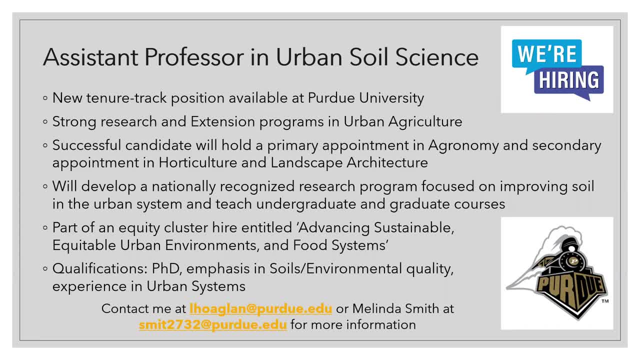 Yeah, So the question is about AMF, which are arbuscular mycorrhizal fungi, And so that just describes a group of fungi that form a symbiotic relationship with plants. So these are plants within the glomera or fungi within the glomera mycota, And so they get inside. 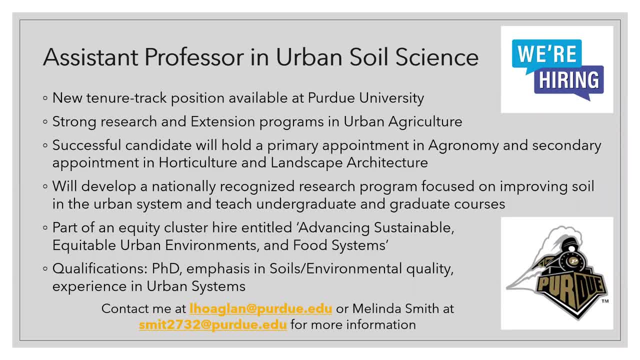 plant roots, They form these little arbuscules that are sites of exchange between the plant and the soil, And they send out fungal hyphae into the soil, where they can solubilize these nutrients and then move them into the plant, And so we don't have yet the results of how they varied. 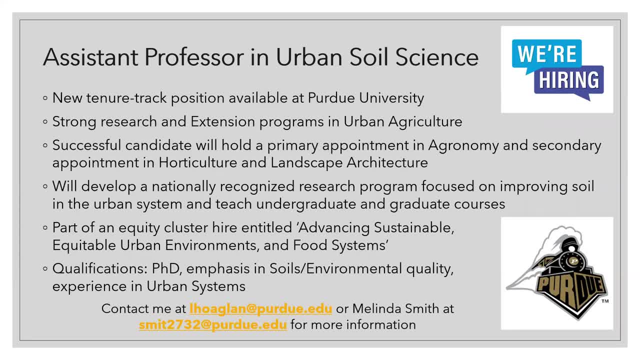 across our urban ag system. But when we did studies at our research farm, MIGS, we found we were just comparing organic and conventional systems And we found a lot more diversity within the AMF and the organically managed system. And I'd have 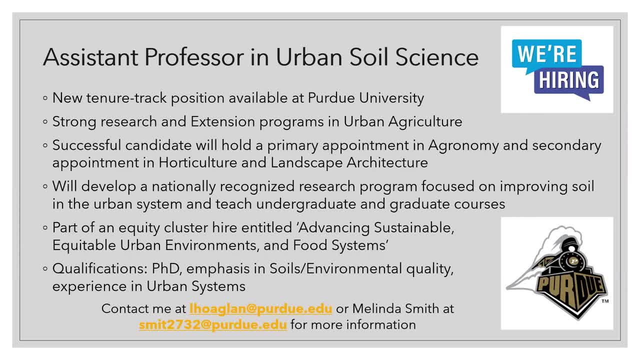 to go back and look at all the different ones. I know chloroidoglomus was one of the most prevalent that we saw in both soils, And so that is not one that's typically in a lot of inoculants. You usually see things like Rhizophagous irregularis, And so some of these other. 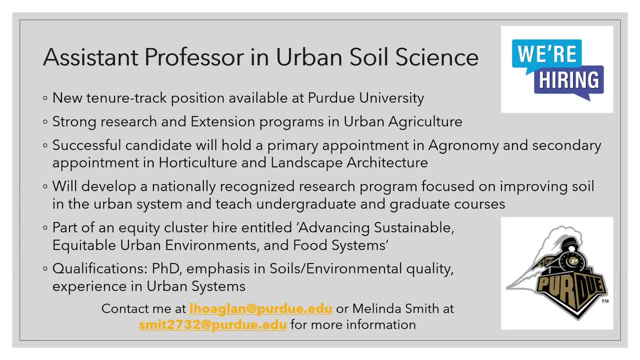 AMFs that we found were more prevalent in both soils And so that is not one that's typically inoculant. And so the AMF again I'd have to look at specific ones. Send me an email I can let you know. But different AMF have different scavenging strategies in soil They have. 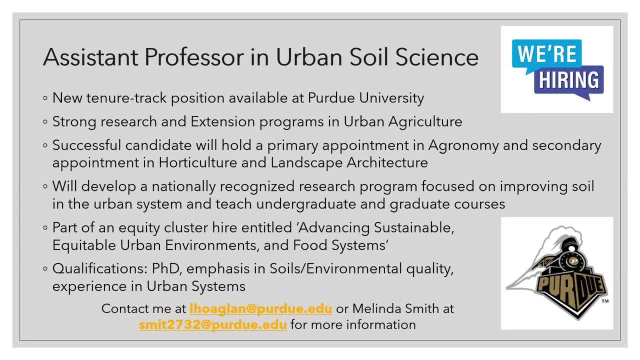 different amounts that they take from plants, And so we think, at least you know, having that diversity in some of these native ones are better. Okay, Yeah, That sounds like a good question for you to contact Lori about, because there's a lot to that here, So let me just go. 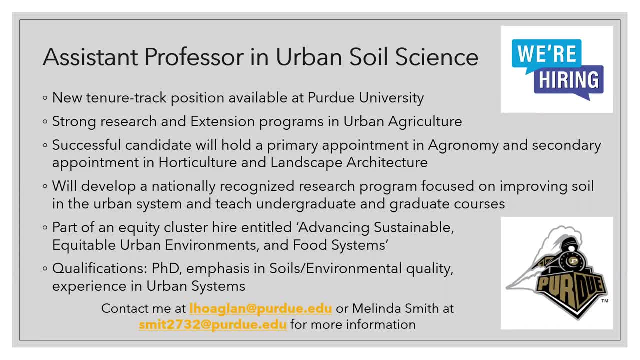 down and make sure, okay, yeah, there's a couple more questions. are there any? are there additional beneficial studies on growing mushrooms with crops, wine caps, etc. oh gosh, okay, yeah, that's a really interesting question and i, um, so, yeah, and i, i saw somebody at the tri-societies last year. 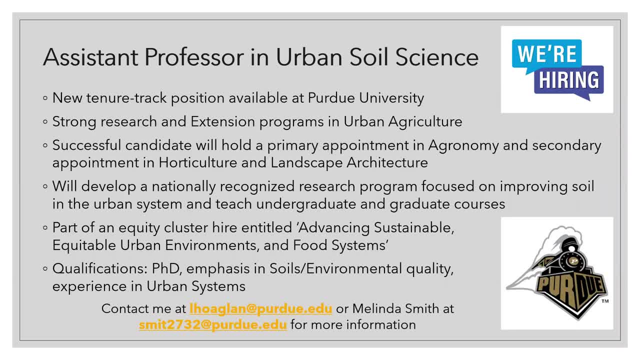 speak about that and i i don't remember all the details. i wish you did um and i don't believe that they saw much of a benefit in this, in that study, from kind of like intercropping mushrooms in the crop, and i wish i could remember what they might be able to look it up by looking up the soil. 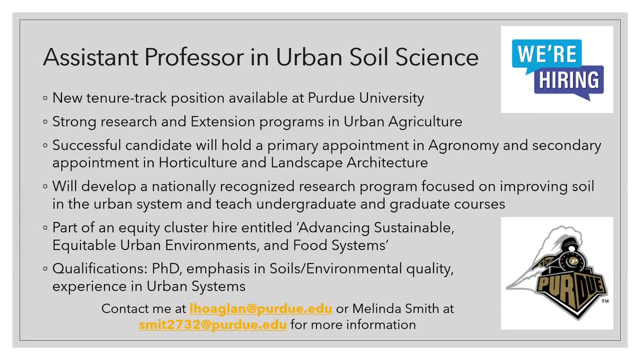 science society's conference from 2021? yeah, searching the abstracts there? um, yeah, because that might lead you to the researcher who's working on it. yeah, sorry, that's a great question. i wish i had more information. you may be able to track that down. okay, i think we've got the last question here. um, thank you for sharing your group's research. 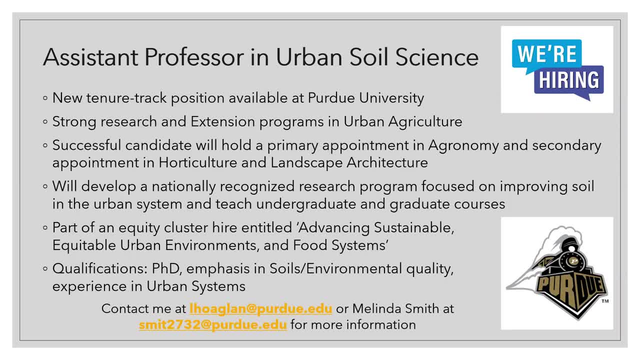 and for organizing the series um. does your research intersect with other active research in urban soil health, including soils contaminated with heavy metals and soil animals like and and and vertebrates, both beneficial and pest? Oh, okay, So great question. I mean, yeah, we're. 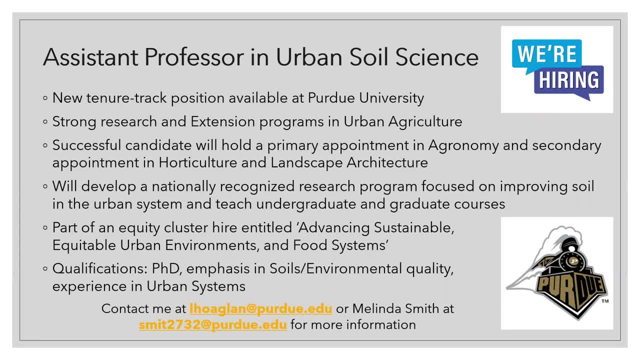 we're constantly, you know, working with different people and different aspects of it. You know I haven't worked so much with the vertebrate pests and things like that, but Laura Ingwell here at Purdue, I know who's doing some interesting work in that area: Doug Richmond.